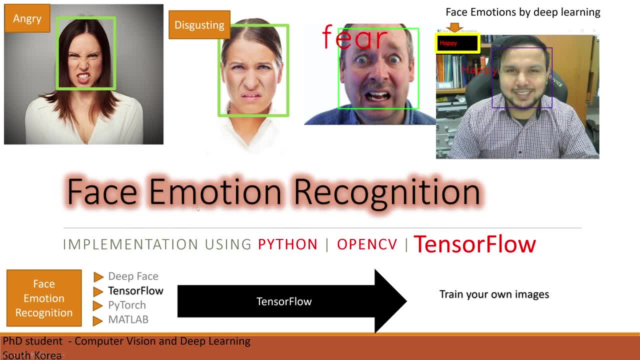 I would like to inform you that for the same topic, such as face emotion recognition, we do have four different videos with entirely different methodologies to follow. My name is Shah Rola and I'm a PhD student at Inha University, South Korea. My major is computer vision and deep learning. 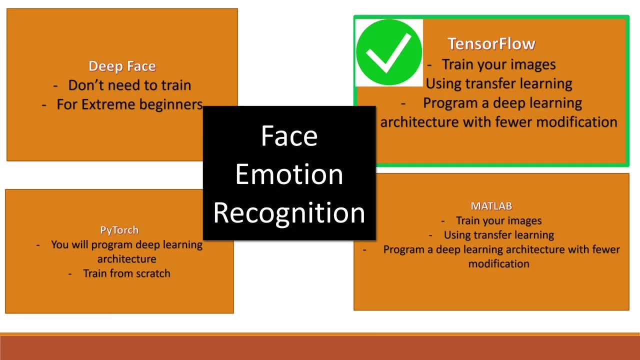 Let's get started. Before diving into implementation, I would like to inform you the scope of each video. If you are at the beginner level and you hesitate to train a deep learning architecture from scratch, deep face is the best suitable for you, because you don't need to train anything and a lot of 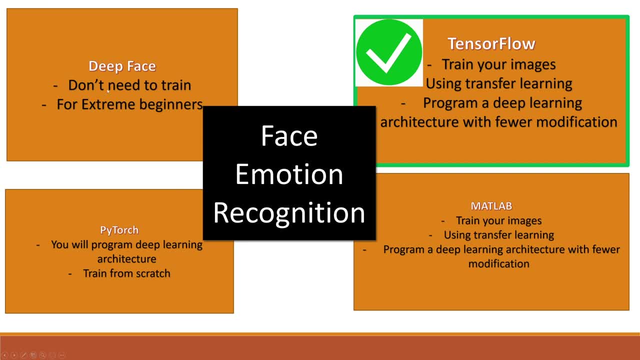 deep learning architectures for face emotion recognitions are already available in deep face. On the other hand, if you are a deep learning enthusiast and any of the programming language or library- sorry, these two are based on python, like the tensorflow. if you want to follow tensorflow, pytorch, you can follow any of them Similarly. 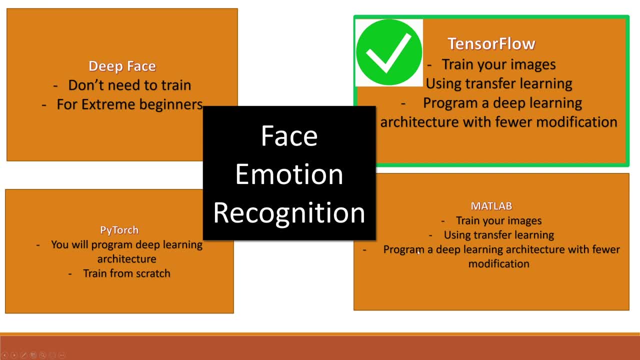 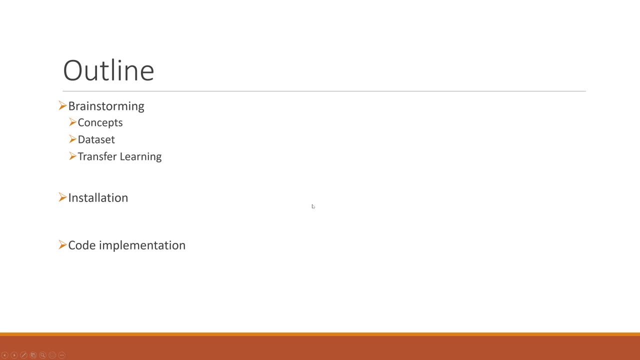 if you are interested in matlab, you we do have matlab based implementation as well. One extra information I would like to give you is that the input and the output is same for all these four videos, while the methodology is entirely different. This is the outline of my today's video, such as in the start, I will explain the concepts. 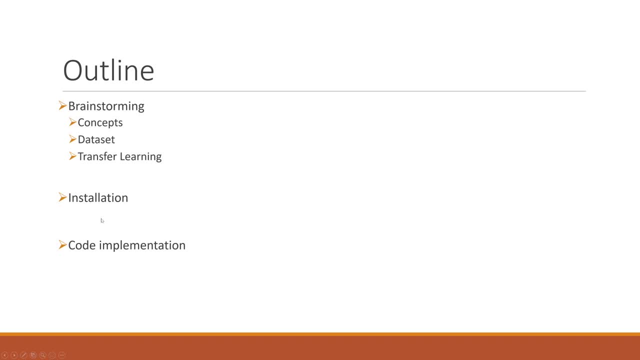 the data set and concept about the transfer learning, then installations and at the end we will be diving in for the code implementation. As I said, that the concept for all these four videos are same and if you know already know the concept and if you already know the installations. 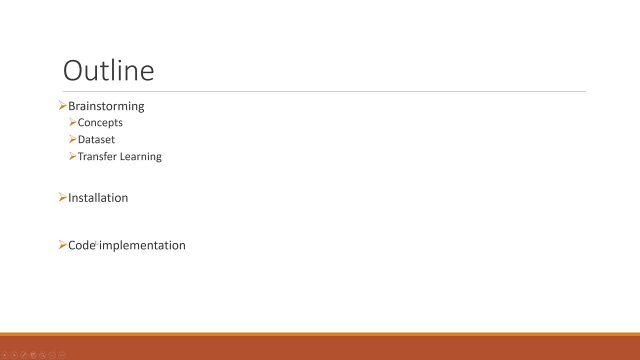 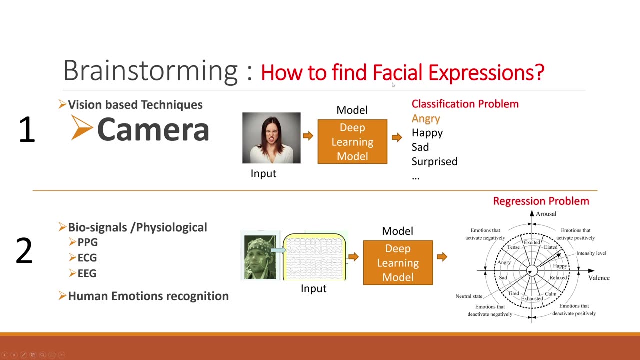 of the anaconda and jupyter notebook. you can just directly dive or navigate for the code implementations. Broadly speaking, facial expressions recognition can be divided into two different techniques, although we can have different other techniques as well, but broadly we can divide into two. One of them is camera based techniques, like we call it, vision based techniques In this scenario. 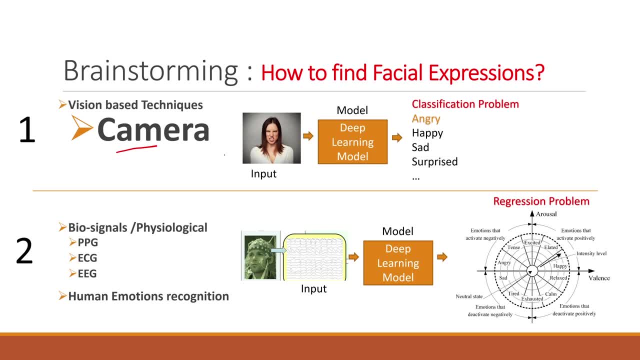 we will be taking a main, an image of a girl, of or any human body, and then we will detect the face and then, based on facial features, we will train the facial features. We will train our deep learning architecture for different classes, such as angry, happy, sad. 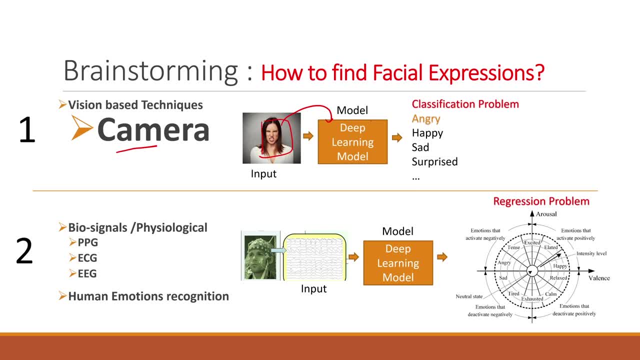 surprise and, correspondingly, in this particular scenario, as you can see that this girl is angry, so we can classify our deep learning architecture can classify this face as a angry face. on the other hand, although we can classify this as a angry girl, but this can also be fake up. 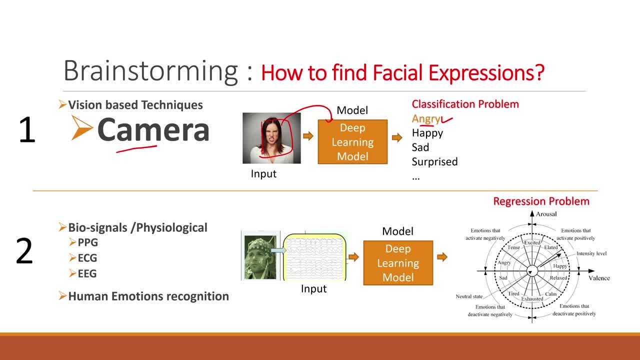 For example, if new cat on a ocean, anyone, anyone, can be MAYOR. basically, this channel has more dingen that afraid the cat. as in the beginning, i show you some video in which i was just faking up my faces for happy and all of a sudden i was surprised, all of a sudden i was angry, so i was just 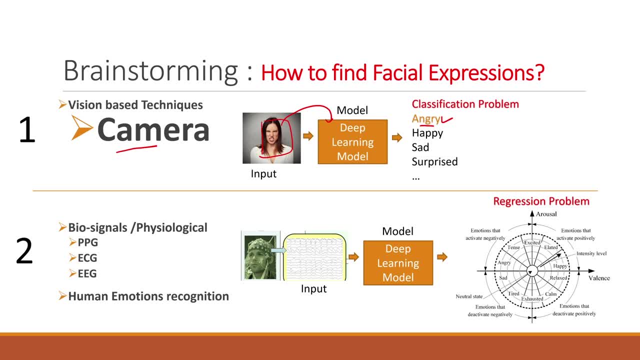 faking up my facial expressions, but actually i was not angry at all, or always not surprised at all. so in order to detect either in real uh she's angry or not, we have to connect some biosignal for real world problem right for real. we can definitely do it in this case. no one can pick. 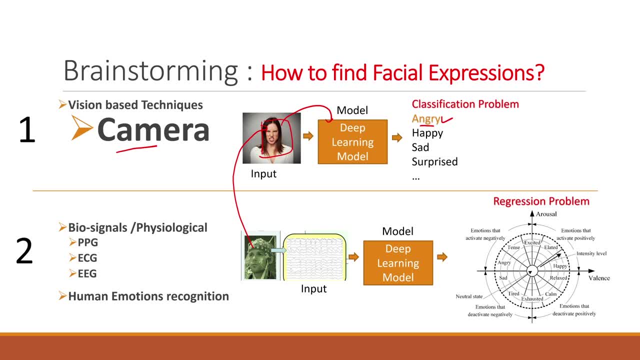 up right, because it's based on your body sensors. one another difference is a difference is that we do know that she's angry, but we do not know the level or intensity of being angry, how much she's angry. in this case, biosignals are the best solutions. for example, biosignal can 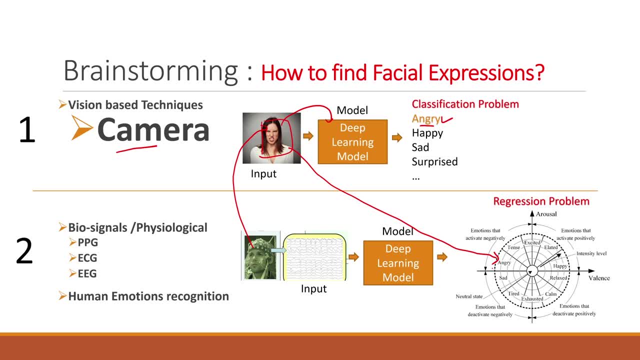 further classify or can further tell us that how much she's angry? in the classification problem we always say that, for example, she's angry and we said one. okay, the output of the deep learning is one, so we say angry. if it is two, we say happy. if it is three, we say sad and so on. in case of the, 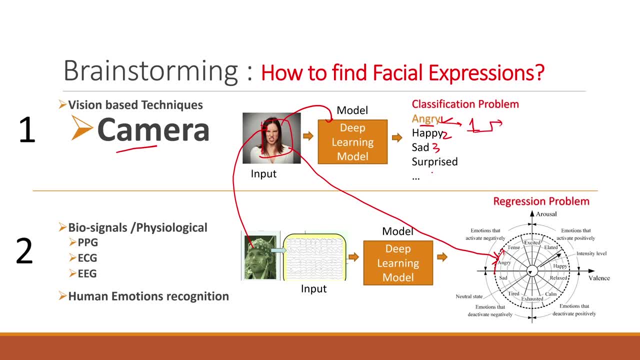 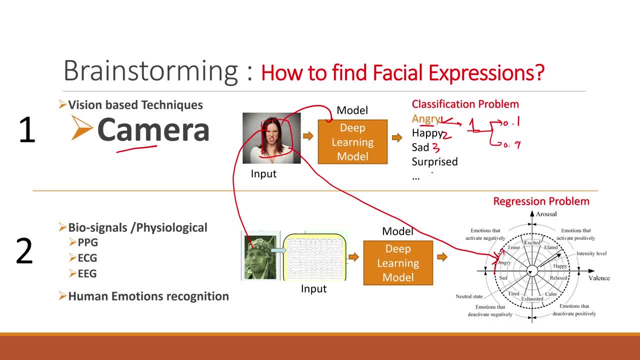 we want to know the intensity of the angriness. this is called as a regression problem. so regression, the output of the regression, is always a floating point, while the output of the classification problem is in the decimal point. so one we can further classify one into 0.1, into up to 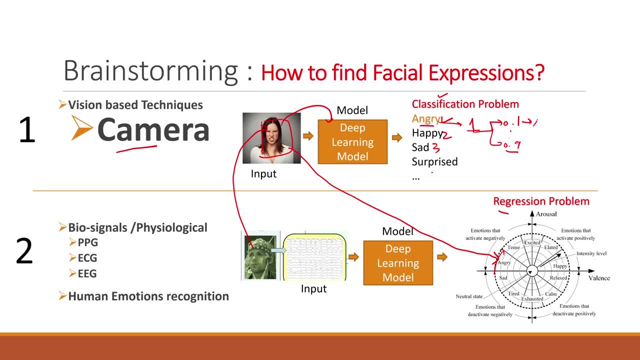 0.9- right. so 0.1 shows that she's low level angry, or the level of angriness is low, and 0.9 or 1 is very high, right. so the output of the regression is floating point and the output of the classification is one. 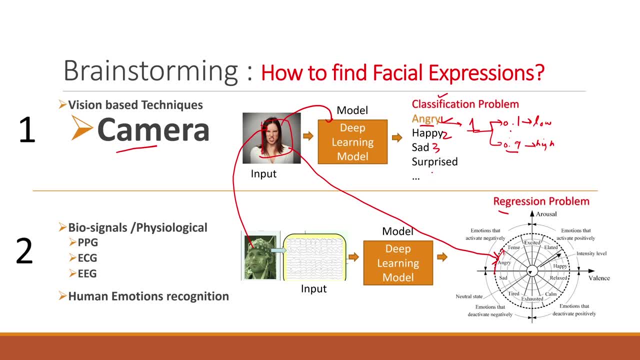 so, using biosignals, we can resolve the regression problem. so other things is, for example, this was, as i told you, that this is eeg based, like brain signals. similarly, the source could be cardio, like heart or, for example, respiratory system as well, so there could be many other sources of the body. 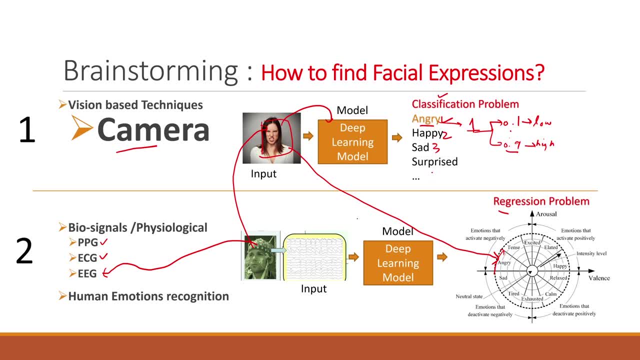 which can tell you that either a person is, which kind of emotions are there? so in the case of biosignals, we call it human emotions recognition, rather saying it facial expression recognition. so in this case, for example, this is 32 channel, a typical eeg signal or sensor, and then we can just 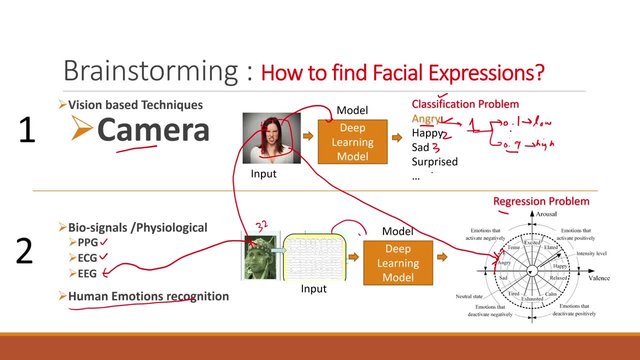 get signals like this and then we can train our deep learning model and then we can further classify into angry, tense, excited and a lot of other categories we do have. now that we have established that our problem is classification problem and our input would be vision based, our, if you, in case you're interested. 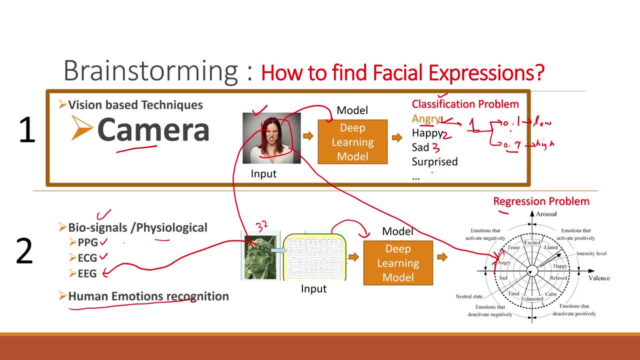 in the physiological signals, also known as biosignals. if you you're interested, we could also make a lot of videos. do let us, let us know in the comments, right, about this video, if you like it. so our topic, today's topic, is this one. right now that we have established that our problem is, 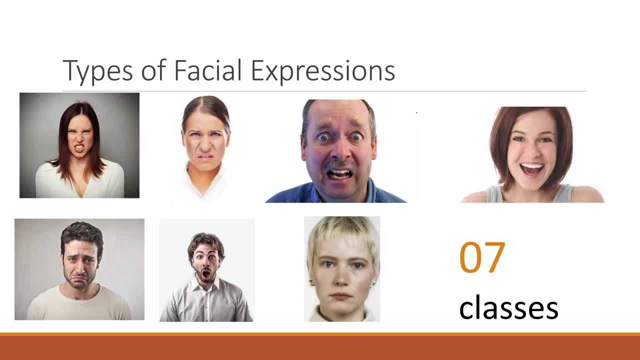 classification problem. right, so we could have many classes, as over here we say tense, excited, and a lot of them, but over here, in this particular video, we are just classifying, for simplicity, only seven classes, such as this girl is angry. this is: this girl is showing disgusting facial expression, right, something we say when we see something very 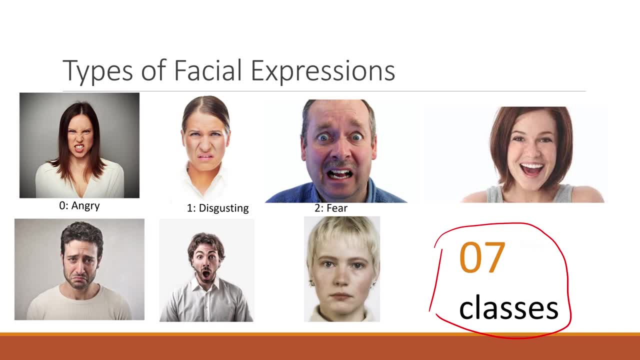 not appropriate. we say disgusting, right. so this is fair, this is happy, this is sad, guy is surprised, and in this case, this girl is totally neutral, right? we do not know what kind of expressions are there, so we classify it into neutral, okay, so there are a lot of different. 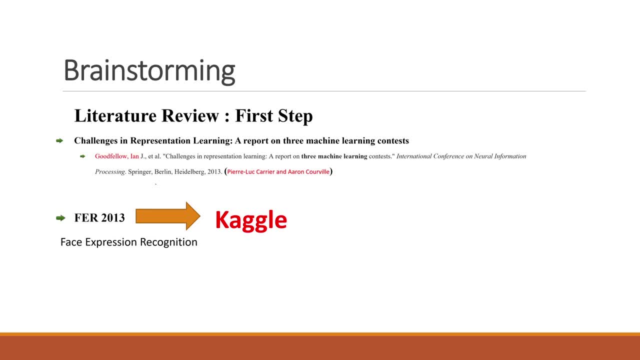 data sets available in the market, you can say in the research community, and the one we have selected for this video is fer 2013, and it's by google, actually, and aeon goodfellow is the author of that, which is also author of or pioneer of gans: generative adversarial neural networks. so 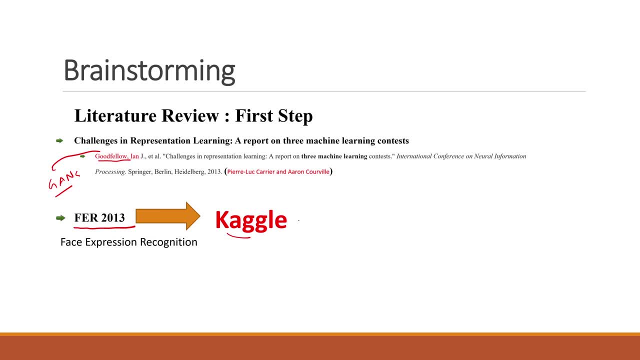 this is published in the kegel website. so those who do not know the kegel website, it's a famous website in the deep learning community, so whenever there is a problem occurred- okay, so a lot of companies are there in the world- they just post their problem in the on the kegel website and the 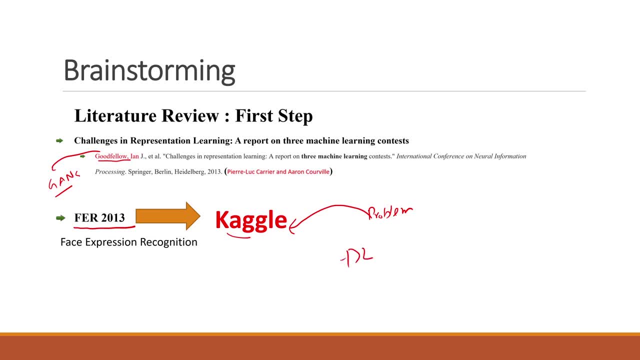 deep learning experts across the world. they just provide the solution like: this is dl1, this is dl2, and up to so on. and then what kegel does is that they hide some of the data from these deep learning experts. then they check the results or test, and then they announce the. 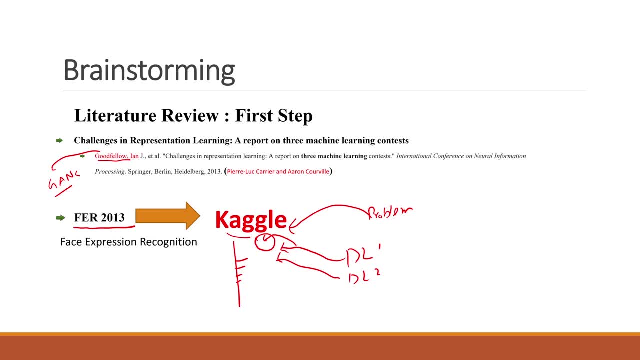 result: who is first, second or third, up to so on. right. so why i told you something about kegel? because those who just starting their career in the deep learning, i would recommend you to visit the kegel website because there are a lot of competitors and there are a lot of companies. 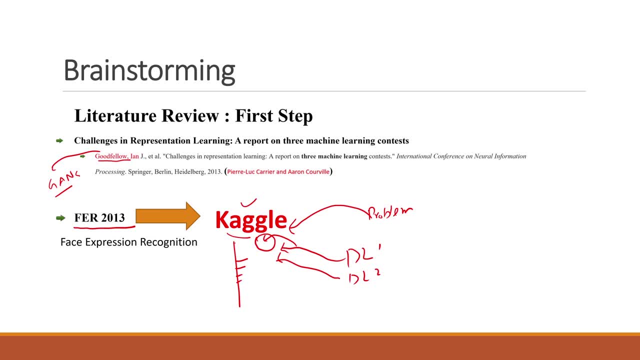 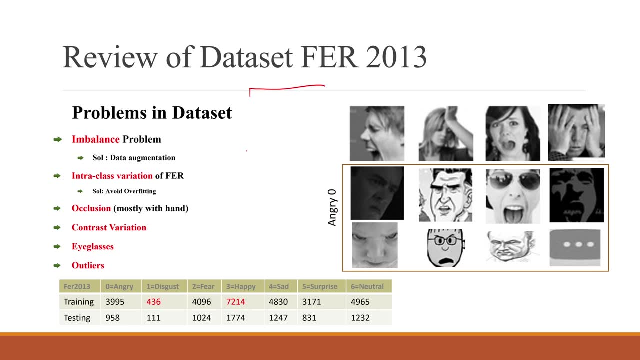 going on and, if you're interested, that would definitely boost up your skills correspondingly. okay, now that we have selected this data set fer 2013, one very important thing is that this data set must be a realistic one, right why, in this scenario, we have seen that this image is crystal. 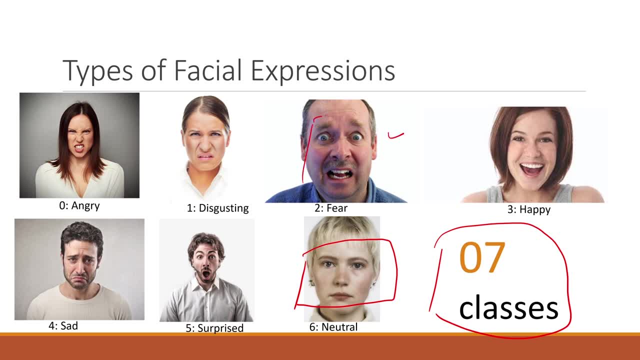 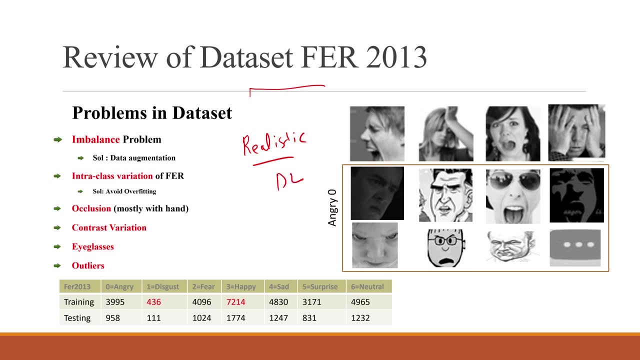 clear. the background is white, we can easily detect the face and the expressions are very clear. but in the case of this image there is no problem, definitely if we train our deep learning architecture on these faces, definitely when we show this face, although this guy is angry, right. 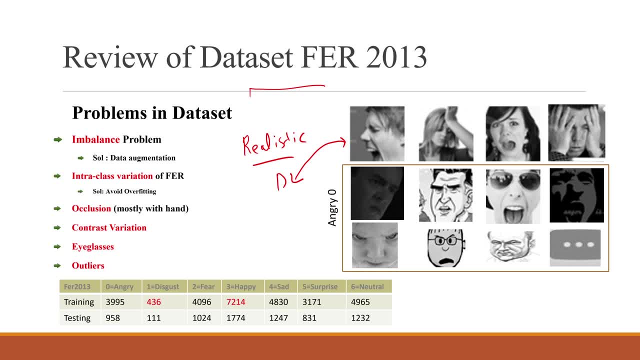 but it would fail. why? because this is one thing is sideways and definitely there is a lot of noise at the side. so a data set should always be a realistic one. so, as i told you before that it is by google. okay, so what google did is Base like from Google website. a lot of over the years, people were uploading their videos. 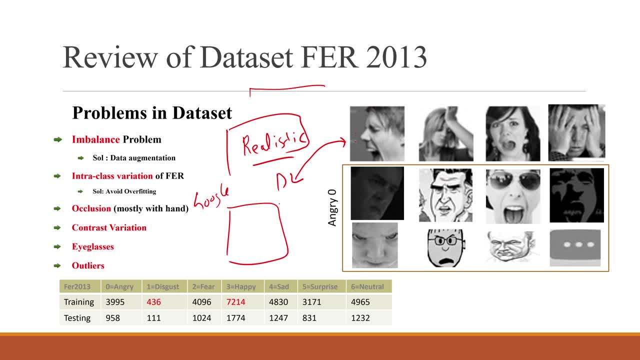 Right, and images like, just like in a Facebook and other things. We were uploading our videos. So what Google did is in order to make this fer 2013 data set, they just went to all the videos and They just or pictures and they just crop these faces, Okay, and then they labeled it. 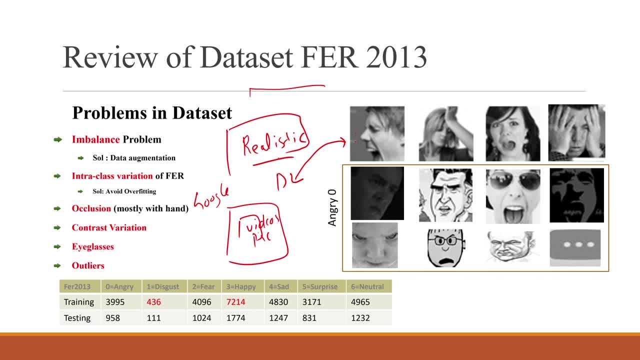 So now we have a realistic data set. So one problem: in the whole complete Google data set, they could only find only, for example, 436 samples of the disgust problem. Well, for the happy, they found a lot of them, right you? because you guys were uploading your images of the happy more. 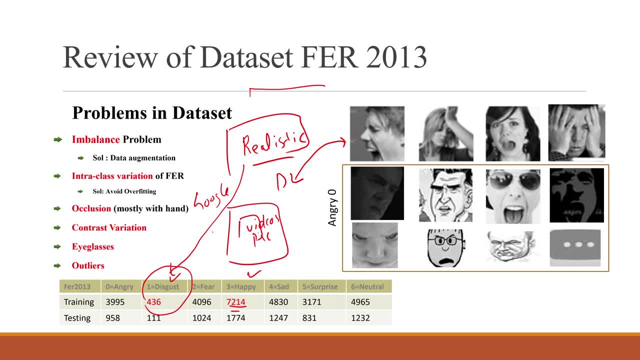 But the disgust very less, because in disgust sometimes you don't look good, right. so So ideally, the deep learning are architecture should have should get same number of the classes. why? because if that for the happy, the deep learning weights will be Biased towards happy. if any of them is more, then it will be biased towards it, right. 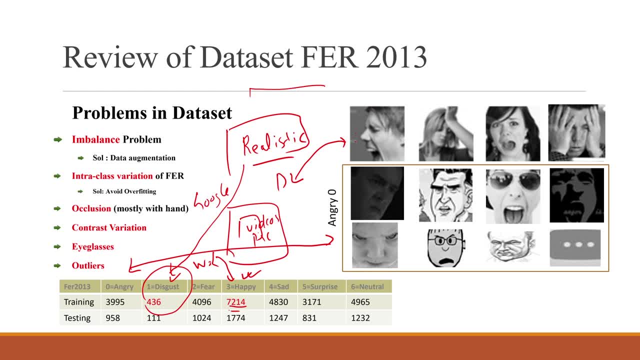 So it will try to infer everything regarding the happy. Okay, the solution should be that augmentation, like, one of the solution is increased. Augmentation mean increase, right augment mean increase. So one way to increase data set, like one way to make 436 equal to 7000, is that this is an image. Okay, I can rotate this image and 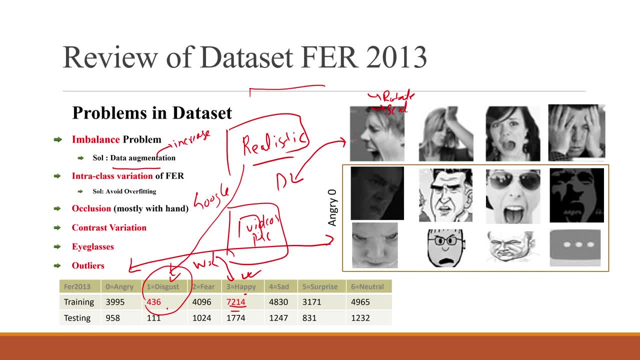 Create another one. Okay, then I can scale or zoom, zoom in, zoom out another image so I can create one, Then one, then up to so many techniques I can do, and then I can create from one To six or ten, or, for example, for every image. when I try to do it it will be more images. 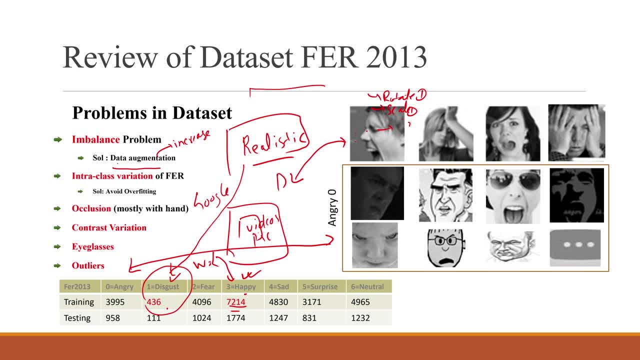 So one solution to resolve imbalance problem is data augmentation. Okay, What is second problem? second problem is: okay. I would like to inform you another thing: Gans, Gans is generative and very cell neural networks which can create more images. Have you seen a lot of? 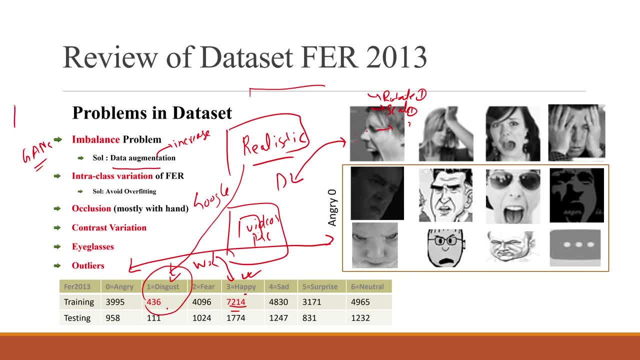 mobile applications who, for example, in the Facebook as well, for someone there is a kid and there is a, for example, Not a kid, sorry. for example, parent based based on parents. For example, this is a girl or this is this is a husband, For example, this is wife, and they can just tell you that what will be the face of your kid, right? 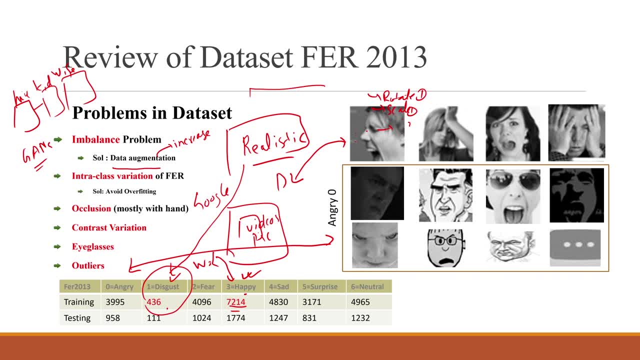 It can just tell you. so there is there, the technology is Gans. So Gans can, based on make, by mixing two facial features, It can generate new ones. So generative, adversely neural networks. Okay so, Okay. So that is again another technique of the data augmentation. 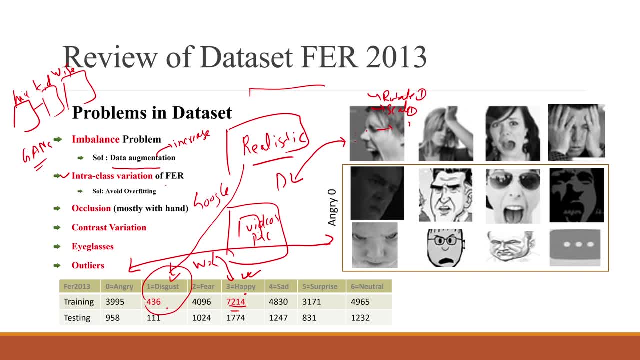 so Another problem is intraclass variation of the fer. so intraclass variation means that all of them belongs to same class. But you can see this is face image, but this is painting and this is cartoon. So these are entirely different. this is a sketch right. 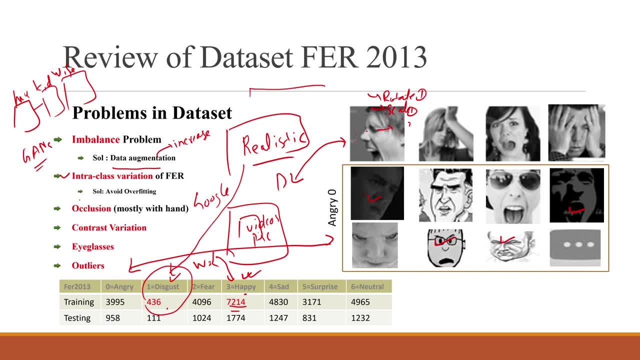 So all of them are entirely different in nature. So intraclass mean inside class. I have a lot of variation going on, So deep learning architecture must be Robust enough to tackle all of them right, Okay. another problem is occlusion. occlusion means that this guy is: 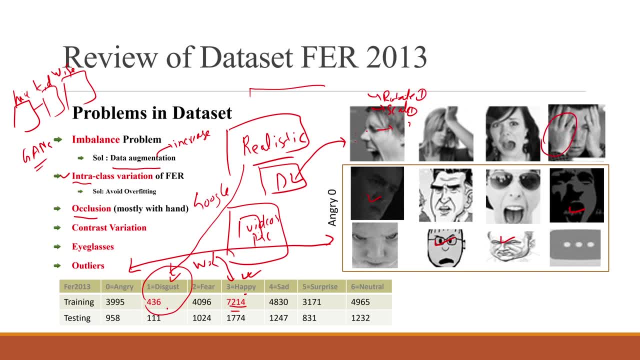 Co has covered his face with his hands, So it's very difficult for deep learning architecture. Why? because only this part has been left right. Similarly, we have contrast variation. This image is too black. Similarly, this image is too black, but this is white. Okay, so we have a contrast variation. 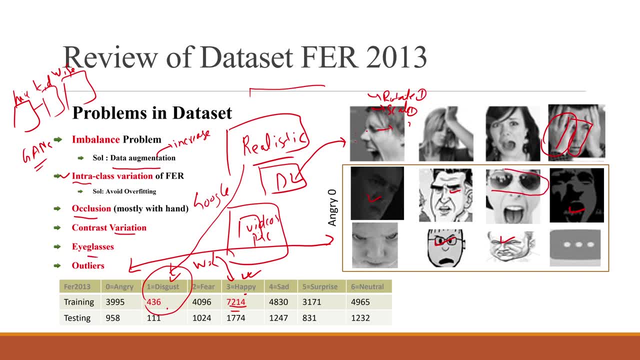 eyeglass problem. this girl has covered her face with the glasses and eyes and covering her eyes. So eyes are very important features. Why, by looking into eyes, we can easily detect that she is Definitely surprised. right eyes are very important features, So eyeglass problem similarly outlier. as I told you that these are just cropped images, 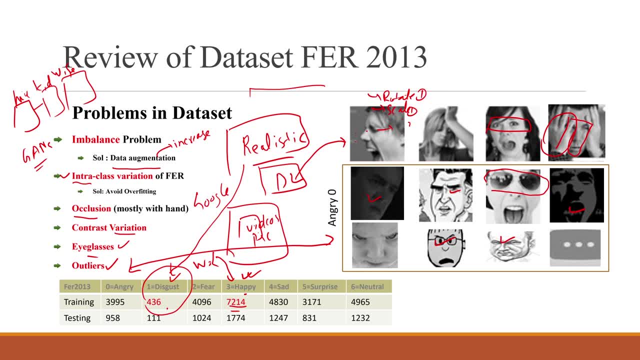 So definitely nothing is perfect in the world. So They have just mistakenly cropped some unknown images and just put it into angry. But definitely it's a good thing for deep learning, because it will. it must be robust enough. Not that we have studied data set. It means what we can infer, what can be. conclusion. 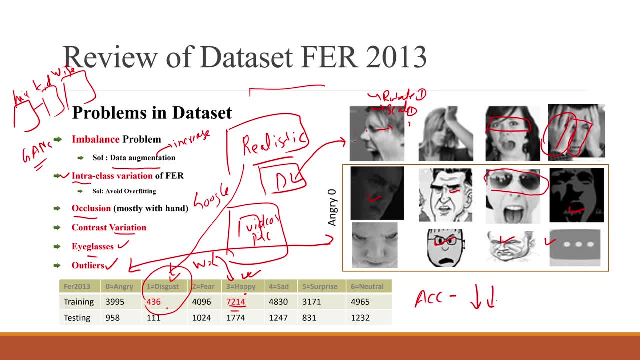 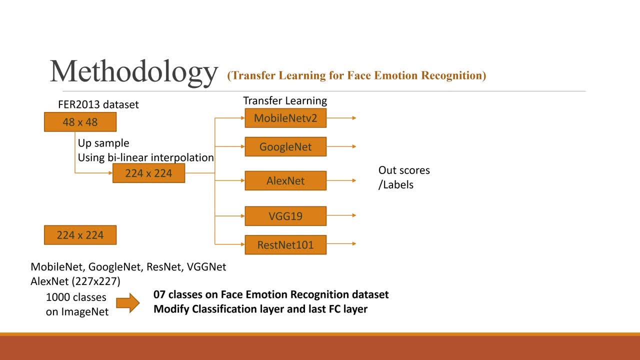 Accuracy will always be very down. Okay, Why? because these are not an easy data set, right? So, in order to get accuracy is very difficult, okay. What is the methodology? How we can achieve Face emotion recognition? okay, Let me tell you that. what is deep learning architecture? 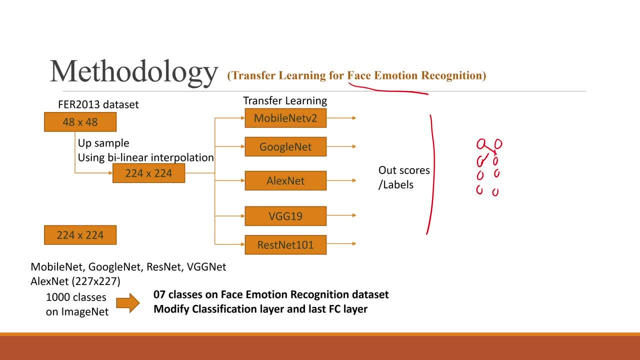 Like we have neurons, like these are the connections we have. Okay, so these connections are basically connected like one first layer and for the second layer, Every neurons are connected to second layer, right? So these are nothing but weights. as you know, we always save our. 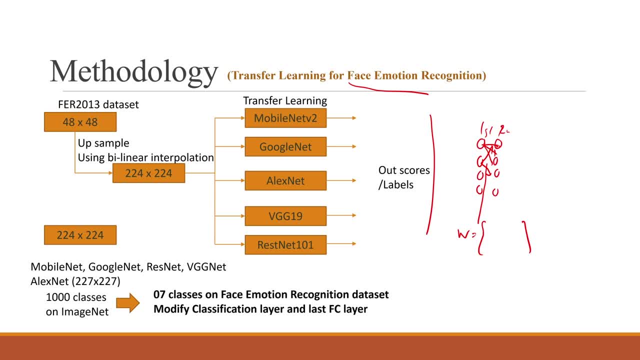 Models at the end, after training, into some weights, right? So these are weights and parameters. So basically, deep learning architecture is nothing but a set of weights. so if you have Noticed that, whenever we train our deep learning architecture, You always get some epochs and accuracy and slowly and gradually we get some good accuracy at the last time, first of all, 90%. 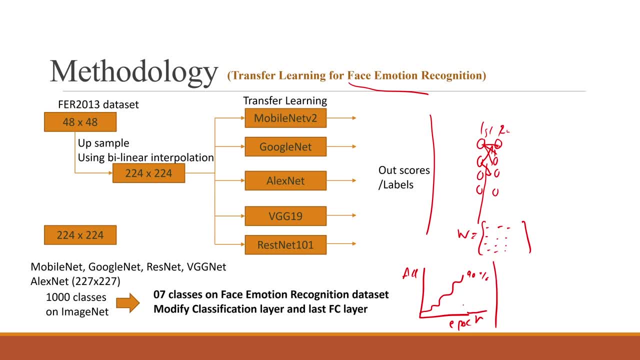 after long, long epochs. Okay, Now the question is, for example, everything was going on here for, For example- let me remove this. Okay, so everything I was doing here was for Classifying, for example, cat and dog and other elephants. right Once I have trained by spending many hours on my computer, or many days sometimes on my computer after training this. 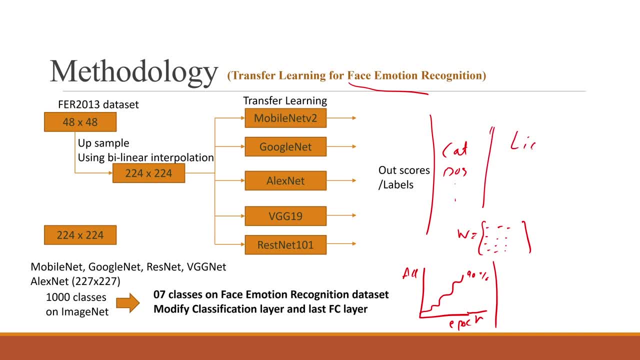 Someone. after one year or two years, someone come up and he want to resolve a problem line or elephant and any other kind of Elephant animal right. He want to classify this. So one solution is that he have to train everything From the scratch for many hours again and it will waste his time. So rather than reinventing the wheel, 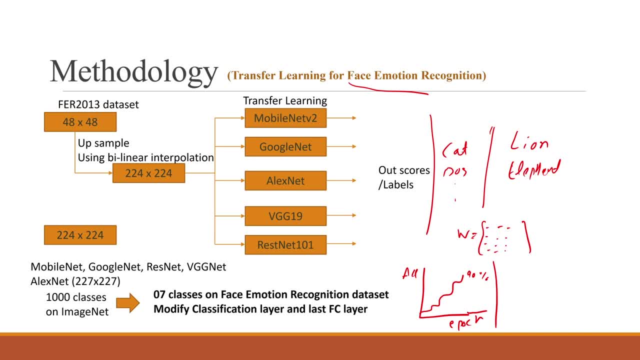 So actually, what happened when we were training between cat and dog? it happened that our weights start randomly. It was random, right, So we started with the random and then we want to modify according to the For getting more accuracy right, for getting more accuracy for cat and dog division or classification. 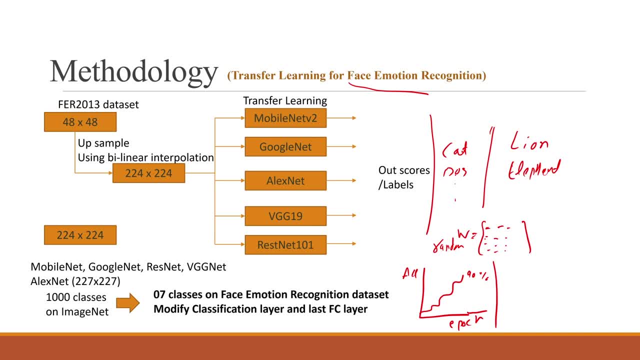 now we come up with a line and and Elephant problem. So what we need to do, the transfer learning, is the best thing, because transfer learning- the name says that We do have learning already, We do have knowledge and we are transferring the knowledge and learning by transferring right, so we can just take this same weight. 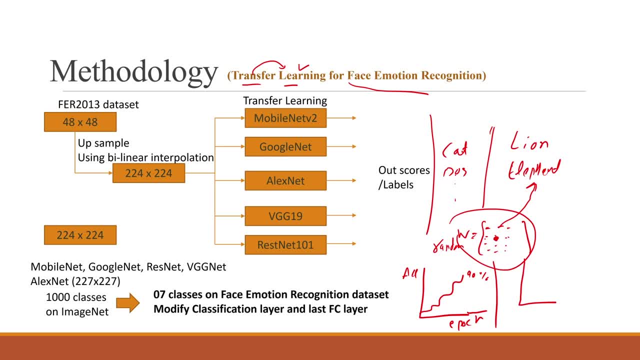 Apply here and we can modify only those weights because you know, both of them have four legs right, Four legs four legs right and a lot of maybe. the texture of their body might be Same some time: cat look like a line right and a lot of other similarity would exist. 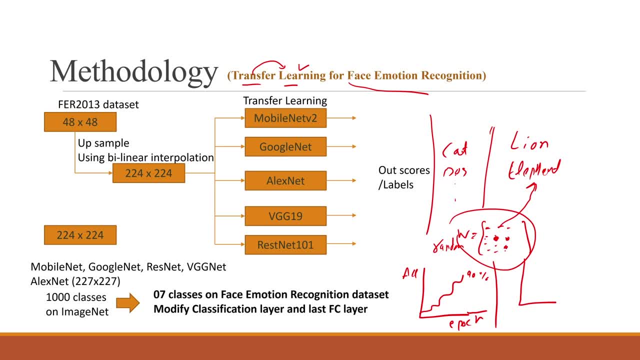 So it will only modify those weights which are exactly related to line or Elephant, particularly broadly speaking, they are all animals, right? so in this case our Hopefully, definitely you will see in the coding It will start 40 to 45 maybe, or a good accuracy will start and you will need only a few box. 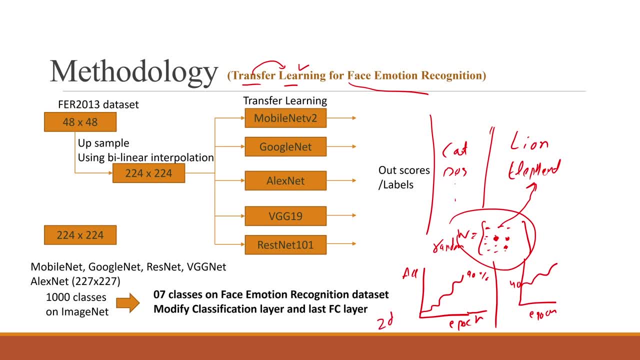 So if it was taking, for example, Two days or, for example, two hours train in this scenario, it will hardly take few minutes and very few epochs to train. why? because it will only modify those weights which are particularly related to line or elephant. so in this case, what we can do, we can achieve an good accuracy or maybe 90, again with very few epochs. 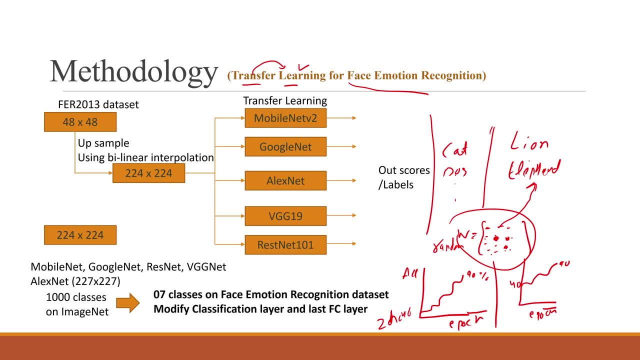 only modifying those weights which are particularly related to a new problem. so in this scenario, the nature of the problem must be same. so, uh, you might have noticed why i have draw a lot of these things. so, okay, now coming to this point, what was here so many years ago in 2012? 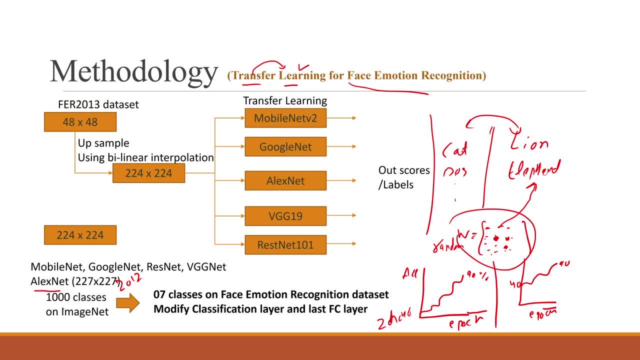 lx net was used for the classification of thousand classes on image net data set. it contains a lot of classes. they are 130 gb data set, a huge data set, right? so the lx net in 2000 classify all these thousand classes with a good accuracy. okay, then over the years, mobile net is. 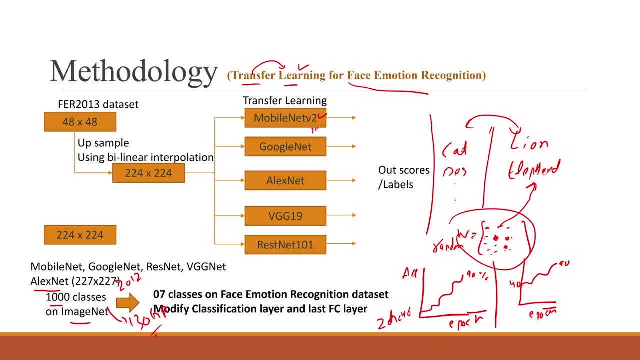 the almost latest one in 2007, 18, i guess, maybe 18. okay, and the google net is its older one, but it's also by google and alex and i told you, and vgg net 19 shows the 19 layers, right, not the year of. 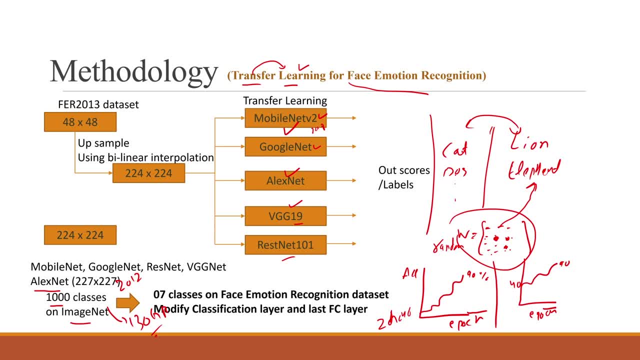 the 19 right. so resnet and a lot of deep learning architectures over the years have just overcome previous problems and they have just modified their weights, and they do exist on internet already, right. so rather than reinventing the wheel, rather than proposing a new architecture for face emotion recognition, it's a best way or good solution to use the existing one. they 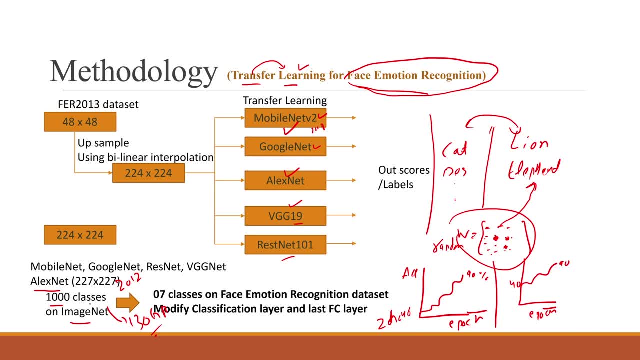 were trained for thousand classes. all we need is to just modify these weights for the seven classes. okay, now the question is: now we have just understand, uh, that, uh, we, just you get the idea what is transfer learning. now the second question is how to do it. how can we implement transfer learning? okay, so, for transfer learning, as we are just treating 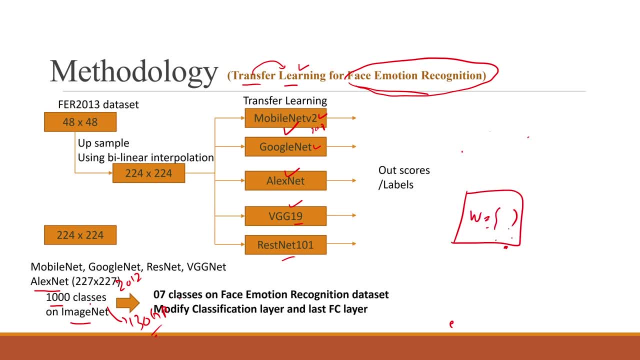 these set of weights, like a deep learning, like this is weight okay, so input and output must be same, or or input must be same, right, because they all of them. lx net was for 227 into 227, but mobile net all of them were two to four into two. four to four. image right inside: two to four into two. 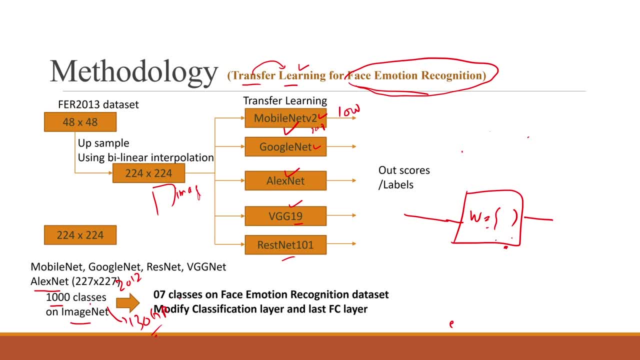 to four image. they were trained right into thousand classes, so everyone output is thousand classes, so on, and everyone input is two to four. that is why these are. these are connected, right, although they are separate algorithms. so in fer 2013, the data set is to 48 into 48, right? so we? 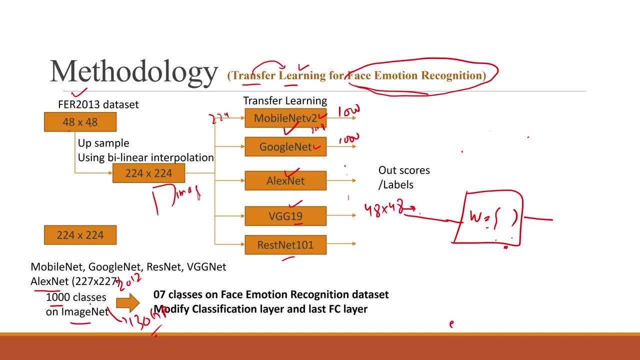 have to resample 48 into 48 into to write up sample using bilinear or any other technique. we have to do it 2 to 4 into 2 to 4, right, once we get the input same. now we can use the same weights. all we need is just modify these. 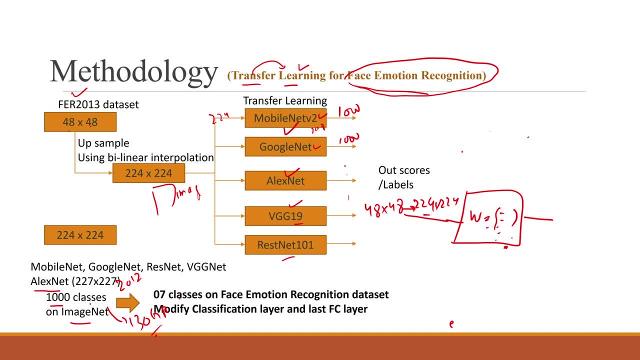 weights for face emotion recognition. we do not need to train everything in this way. you will witness soon in the video that while we will coding, it will start a very good accuracy from the start. we will get a very good accuracy from the beginning why? because we are not initializing. 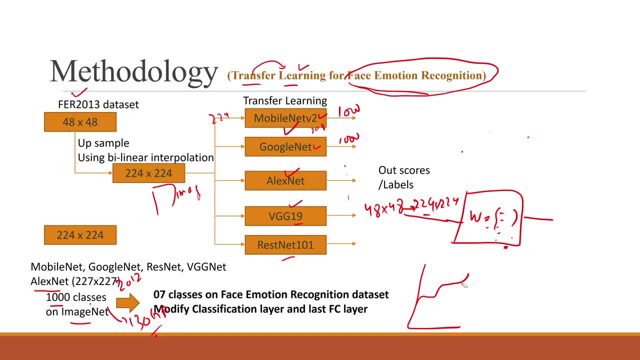 these weights randomly. okay? the second thing is that our output is different. they were designed for thousand classes. our output is 7. as you know, the fully connected layer- the fully connected layer- is always equal to the number of the neurons inside. the fully connected layer- is always equal. 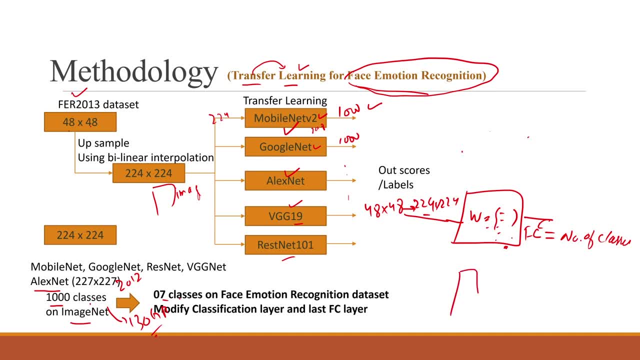 to number of the classes, as we already know that. so what we need to do is thousand classes there were. what we will replace this into fully connected layer having only seven neurons. so, for example, if mobile net or any any architecture, we have deep, many layers of the deep learning architecture, so on. so what we will do, we will only cut this fully connected. 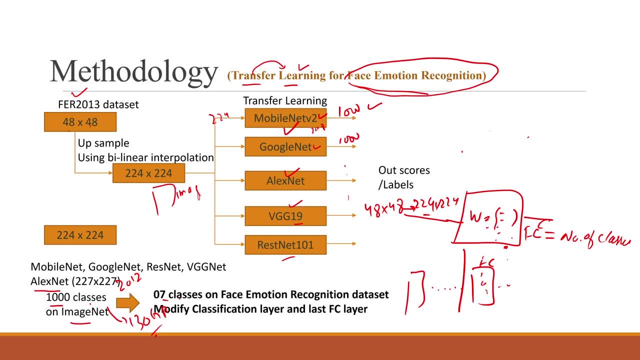 layer from an from deep learning architecture of the thousand classes and we will modify this thousand into seven, thousand into seven, okay, and then we will recreate a new one. and another things we can do. we can freeze some weights as well, but in this particular video we will not freeze any layer. but, for example, if your problem is too much similar, 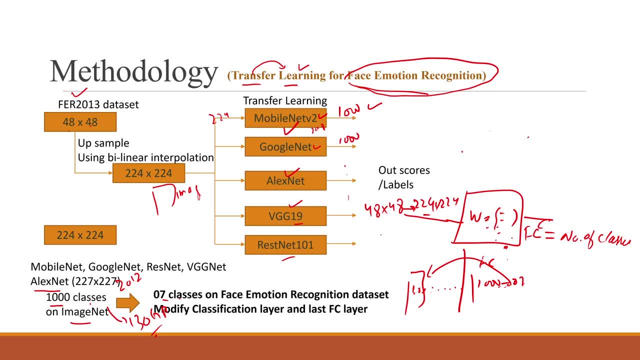 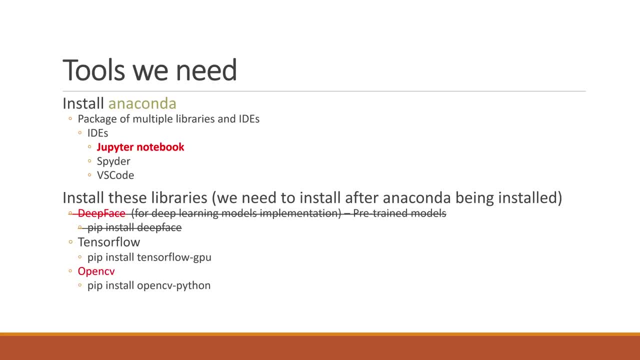 then you can freeze some layers as well. okay, so this is all about transfer learning, so now it's time to dive for the implementation, and the tools we will be needing for them is anaconda. anaconda is package of multiple libraries and, for example, different ids, jupiter. 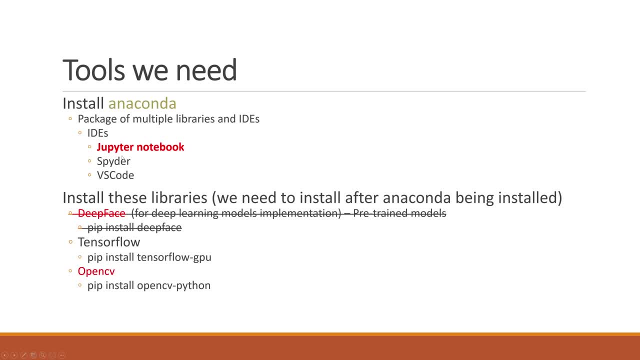 book, spider and vs code and many others are available in the market. so i would really prefer jupiter notebook and i will show you how to install, and previously we followed a video on deep face for beginners level. now we are slowly and gradually going towards a higher level. 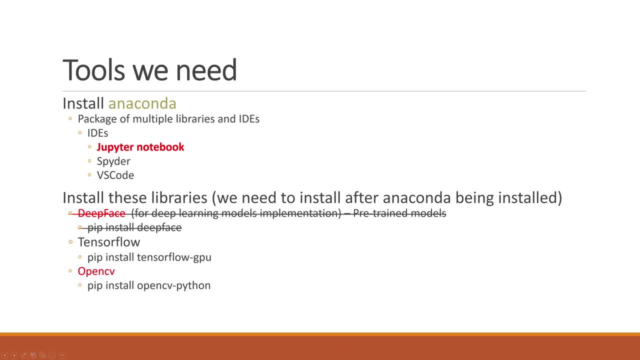 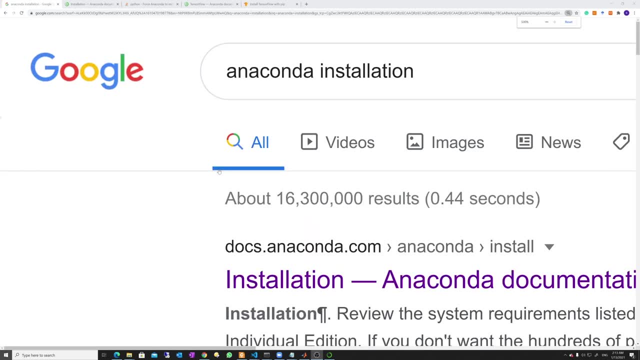 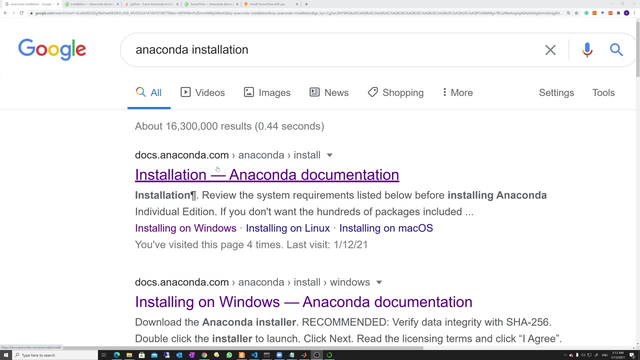 and these are the installations and we will shortly tell you how to install everything and how to set up for the implementing everything. in this section we will learn how to install anaconda and tensorflow and other dependencies. so if you already know how to install tensorflow and anaconda and your jupiternerd book, so you can just navigate to the coding section. but if 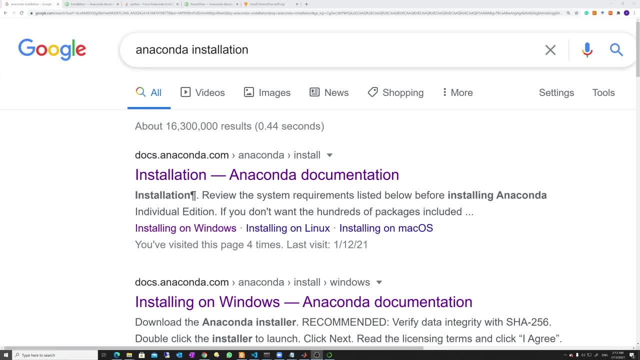 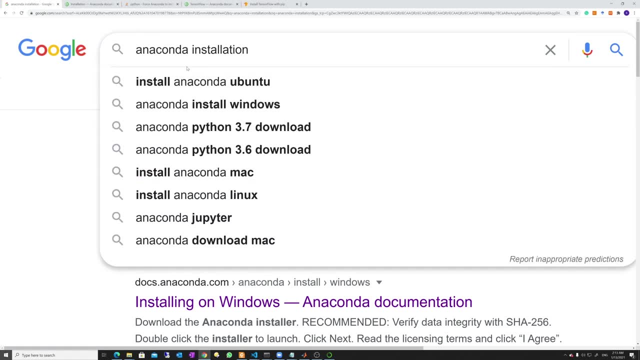 you do not know, please stay tuned so that i can just show you how to install. so all you need is to just write in google anaconda installations. once you write anaconda installations, as well installations, and you press enter, these kind of windows will appear. why i'm showing you this? 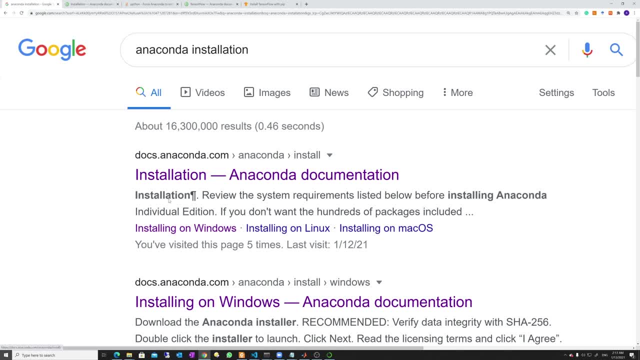 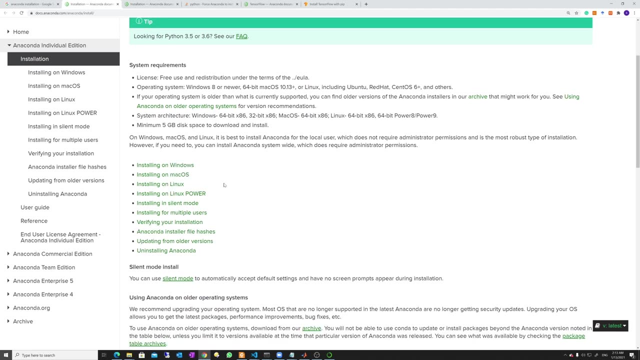 method because it's generalized one and usually the it's keep changing right, so all you need is to just write an account: installations. once you click open a new tab, this kind of installation setup will appear. so over here, based on your operating system you're using, for example, if 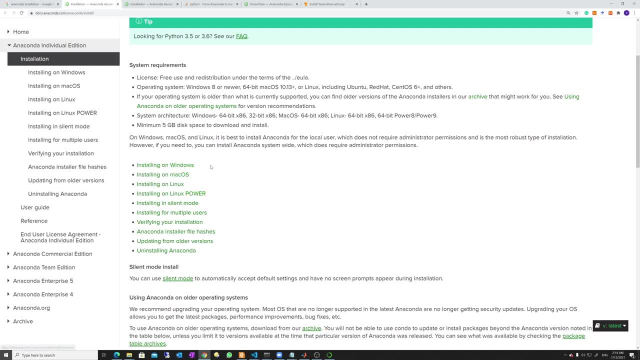 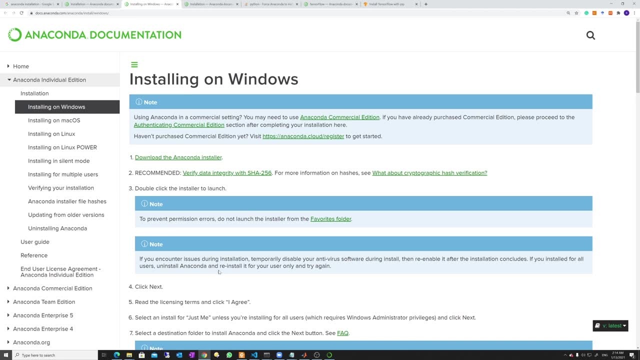 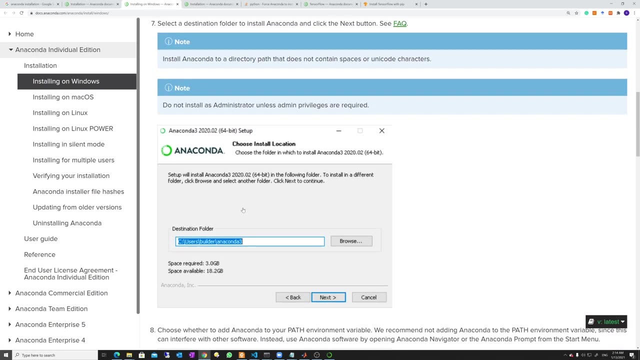 you're ubuntu user or mac os and other users, so you can just install. so as i'm using windows, i will just click this option once it is appeared over here so you can see over here you can just download the anaconda navig installer and then over here all the steps are shown. so we are lucky. 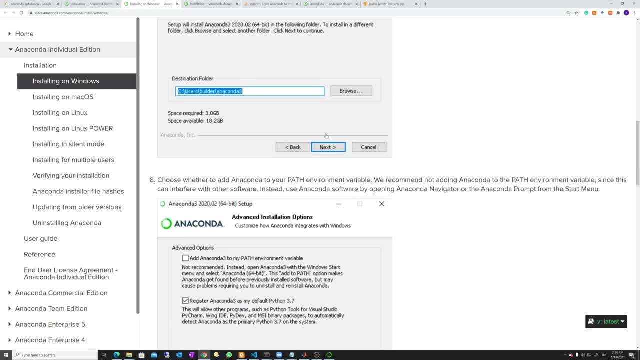 that we are using, for example, windows. so it's super simple. all you need is to just click next, next, and just install okay. so now i believe that you have installed the windows app, so let's go ahead and install the windows app. so let's go ahead and. 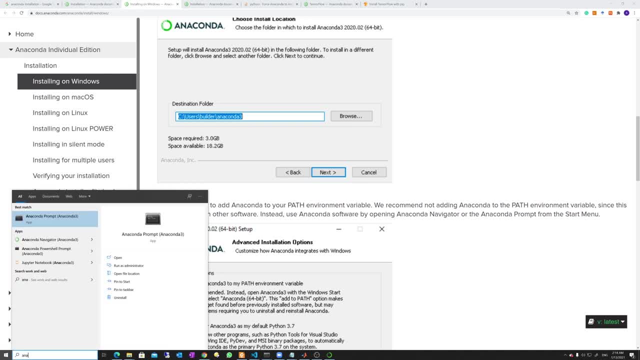 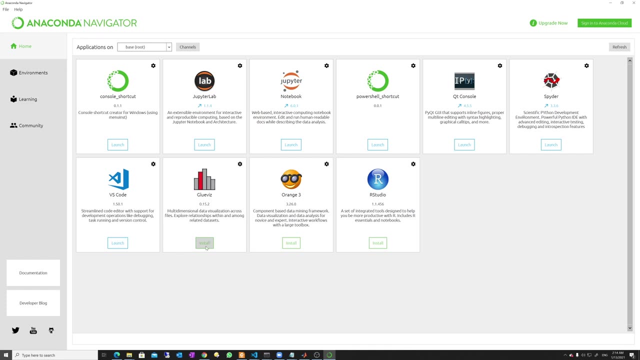 install successfully. install the anaconda. once you install the anaconda, uh, you can just write anaconda, and this time you need to press anaconda navigator. once you click the anaconda navigator, this kind of window will appear over here. you can observe that some of them are green buttons, like 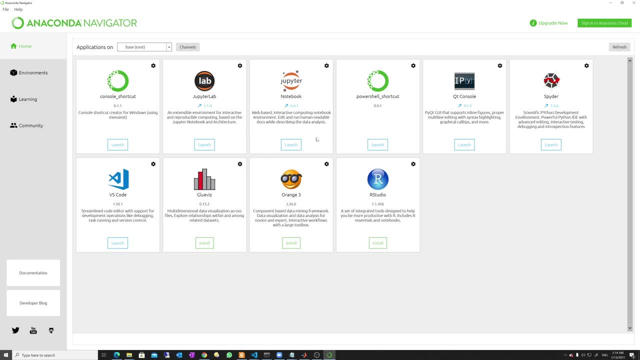 for installations, as i have already installed the jupyter notebook which we are going to follow for this tutorial. uh, this is. this has been changed to blue. one method to open jupyter notebook is to just click this launch button, but i would recommend you that you should better create a folder and then again you should go navigate anaconda prompt, not. 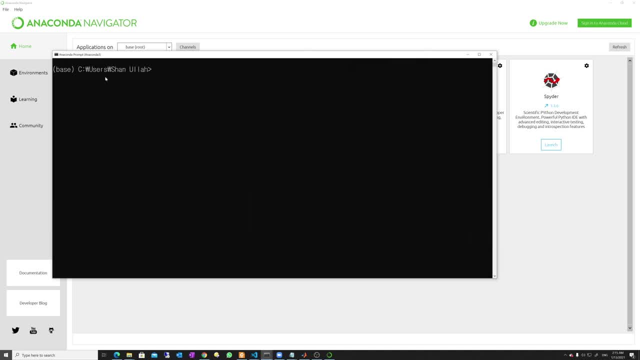 navigator. and this time, for example, i have created a folder and i can just move to any folder i want or just copy and paste from the explorer the path i can just copy from an explorer, like such as d, and then any of the path. okay, once i have done, uh, being navigated to a particular folder. 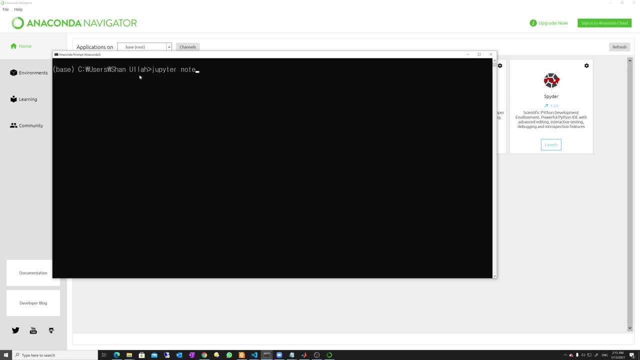 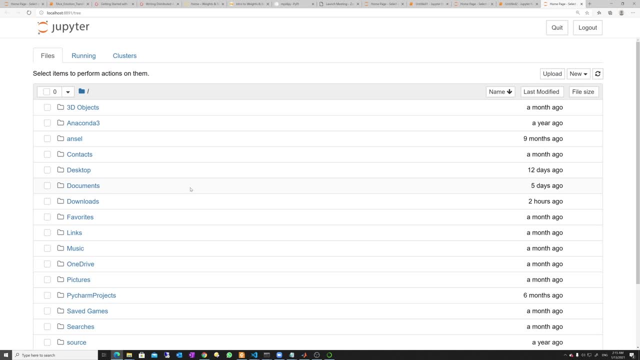 all i need is to just write jupyter notebook so it will appear. based on your default explorer, it will appear so once in the uh it. for me it has been opened in the microsoft edge, so now i can just open python and over here a jupyter notebook. 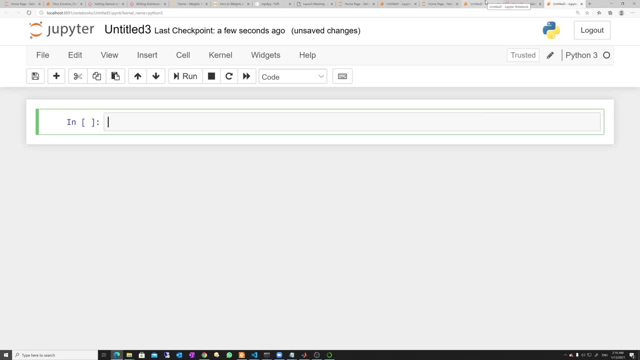 notebook has been opened. okay, so, or till this point, we have learned how to install anaconda and jupyter notebook. now it's time to learn how to install tensorflow. in order to install tensorflow, again, you can navigate to. you can just write anaconda and this time make sure you just run. 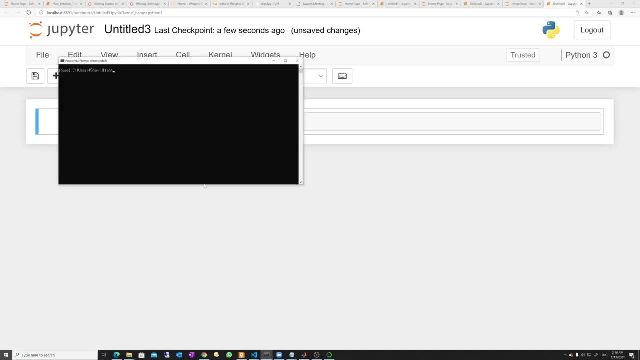 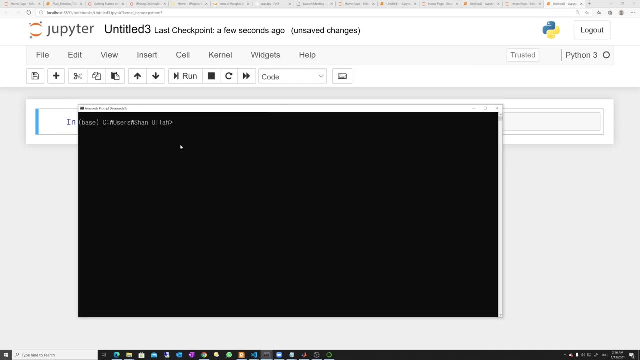 it as administrator. so once you again, you can just open as administrator. once you open, the first method is to install the tensorflow. is, for example, pip install tensorflow. this is the first method. so if you, if you do have GPU, you can just write tensorflow dash GPU. okay, if you want to install a particular version. 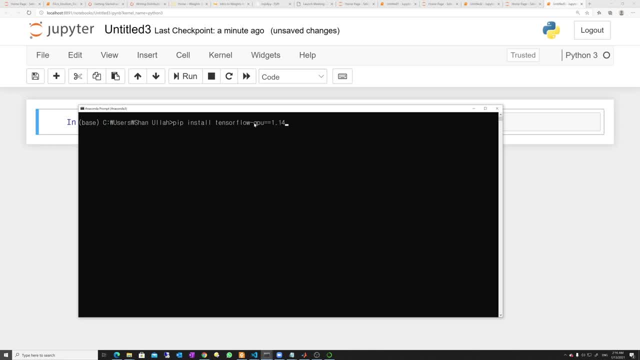 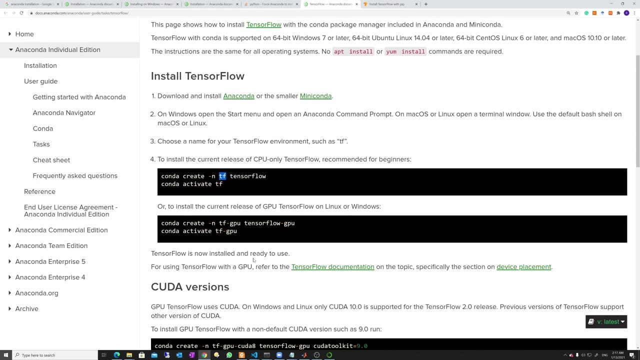 then you can, for example, 1.1.4 or any of the version. if you just do not write anything, it will install the latest version. this was the first method, right? the second method is, for example, using conda. so the second method is using conda. you can, for example, write conda: create and. 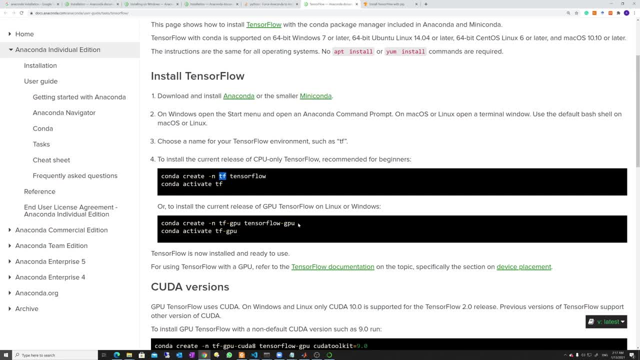 tfg GPU in tensorflow, dash GPU. so this is the second method you can install. so in this case you just write conda, create and tensorflow and all of the steps are same. rather than pip, you can just write over here. so both of the methods are better, but over here the good thing is that it would create a virtual 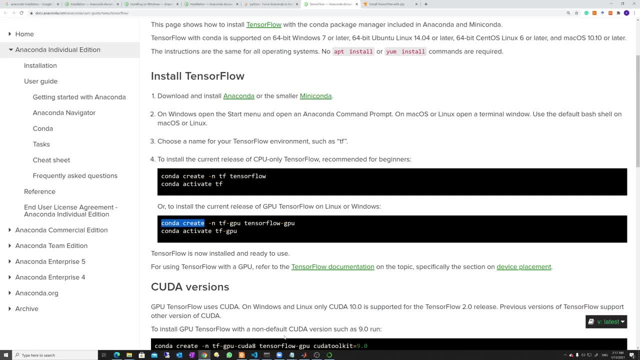 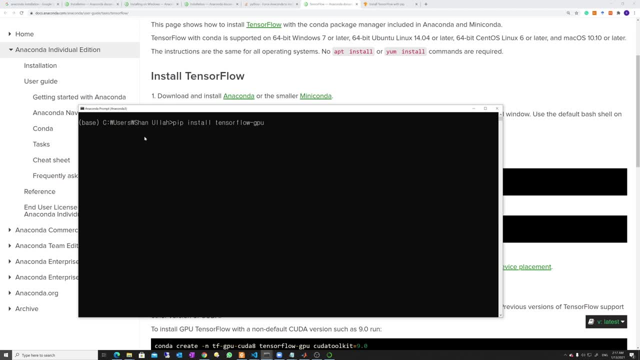 environment so you can separate. the best thing about anaconda is that you can just separate all of your things. for example, here you can see its base. so if i just write conda env list, so over here you can see. over here i have a lot of options so i have installed some of the tensorflow. 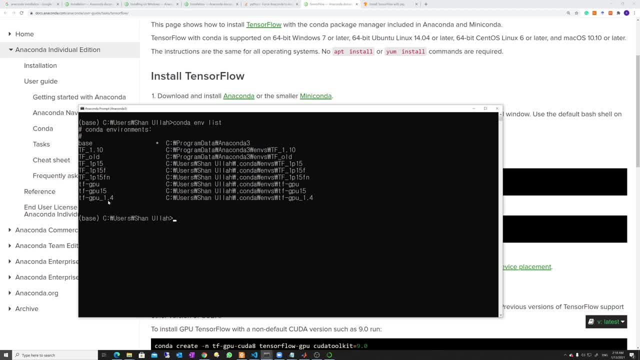 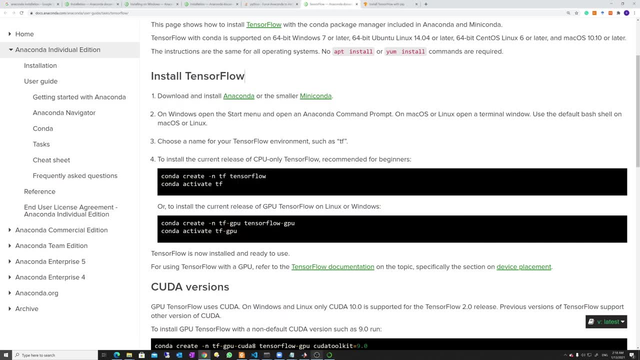 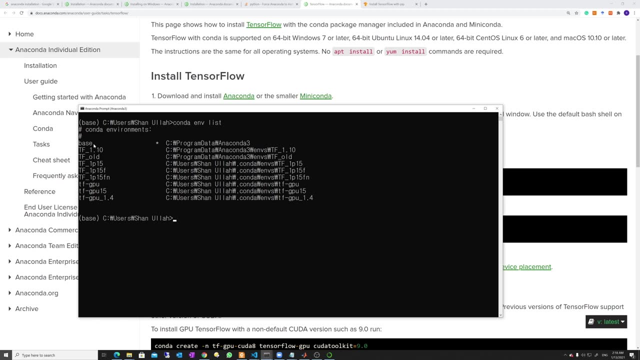 version in the base than older versions in other virtual environment. so this is the best thing about it: that contact create. once you do it, it would create a special- uh- virtual environment for you in which you can install. so if you want to check, if you want to activate any of them, 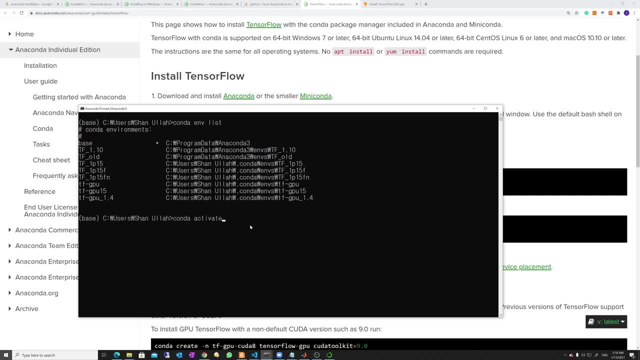 you can just conda activate. you can, for example, tf dash gpu. let me, okay. so this has been changed now from base to tf gpu, if i want to check which version is, for example, this: these are the names, right? is it's not actually tensorflow like this? 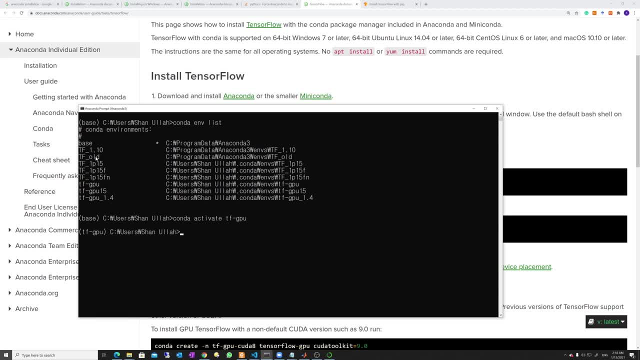 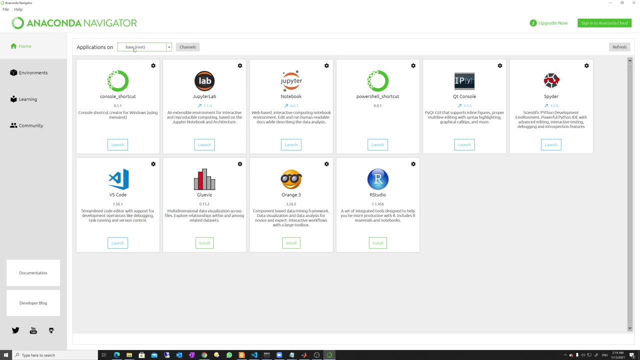 is tf old. tiff old is not any version, so i might have installed any of the version by the name tf old, but i would recommend you just write a particular version. uh, this this is the name- right name- of the version. so if i want to check, i can just click over here or see over here you. 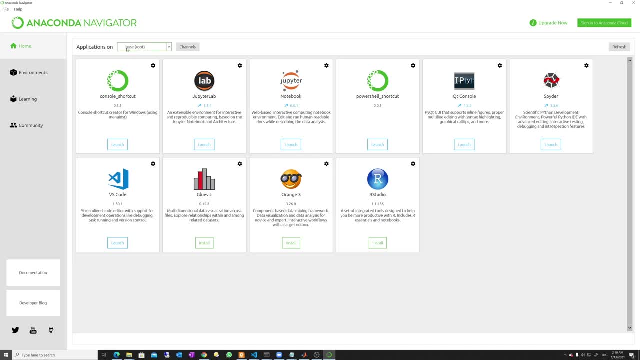 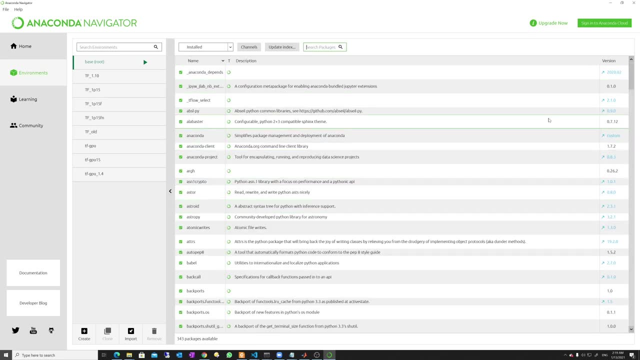 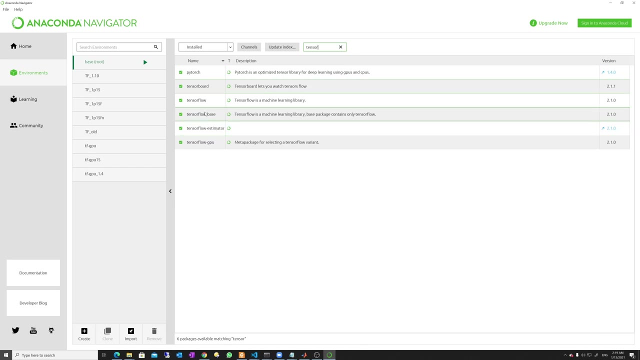 can see in the any conda navigator, the base is my environment. if i check the environment over here, over here you can see a lot of installations. if i want to check either i have installed tensorflow or not, so i can just search tensor and then over here tensorflow. 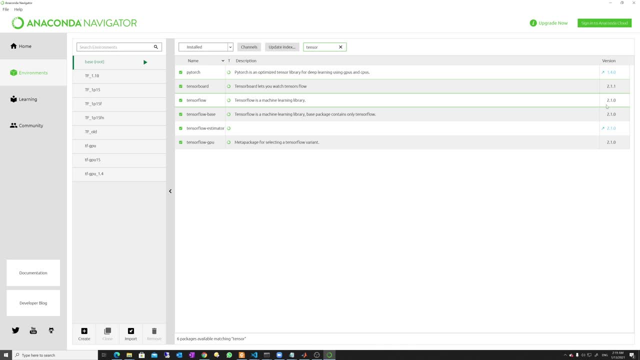 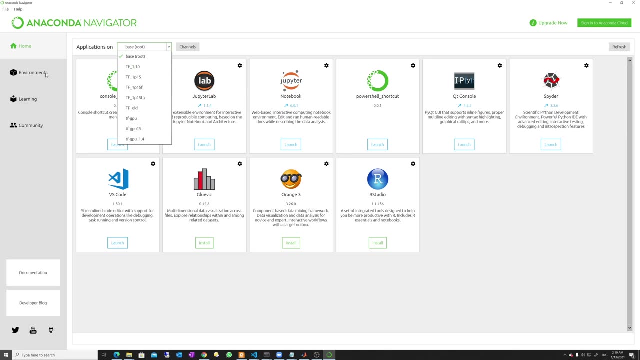 it will show me tensorflow and then you see, okay, it can also tell you which version you have installed. so you can just check, uh, click any of the version and then you can just go with the environment and you can check which version of the tensorflow you have already installed. 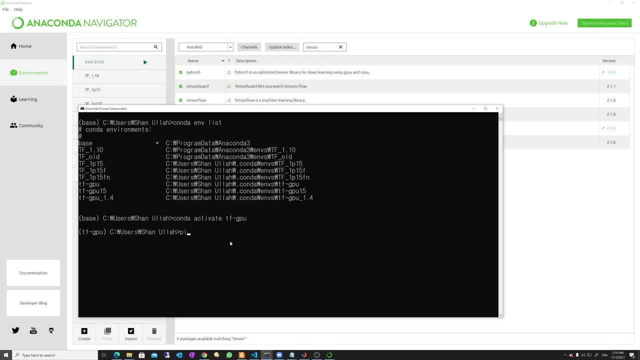 okay, so, uh, i have told you two methods. one is pip install if you are the beginner level and you do not know, uh, anything and you don't want to be confused, so the better is tensorflow dash gpu. it will automatically install the latest version for you. okay, on your default environment. but if 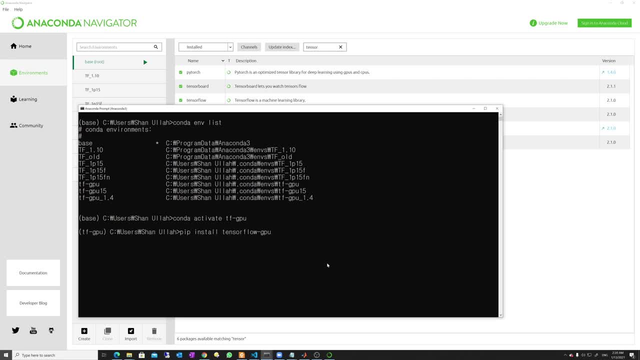 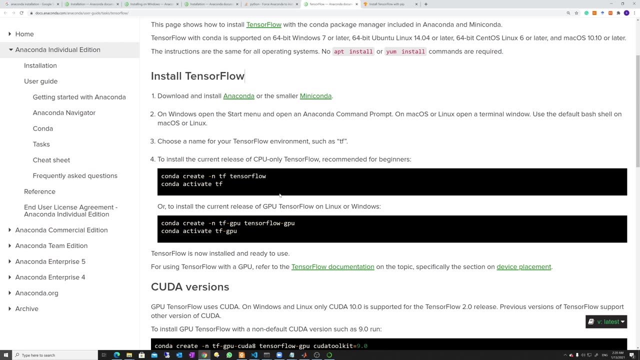 you really want to care and if you want to have multiple versions parallelly installed and you can just switch to any of the version, so i would recommend you to just conduct, create. just i show you over here, conduct, create and like this: uh, secondly, if, for example, later you decided that 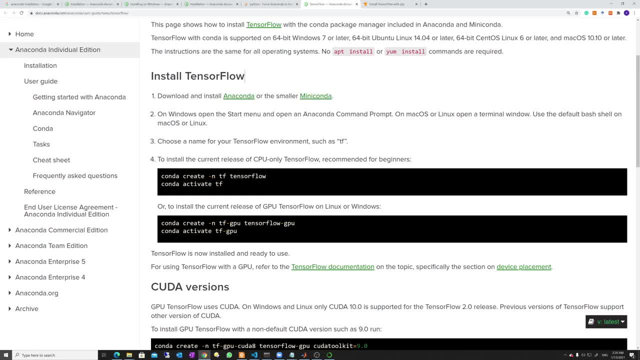 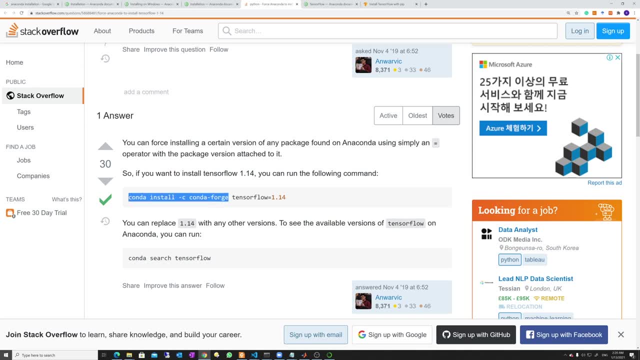 i don't want to install a latest version and i only want to install the older version. so then you can just write conda install forge like this. so what it will it does: it will uninstall all of the previous version and it will install the particular version. so that's it for today's video. 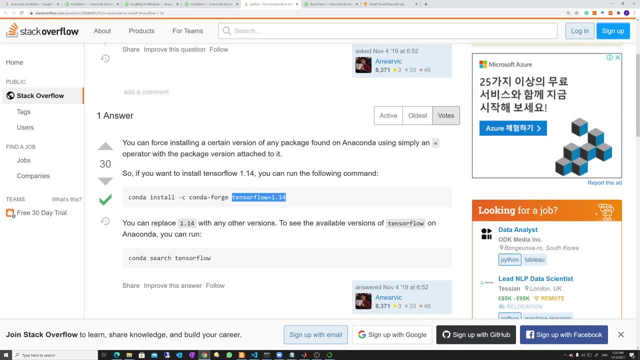 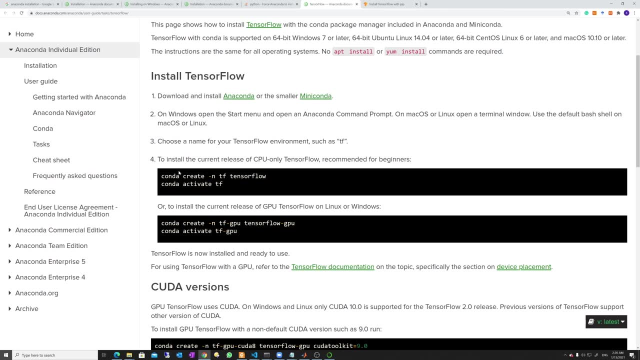 thanks for watching and i will see you in the next video. bye, bye. you are just pointing out. so this is the matter. otherwise, for fresh, fresh installation, it's better to do it, conduct, create. so this is. these are the two methods, so it's up to you. now we are going to. 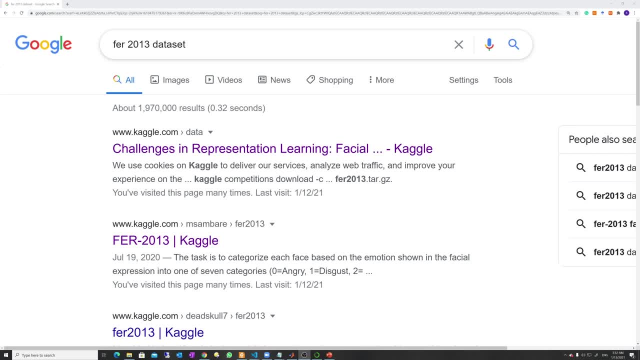 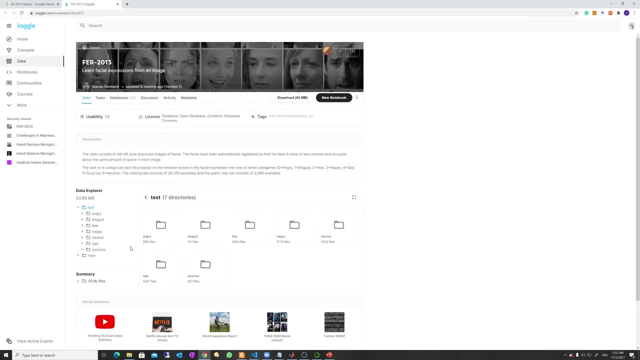 die for the coding section. in order to download the data set, all you need is to just find fer 2013 in the google. if you press the this enter button, you will find these links, and once you open these links, you will find the data set available on the kegel website, such as training and test data set is 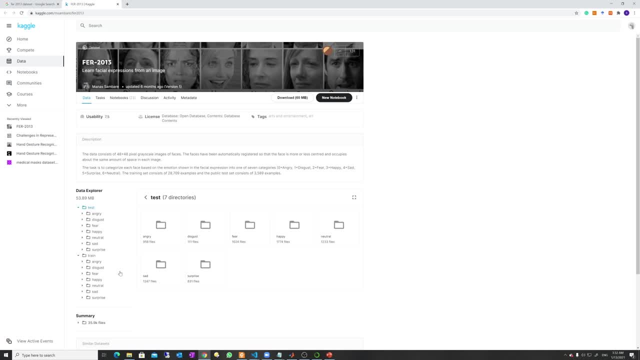 available. both of them have seven classes each and they have different files. so over here you can see that for training we have much more images because we will be using for training and for test purposes. we have- although we do have the test- similar folders but we have very less in number, so the distribution is always same. you don't need 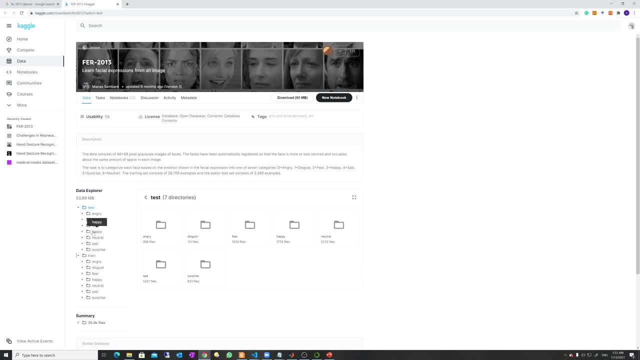 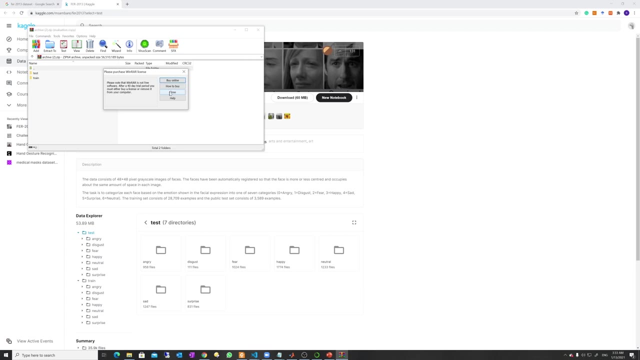 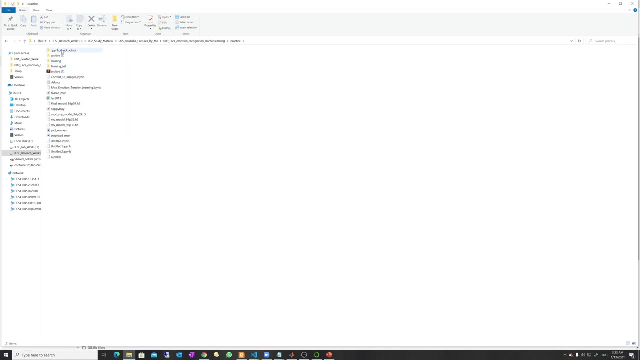 to care about the distribution. so test is for evaluating your model for the accuracy purposes. so once you, you can just click over here the download and it will start downloading, and once it's downloaded this pop-up will appear. so i have already downloaded this over here, this archive in which i have training and test. 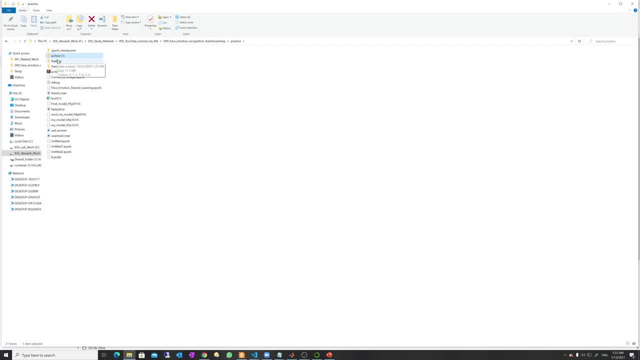 data set. so what i did is i created a folder named as training. you can name any folder, right, you can have any name, and then i have renamed 0 to 6. i did it because i need it for programming purple, so that the if else statement is easy for these number. so angry, i just 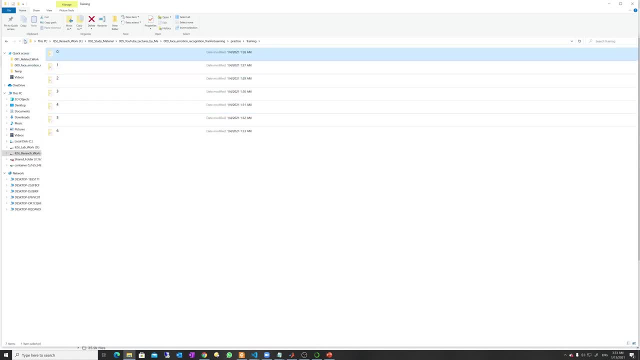 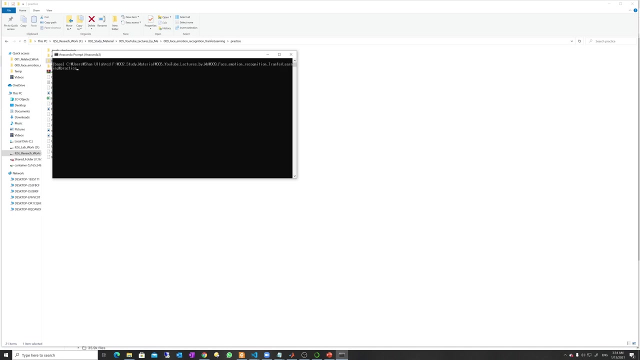 converted to 0 and so on. right explaining how to sideload. and so let me open. now that i have created the folder, let me open an account and navigate to a particular folder. then i will write: jupyter notebook, jupyter Álike, a notebook. and now let's say that these are our strings. and if i want to switch to jupyter notebook, then it can be changed to something with people and we will have to give it to this reader by name and name. if we name it jupyter entre aqonda, that means the methods for Repeat purposes, and i want it to be this one and to 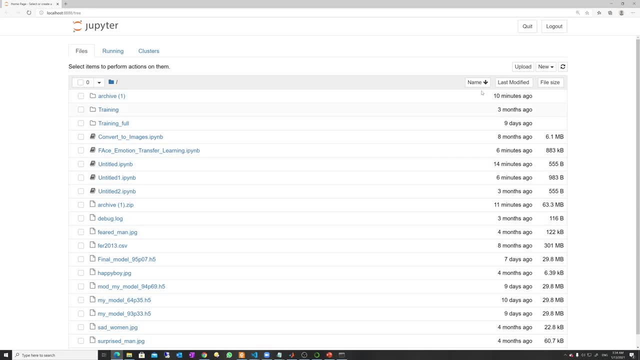 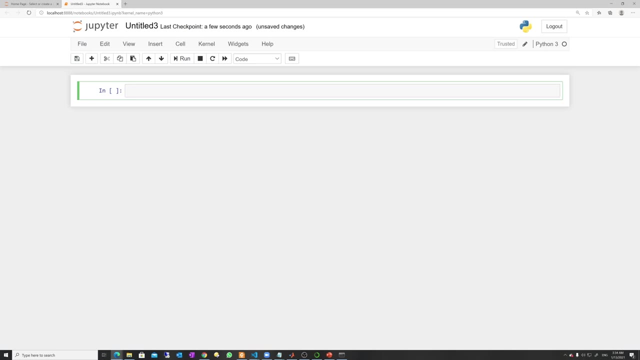 so this kind of window will appear so I can just click new and new python and let me open my nodes as well, and I will separate my nodes from here so that we can just start stepwise. so the first step is installations. right, so these are the 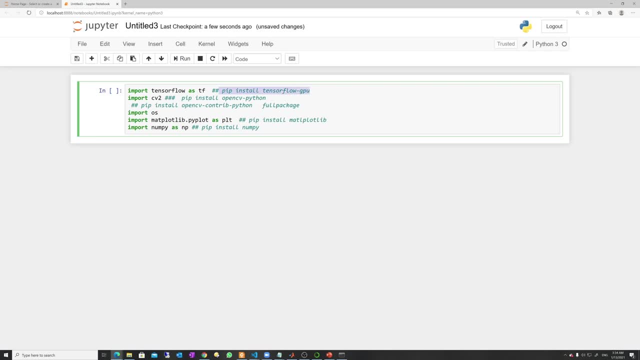 installations. I hope you have already followed the installations of the tensorflow and the same way, you can just go to anaconda and then open it, run as administrator and just write this: pip install opencv python. and for I recommend you that you install the full version and you don't need to install this. it's already there by default when you install. 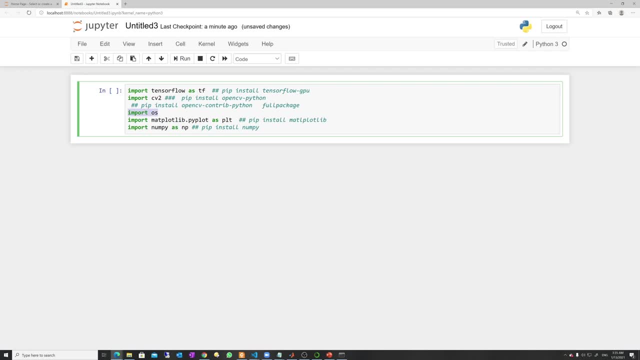 anaconda, it's already there for folder opening purposes. and then you need to install matplotlib and then you need to install numpy- so I hope you have already installed. or in this case you have to enter shift, enter. you have to press shift and enter right. this is a shortcut key. if you don't, 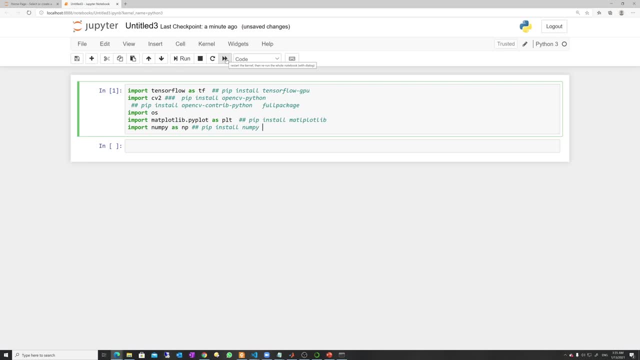 want to do it. you can just be over here and just click this. it's for restart, I guess. okay, you can just run and you see over here the number has been changed. but I follow. basically, shift enter, which is a shortcut key such as shift plus enter, right, you need to press like this. so shift enter. I executed. 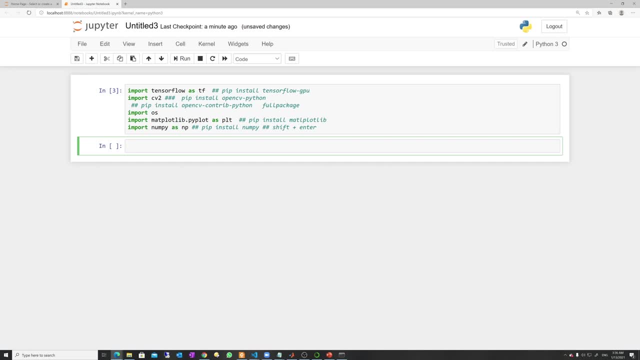 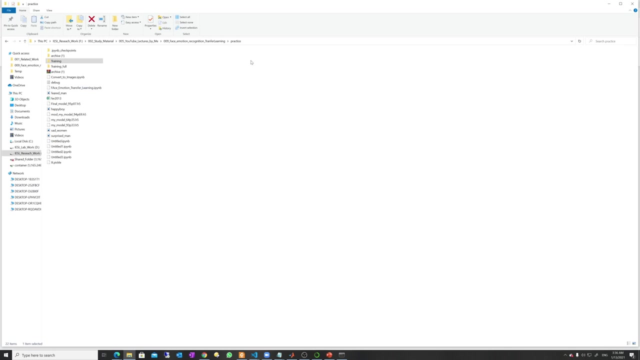 third time. so that is when the number has been changed. so now I can read the image. for example, I say image array is equal to cvt dot. im read training. okay, so i'm navigating as i'm here. i have opened this folder right, let me zoom for you. 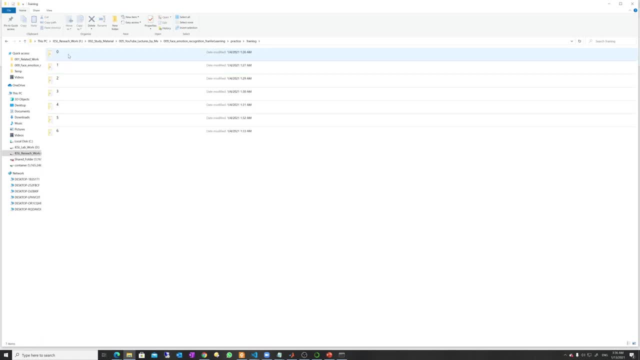 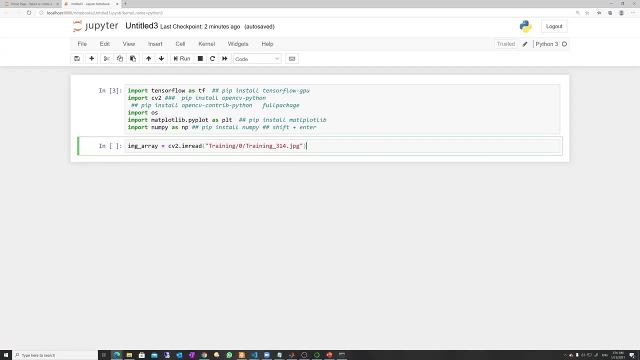 so i have opened this folder and this is the training and inside i'm just opening zero and whatever is my first image? i'm just reading that. so inside cv2, i'm read, is the command. okay, let me show you again for example, if i want to do it again: image array is equal to cv2 dot. 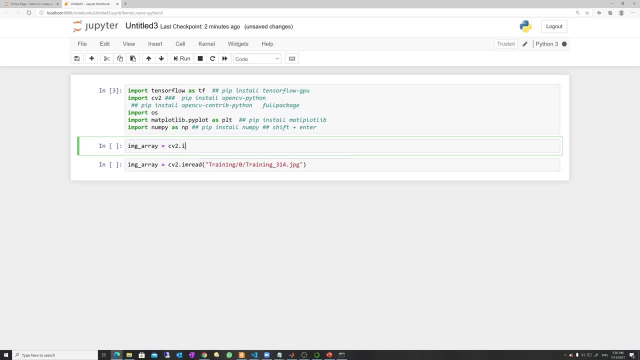 when i write and if i press tab, there are a lot of options. when i said i am, you see how i will get, i'm read. so, and right now i'm reading the image. so these this is as i'm in the corresponding folder. so in the corresponding folder i'm just reading a particular image, such as 314, for example, why? 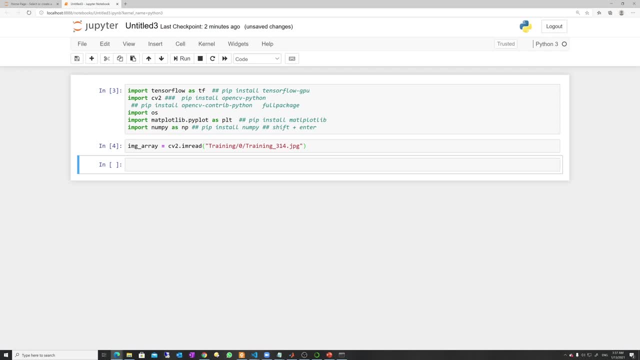 if i press shift, enter- now image has been read. i can check the size of the image dot shape. if i write the shape, see it's 48, 48 into 3, so it's rgb, green channel, sorry. rgb image, okay, as the name says. rgb, red, green, blue- okay image because it has three channels usually. 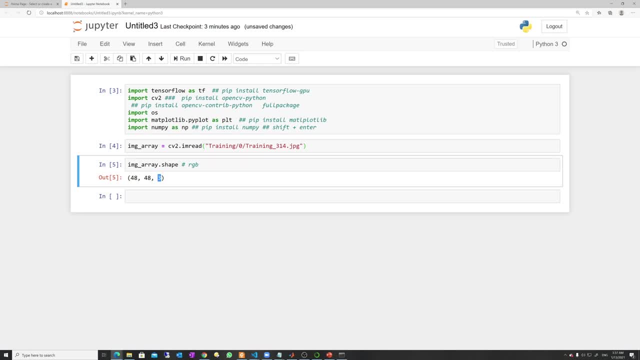 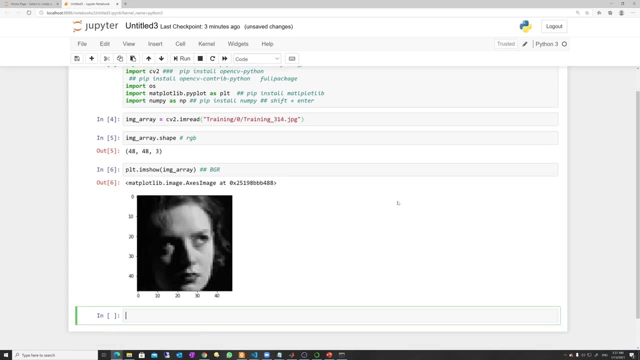 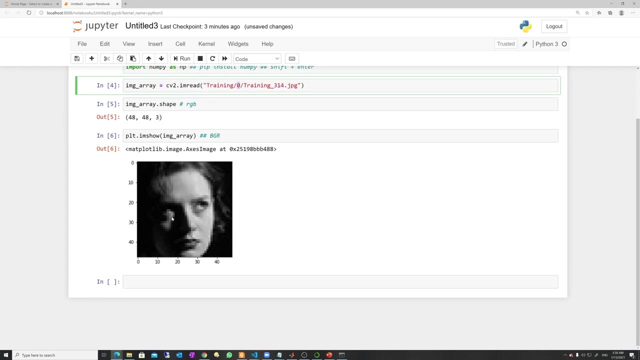 if it is not rgb gray, then it is one, so let me plot it. okay, if i plot, this is uh, as i said, it's zero and it's angry class. so this is the image. see over here. it's very uh blurry image because it's 48 by 48, too small image. 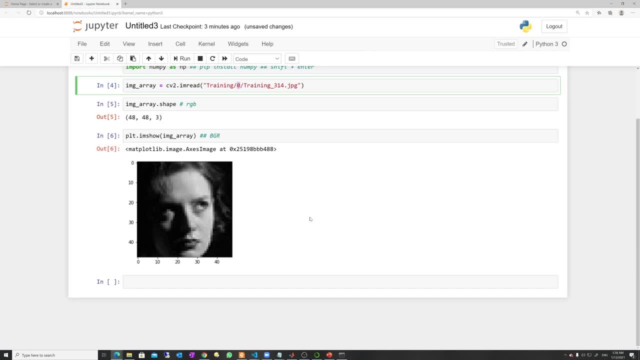 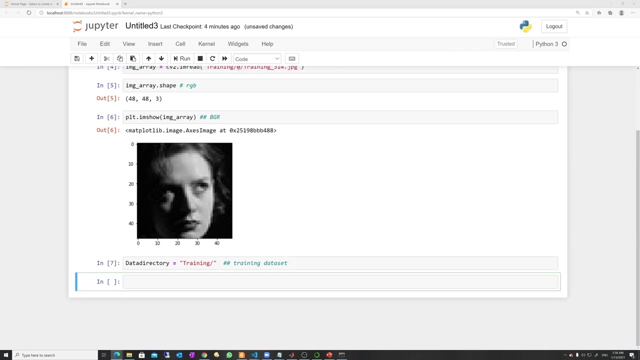 and we want to show it. that is why, actually, it's not that blur, but in order to show us it has shown that it it is a kind of blur. then what we need is: let's create a data directory, such as training, so the training data set we have, and then, as I 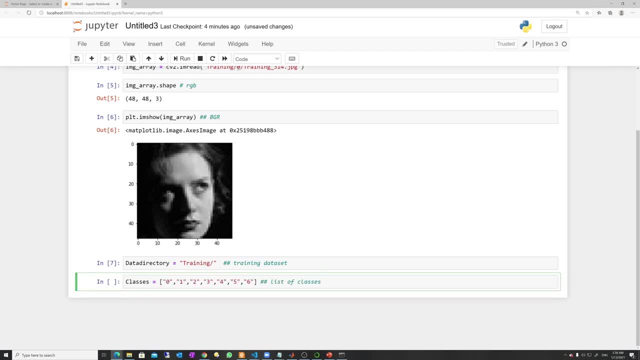 show showed you that how many number of classes we have, like 0, 1, 2, so over here. if whatever is the name, this must be exact name of your folders. it must be like this: okay, so as I showed you that I have created and inside the training, I 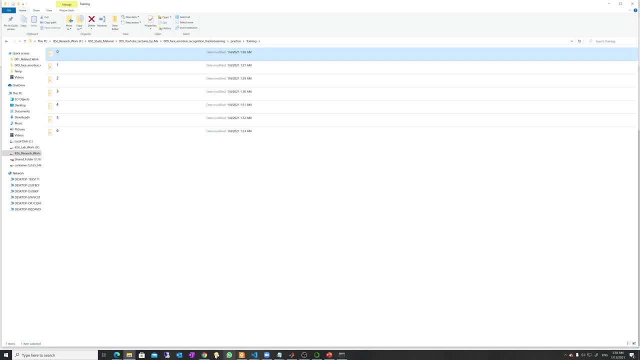 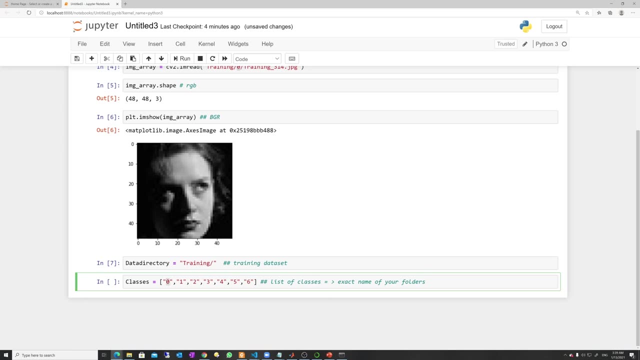 have created 0, 1, 2, 3 up to 6. I have renamed. if you haven't renamed, please just follow the the same name, right? if you it's angry and other things, then you can do it angry and other, right? so if you haven't? 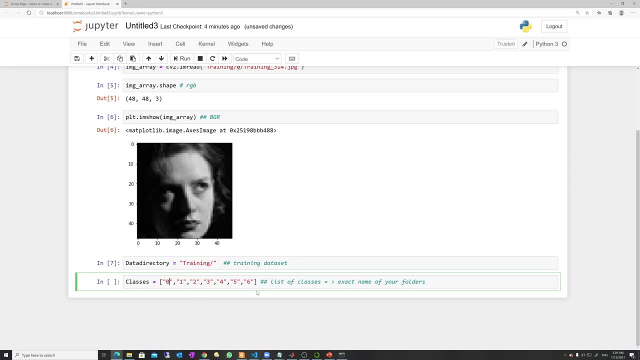 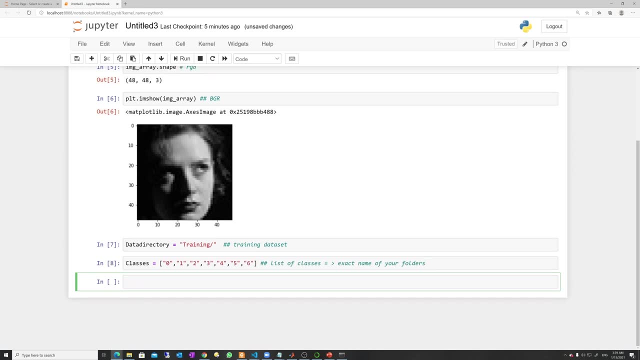 done sub to you. so it's for me. I 0, 1, 2 is programming the easy, so that is why I just convert it in. so it's totally up to you. now that I have created, let me read all of the images, as I read one of the image, so let me read all of the images. 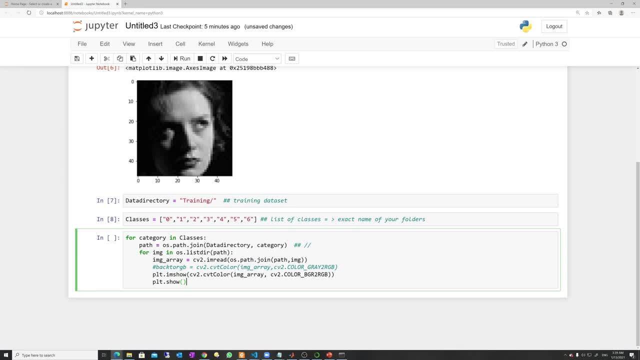 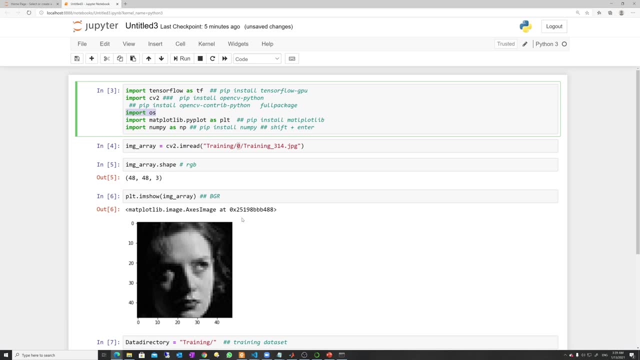 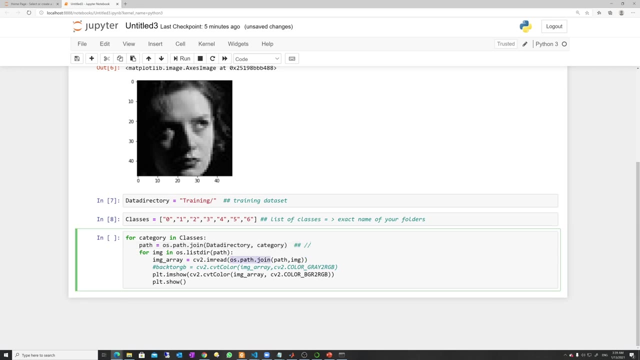 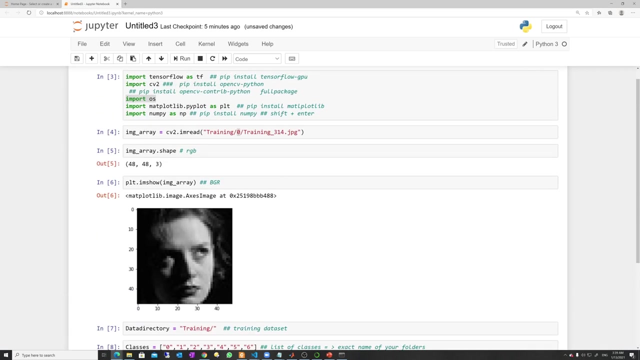 so I'm just having a loop for categories in classes. so I'm just part that OS as I have just used. import the OS. now all I need is to just OS dot list directly. so all parts will be given and all part will be provided and I'm I will be reading all the images, okay, so 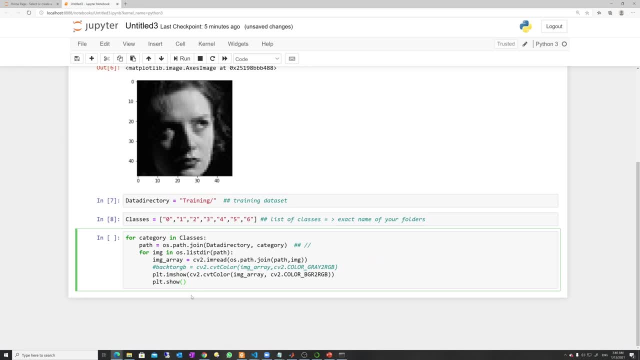 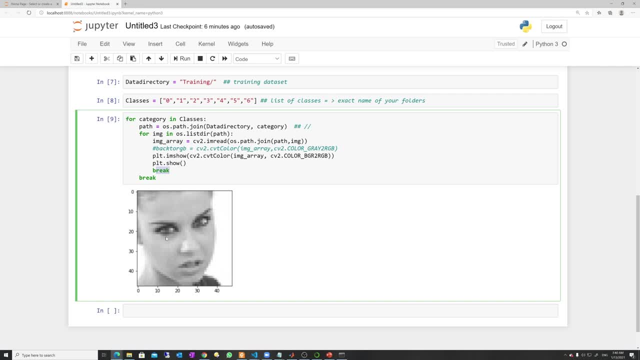 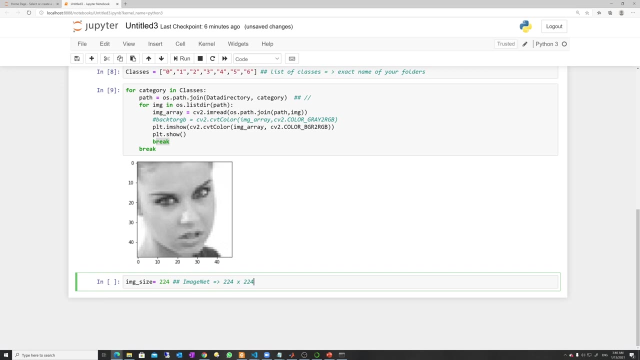 this. this will be start showing all of them. so let me execute this. this will be start showing. establish that my first code is being read. so the second method, sorry. the second step is to change the size of the image, as we know that for image net we do have two to four size, so it's 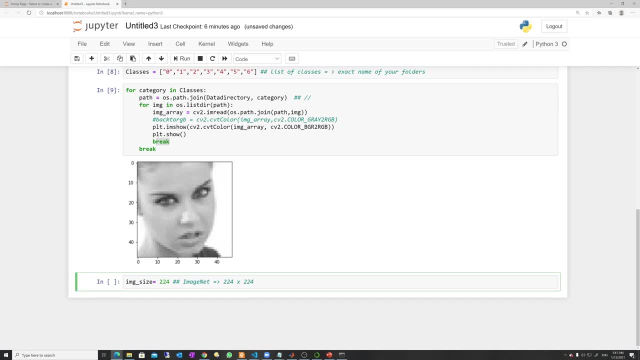 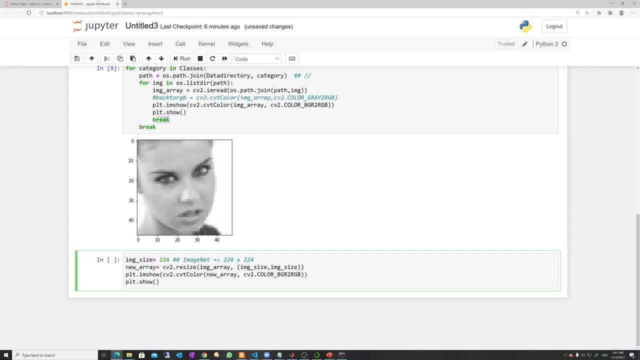 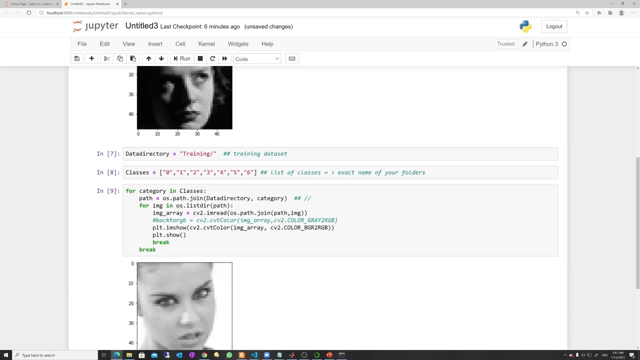 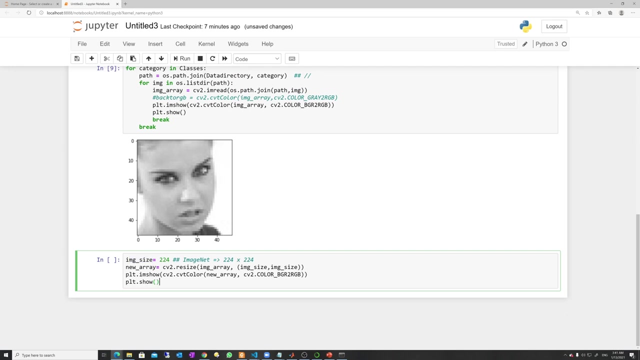 better that we should have change the size of the image. let's change the size by cv2.resize image array, this image array we need to change, and then image size. so two to four into two to four. so it will change this 48 into 48, into two to four, into two to four. right, and then i'm just showing. 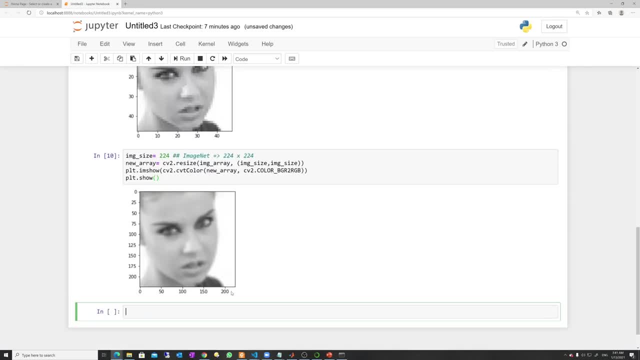 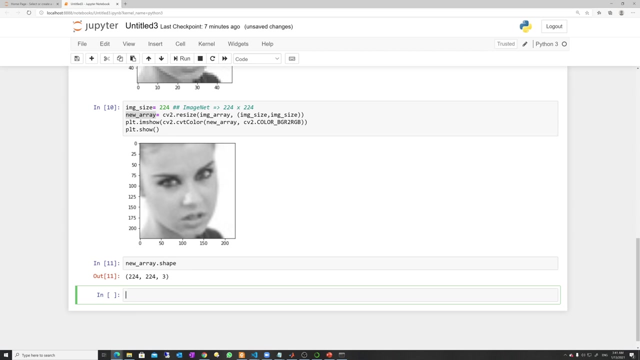 it. let me do it. you see, so now it becomes two to four into two to four, if you, if i want to check the new array size, if i execute it is to four into two to four. why i did it? because i am using transfer learning. so for transfer learning, 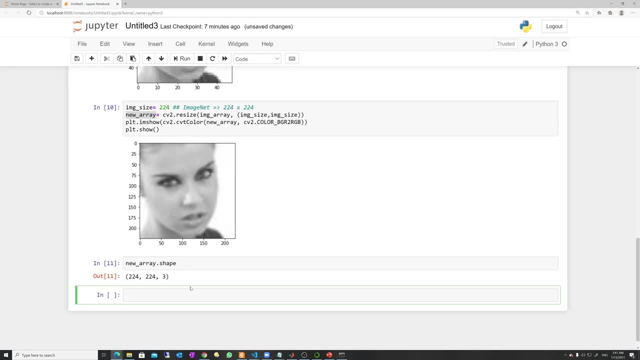 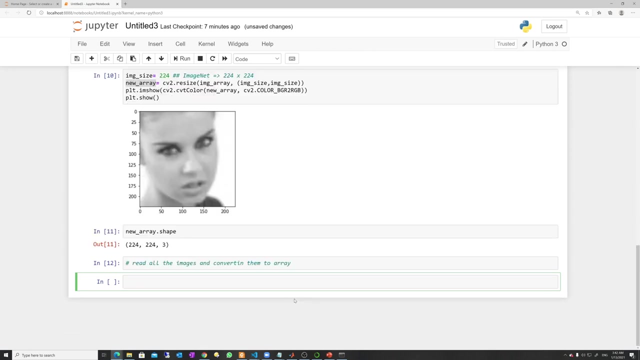 if i want to use any particular deep learning classifier, so that takes two to four into two to four. that is why i'm doing it. so let's do it: read all the images and convert them to array. so, although we just did so, the one best thing is to just convert cell into markdown. 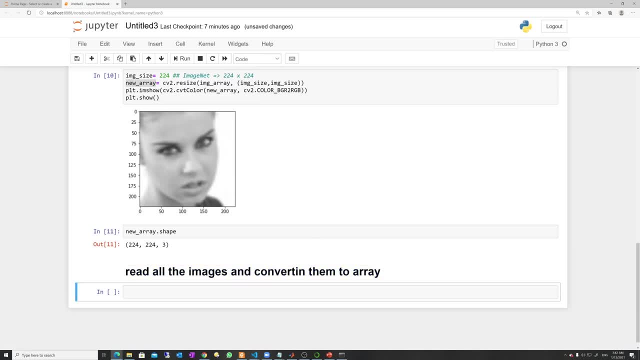 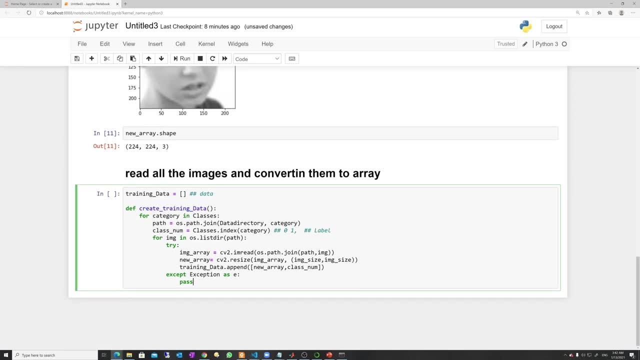 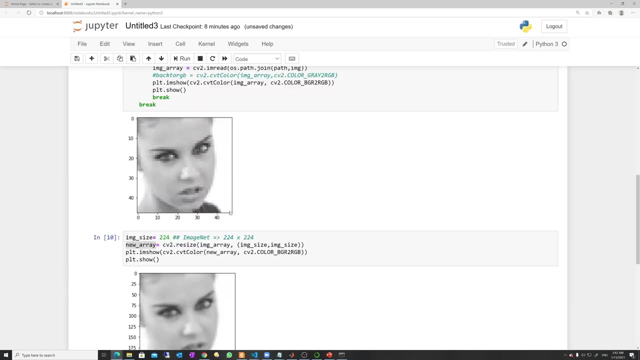 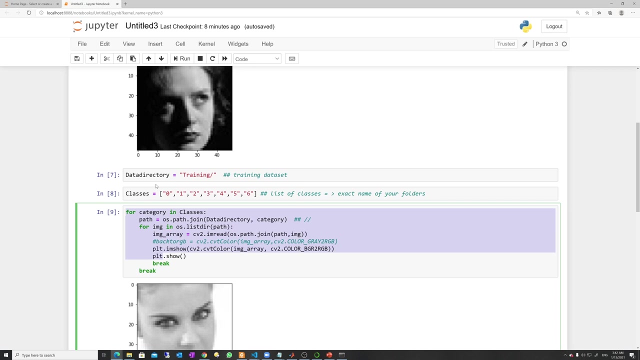 so that we just convert into the nodes. so, as i did it before, let me do it like this. so now i have created a full um, a function, right, daft, create training. so all i did is just copy all these come and and commands. i just changed the data directory to training data. okay, so that i have already executed. 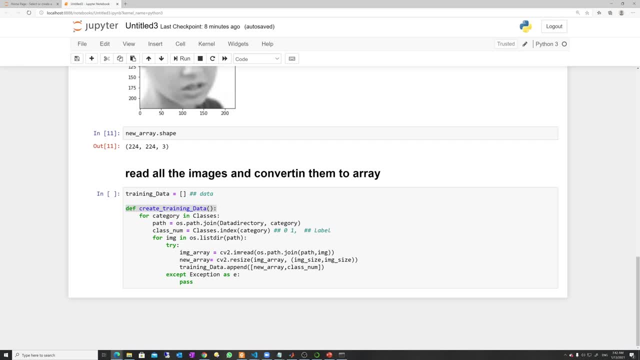 uh, data directory and categories, all of them. and now let me save everything in the training data array. right, so this will be array. right, so we are. i will read all of them and then i will convert. i will just store all of them in my training data. error. okay, this hasn't been executed. 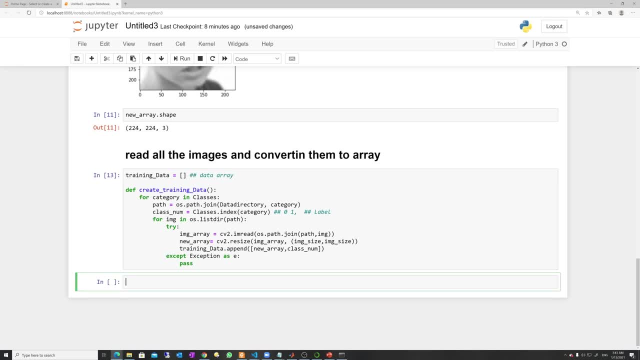 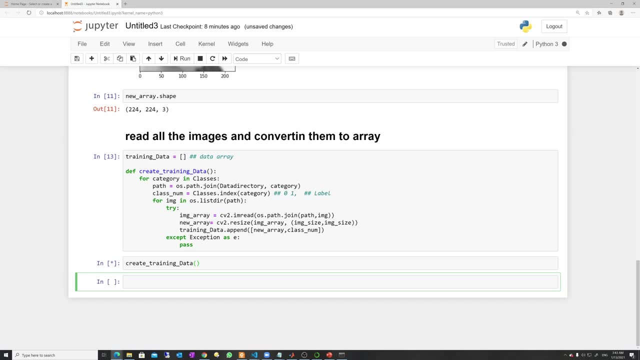 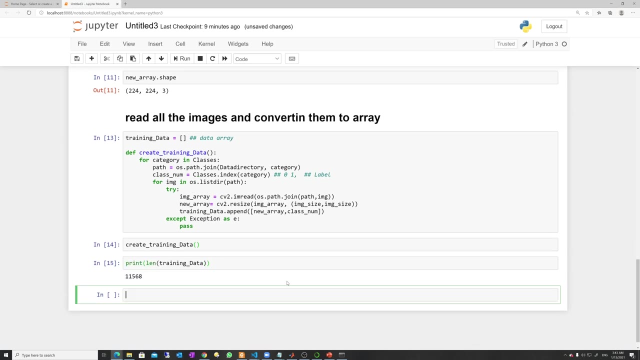 yet why? because i haven't called the function yet. so let me call the function and then again shift, enter. once i read that it has started reading all of the images, so it will read all of the images. now let me check how many images it has read, so i have actually shortlisted few of them. 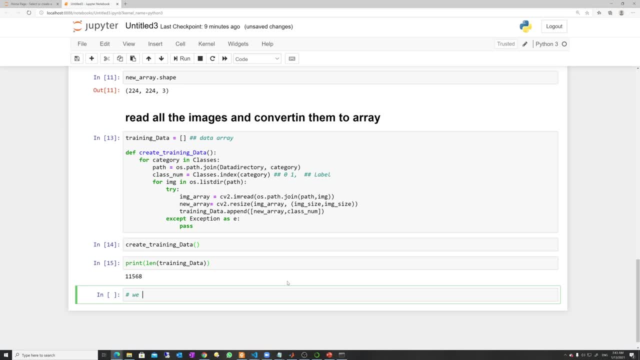 because i'm not doing it. we are just using training and deploy, deploy, deploying for real time webcam demo. so we are not proposing any deep learning architecture and so we are not interested in accuracy- although we do have interested in accuracy, but for just drill. i have just shortlisted. 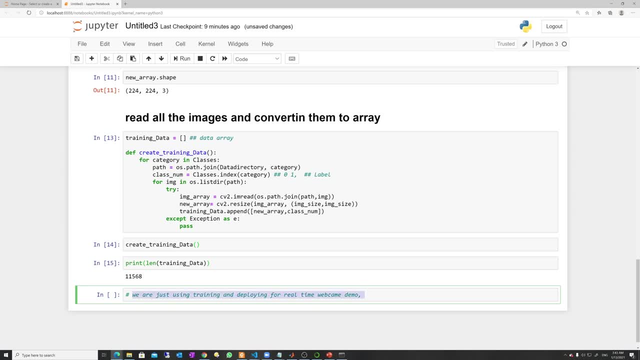 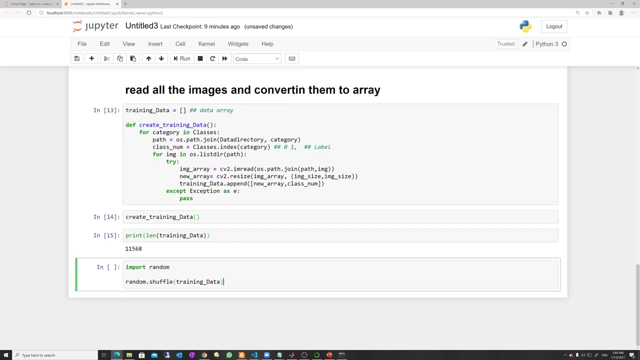 few of them. so in your case you can also do it. so even you can run raw as well. so it doesn't matter, you can just draw, it still perform well. but for as there are too many images, so that is why i have shortlisted them, because for real-time demo, i'm doing everything over here, i'm doing everything live, so definitely. 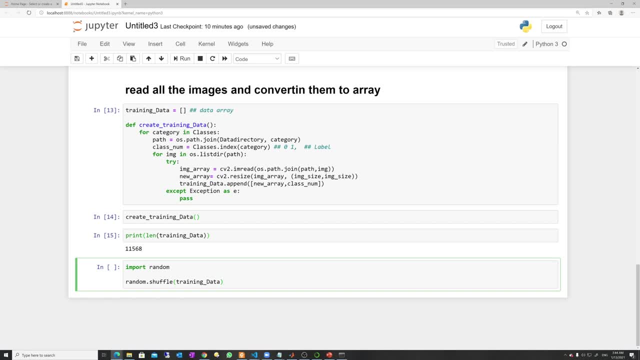 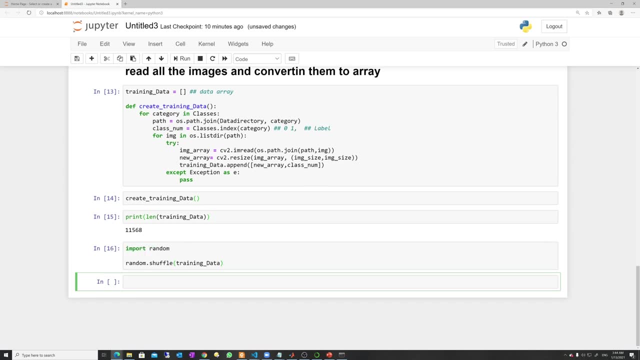 it would take time. then i have to stop the video and then if it there are too many images, so that is, i have shortlisted them, so let's import the random and randomshuffle. so what i'm doing over here? so i'm just shuffling it. why? because 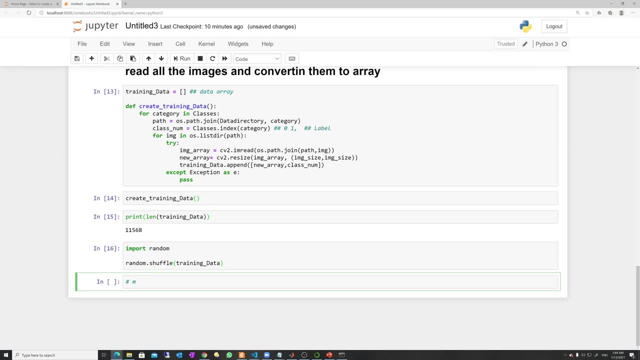 my deep learning lab. my deep learning model should not be. should not learn what is the sequence right, so it should not learn the sequence. that's why i'm just shuffling it, so that my deep learning architecture should be dynamic and robust and it should work to all of them. 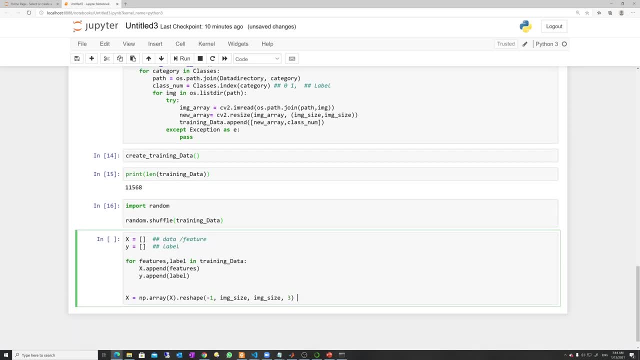 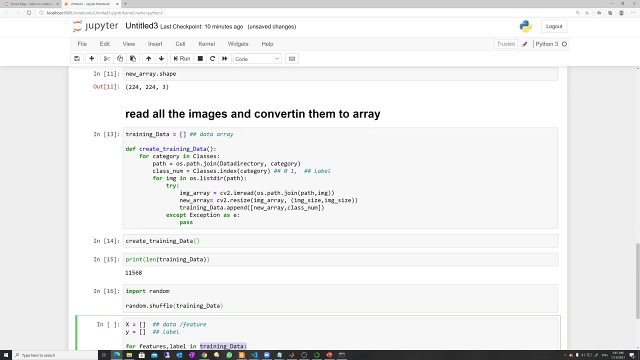 now that i have shuffled everything, let me create data and a label. right, data means the features, right, so i'm storing feature all of my features in the x and then storing y. so i have just got training data. okay, all filled and i have checked the training data. 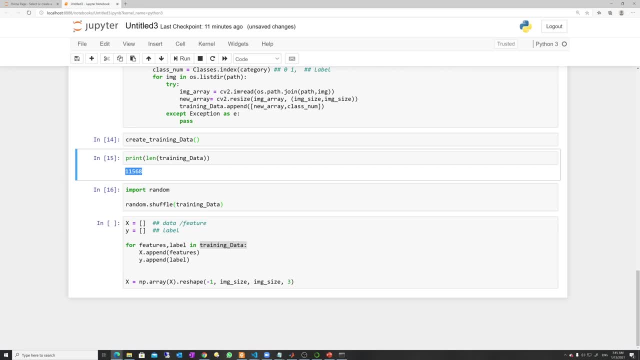 length that all of the images. i do have it, so i'm just reading every one and i'm just labeling it correspondingly, right? so the x- i will have the name because it goes some other way, even though it looks more- get known in the reverse way. 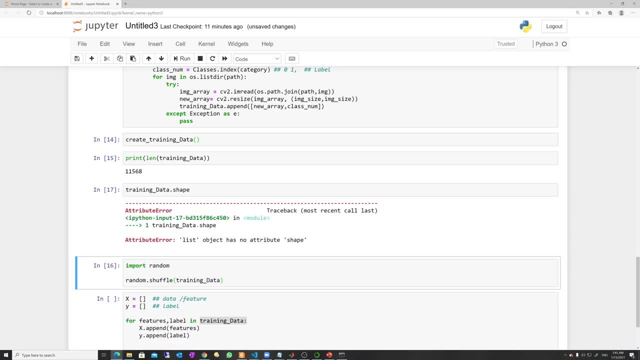 so the x is usually about problem demarcation, but it is treeton type of custom tree or tree and if i do that, normally it will build any type of tree that we want. i will have to change those values. i just want toü. can we check the? let me check the shape of it. 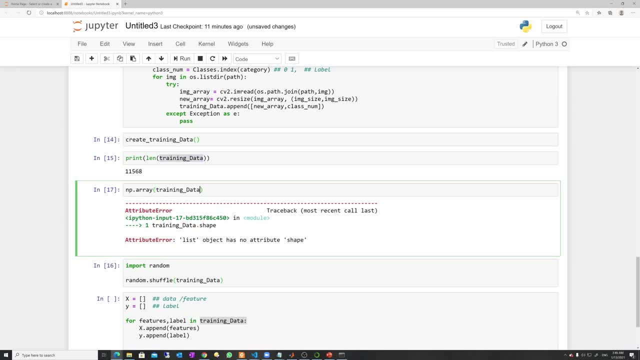 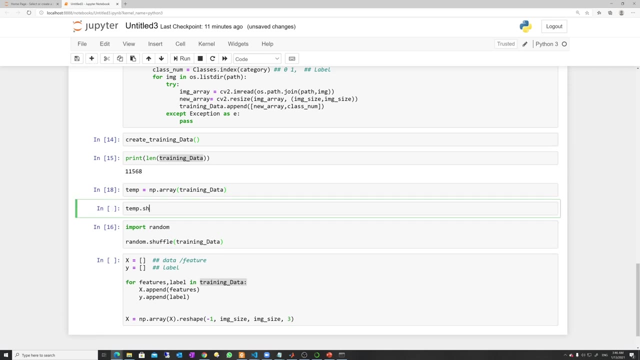 oh, it's a list, so okay for you guys and i can change temp. why i'm doing this step? because i didn't know you don't need to do it. i'm just doing it temporarily. so temp dot shape: because for list it cannot tell you the size, so that is why so. 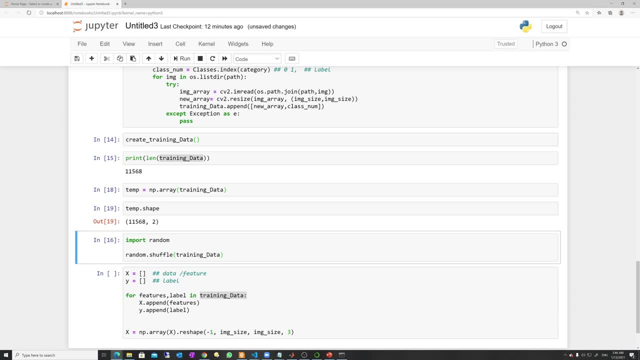 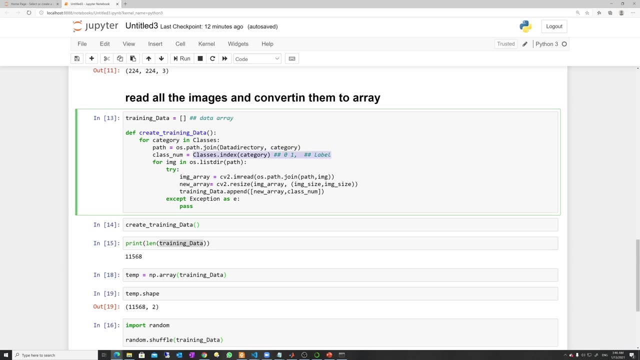 actually it has these rows and this much columns, so 48 into 48 they have just all images and everyone has two columns. so one is data and one is label. actually, so, over here, as i told you that my class name is actually my label, so while preparing this i have just store my class name. 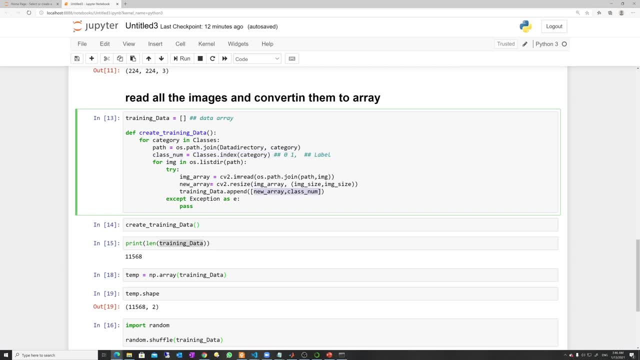 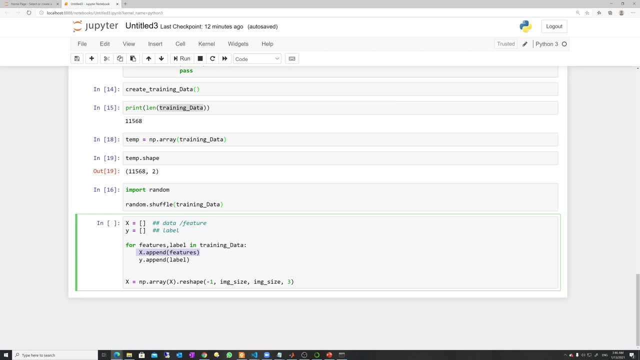 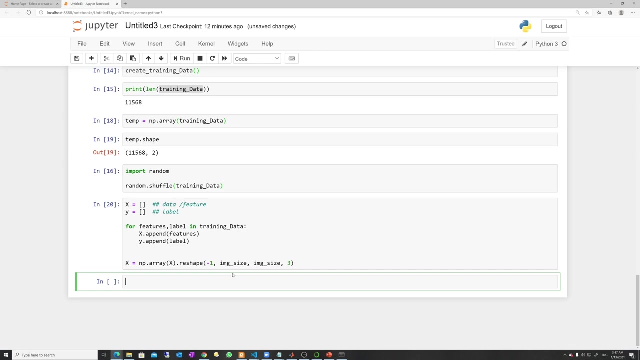 inside it. so one is one. two columns: one is my array, one is my class number. so that is why this one is my array, which contain images, and this one is label correspondingly, let me execute as i haven't executed. yeah, shift, enter over here. you can see like i am doing like this. so i'm just actually converting. 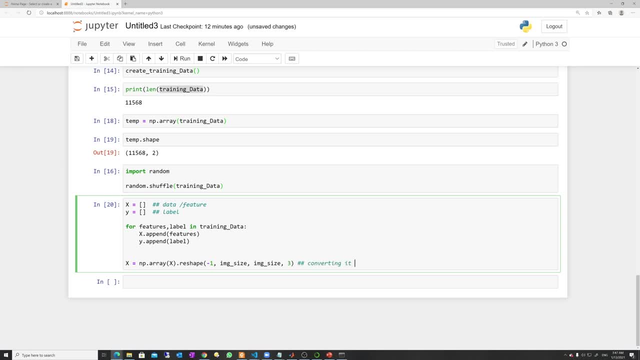 converting it to four dimensions. actually, for the mobile net, i will using deep learning architecture such as mobile net, which takes four because it can't contains depthwise convolution neural networks, so it takes four dimensions. so i'm just doing it minus one. minus one means the end, so i'm just putting one at the end. if i just check what is, 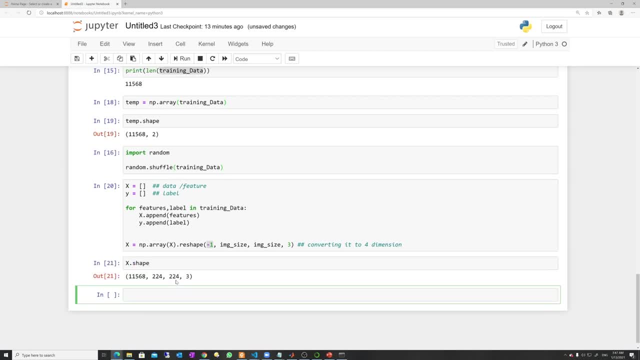 the shape you see over here. so all of my these, uh, these, this is the number of the files, and these are two to four into two to four. this is the image, and all of them have three channels. so this is my image and these are the number of the images. right? so, before applying deep learning, 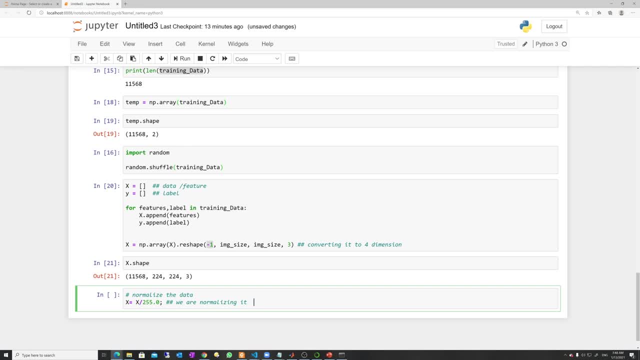 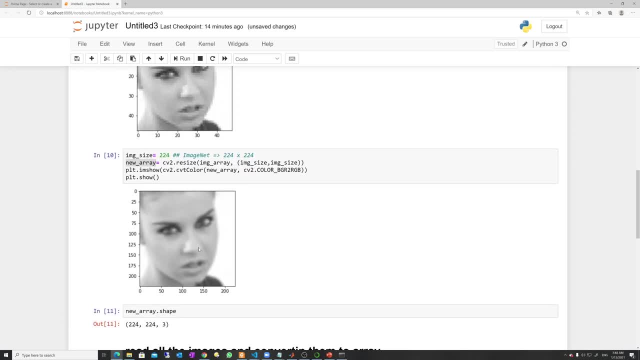 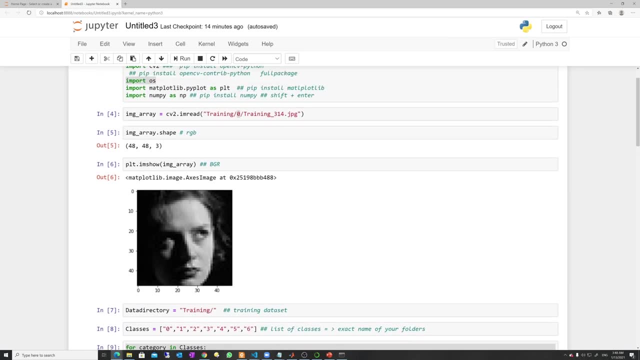 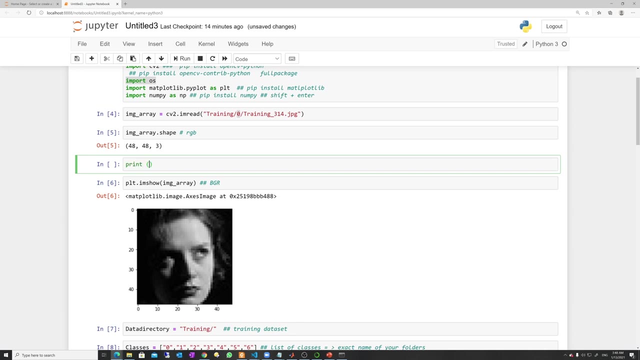 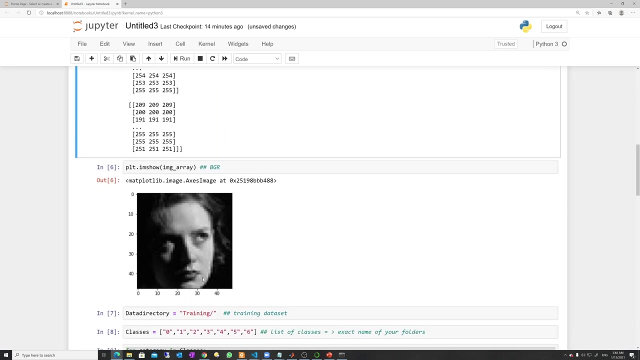 two, five, five. so over here you have seen. let me show you if you do have image. so this was the image away. so let me plot or print for example, then measure it, so you see all the values are like 2553, so the black means the black are 253, so black means 255, actually the maximum level to. 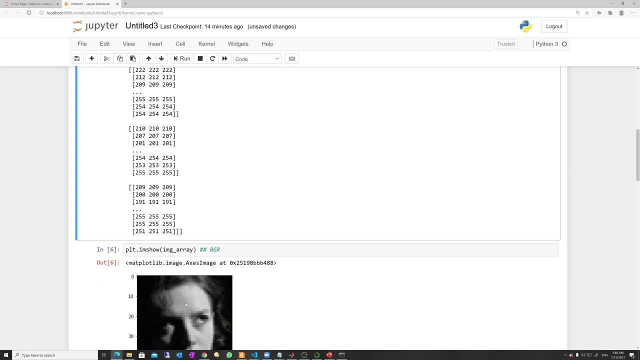 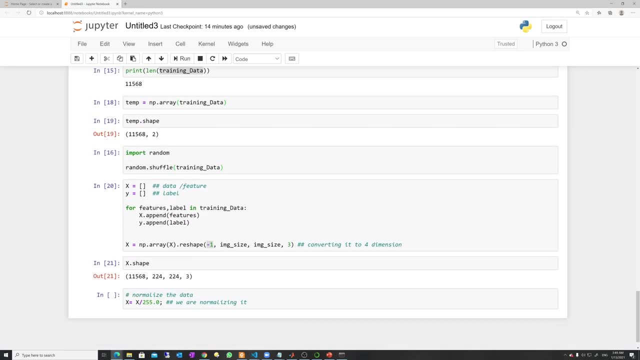 the black is 255 and the minimum level to the white is zero, so it's a gray level. actually the channels are gray level, so that is why i'm just dividing into 255. so the maximum 255 is black, so i will divide by the maximum number, so it will be normalized. so all then, it will be normalized. 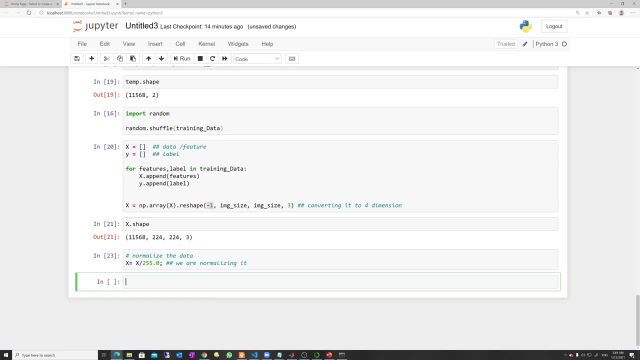 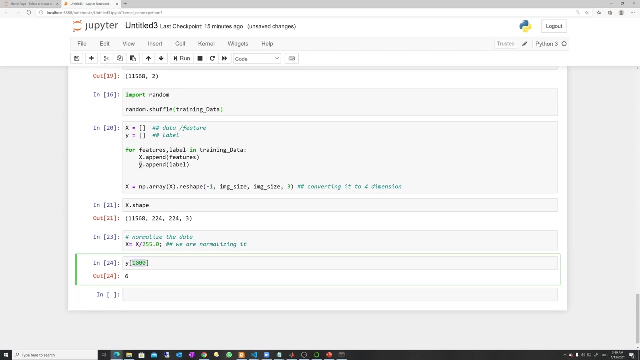 so it's. it's a very important before training. you should always normalize it. so let me check my y, like in this which i have append. for example, if i check the thousand, so it is six. if i check any other number like out, these are the same. let me check the shape first. ah, again, it's a list. i. 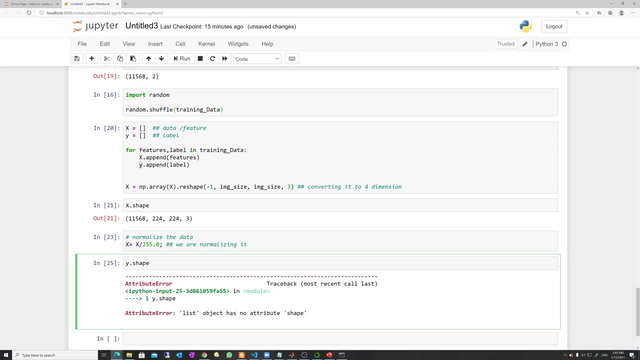 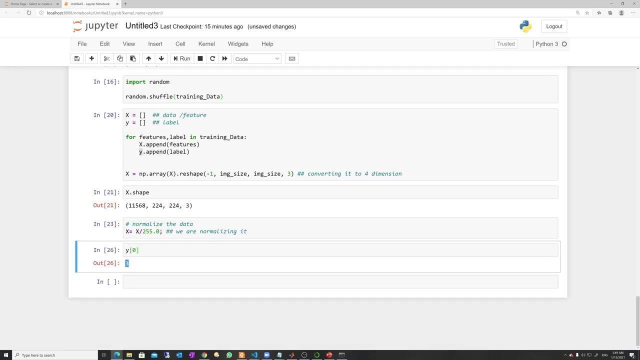 need to convert into numpy, but you don't need to actually all let me check it. so y, zero. so you see this, this is zero. so actually these are, these are labels as i have shuffled them. so now they have shuffled, and now zero means three, three means happy, i guess. right. so zero. one, two, three. so these are the numbers, right, so now. 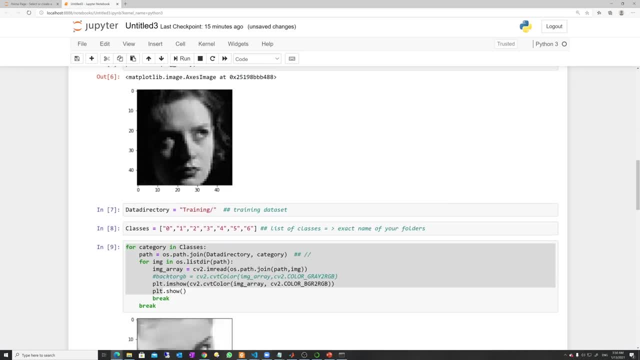 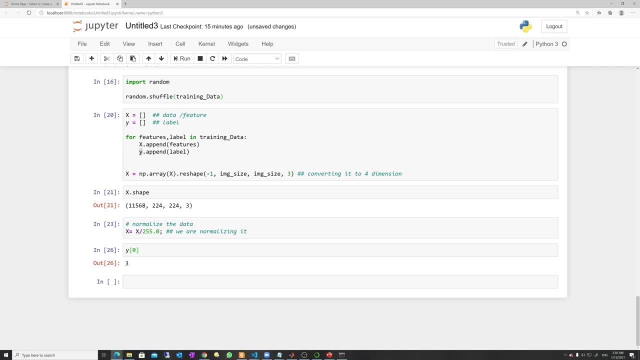 these are actually my labels. why? because i have converted them into the class numbers. so over here y is my label, so let me convert into array as i show you that these cannot be the list, as it don't work like if i do it like shape. so you see, over here it shows me list, so it is actually. 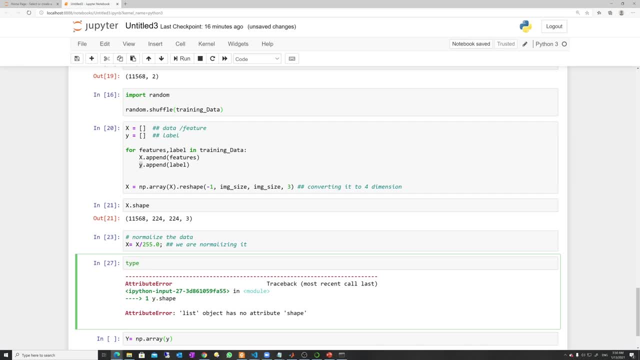 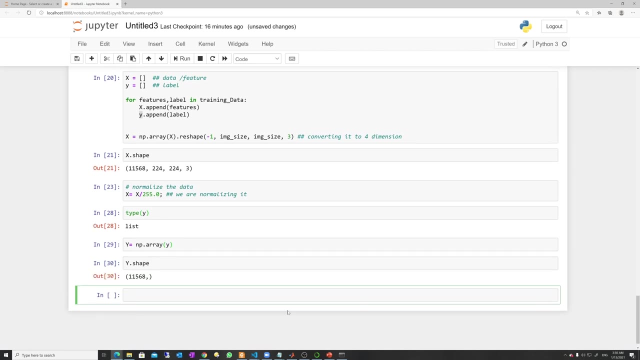 list. if i say type, why it will show me list, right. so these are the list. let me convert into numpy array. these are the command to convert into numpy array. now i can just check the shape right. so these are the shape. so actually 1d array, and then you see the shape of this must be same. so data and these. 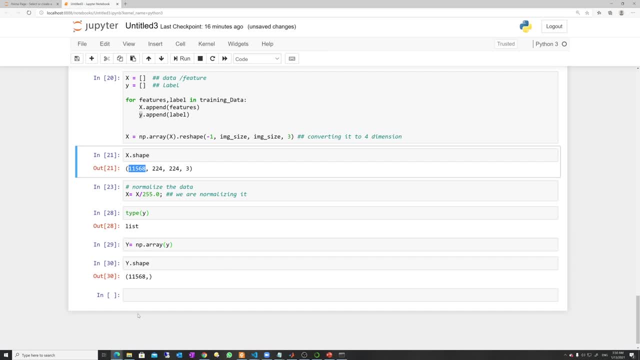 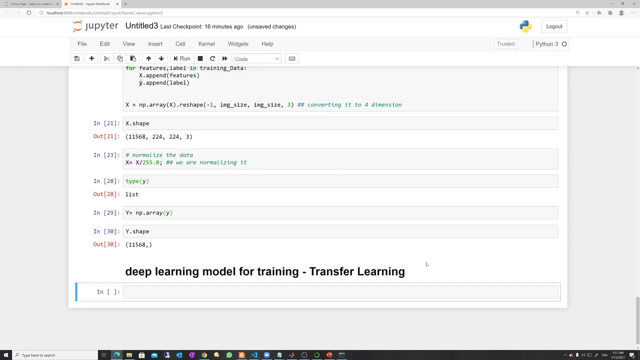 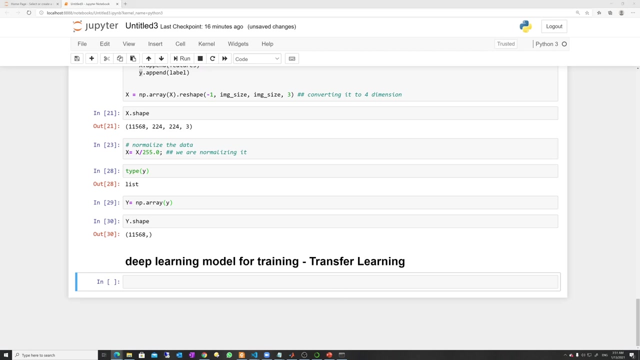 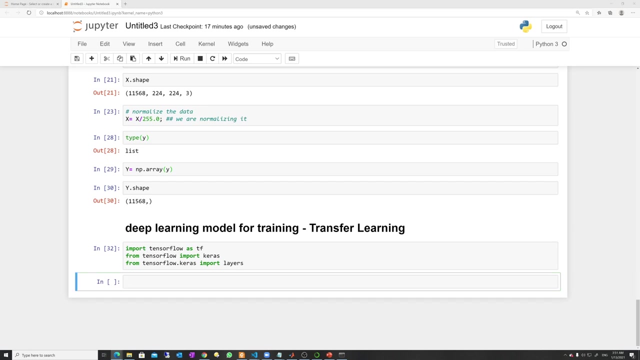 labels. now that i have defined my labels and my data, let's train our deep learning architecture. let's create a node deep learning model for training we are doing, going to do the transfer learning. i will just import tensorflow as tf and and the keras i'm done. okay, if i write model this on my variable name and if i say tf, talk keras, then 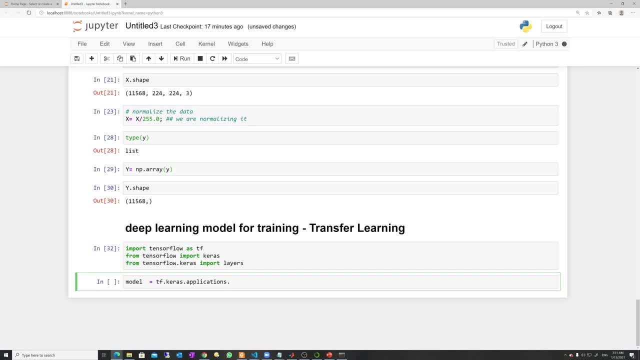 applications. if i press the tab, then if i press the tab i have a lot of options. so any of them I can take it and then i can perform the transfer learning. so what i'm going to do over here that i can, these are the weights, actually the trained weights, so on the thousand classes. so if i take any of them for 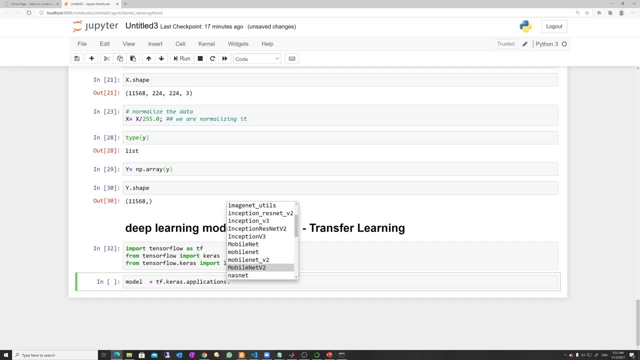 example. the latest one is mobile net version 2, although version 3 is also available, but as my tensorflow version is 2.1.0, so in that case it's only version 2.. if you install the latest version, you will find version 3 as well. for now, i will just take version 2.. so what is this? this is actually. 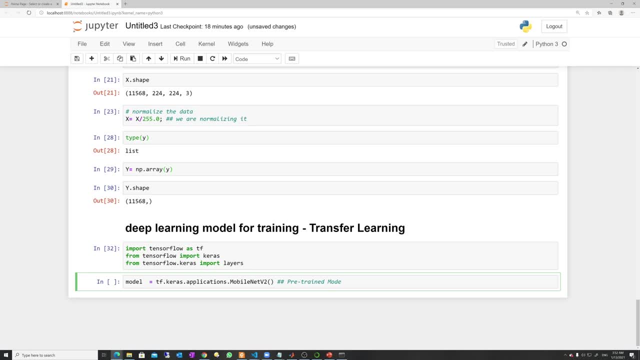 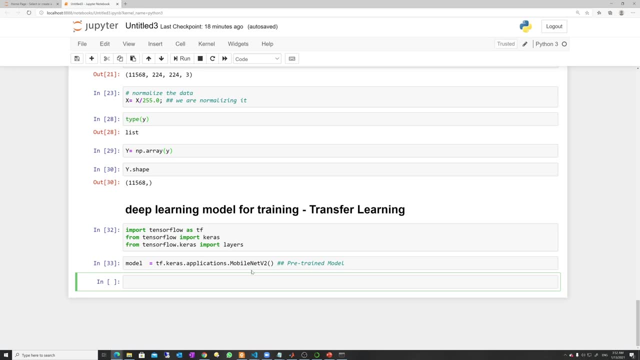 free trained model right. let me execute. so now this: in your case it might download the model right. so in my case it was already downloaded. that's why it didn't take a lot of time. well, in in your case, if you're doing it for the first time, it will start downloading. so make sure your internet. 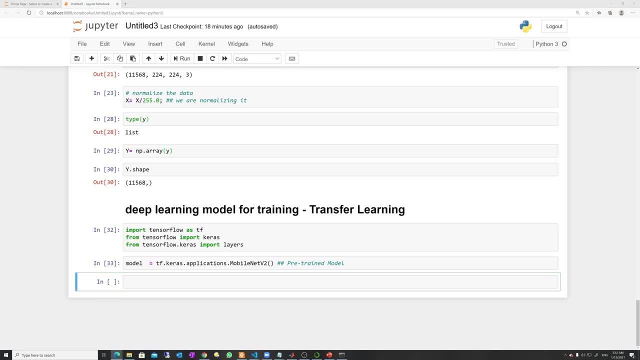 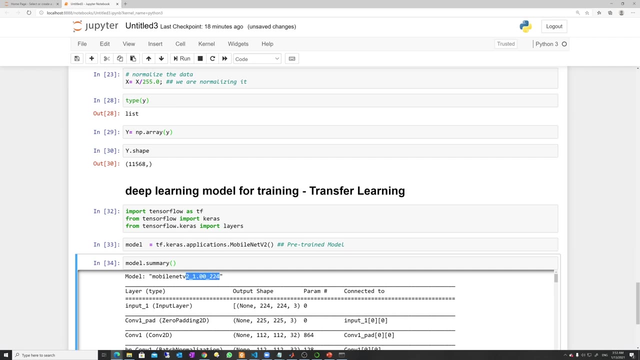 internet connection is up so let me check the model summary. what's in inside it? like this: this is the model summary. so actually you see, the model number is two to four because they were trained on. these are the name of the model it is trained on: two to four. that. 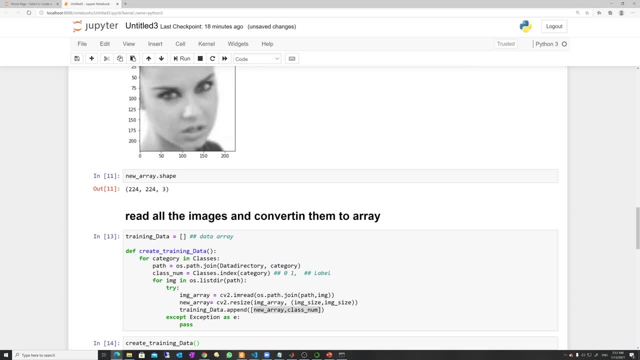 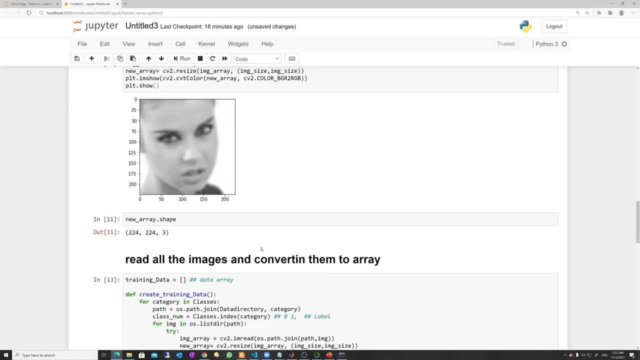 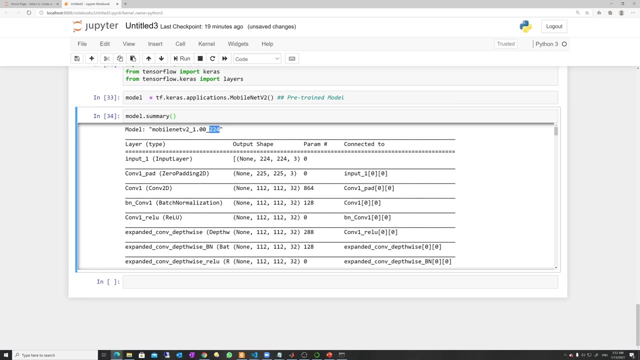 that was the reason why i changed all of the size into two to four. before it was 48 into 48. you see, it was 48 and 48, but i changed everything into two to four. why? because mobile net, except two to four into two to four. you see, so now i can judge like it takes the input two to four, two to four. 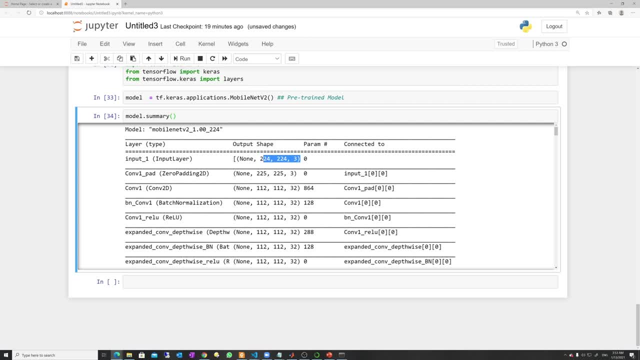 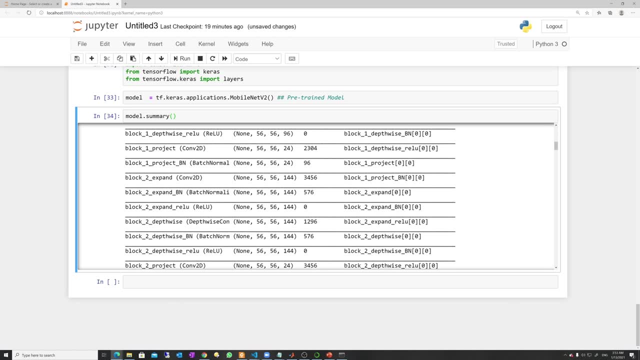 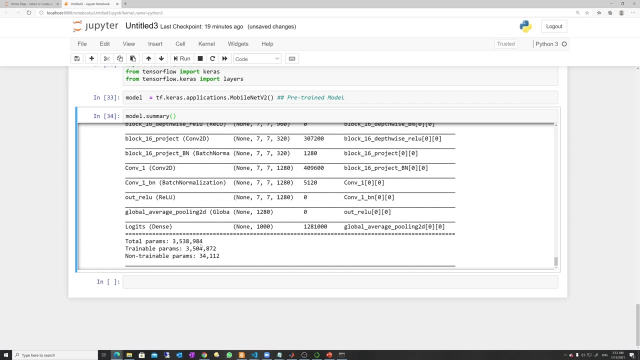 into three. it takes rgb image. if if it was gray, then i have to convert into rgb. it has a lot of layers. it's a huge architecture. mobile net version 2 very accurate. it has almost 3.5 million training parameters- right, so it has a lot of training parameters. 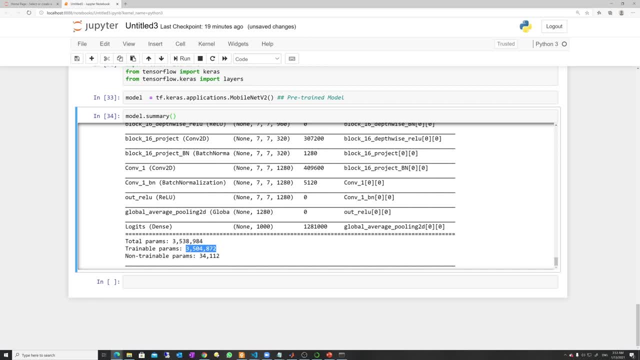 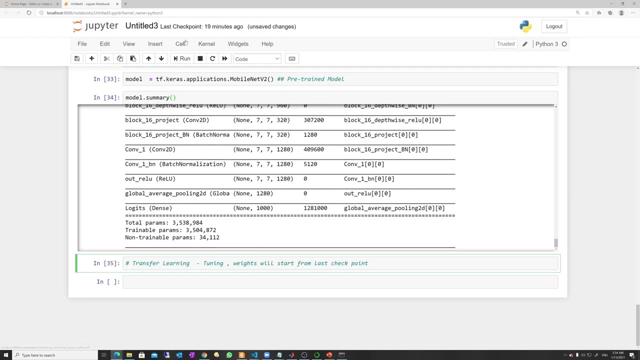 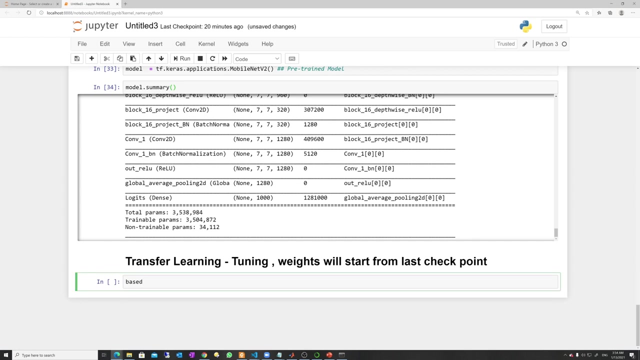 what i can do over here that it was trained for the thousand classes, right, what i can do is let's perform the transfer learning. let me convert into the okay transfer learning. uh, let's do the transfer learning. so the first part is that let me change. check the base input. so what could be my base input is that model dot, if i say layers, because 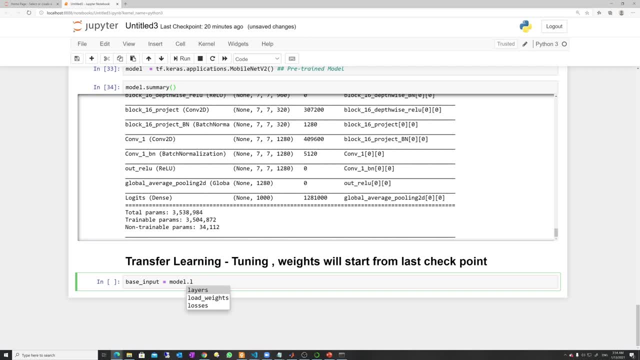 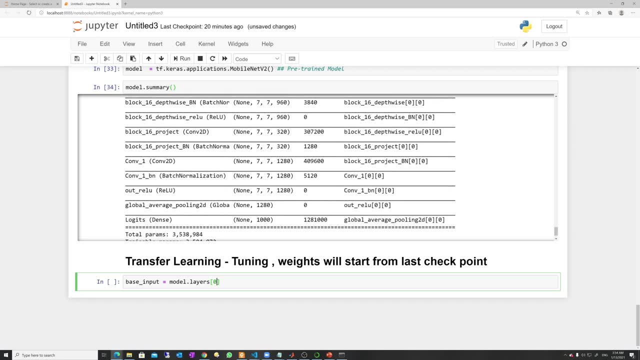 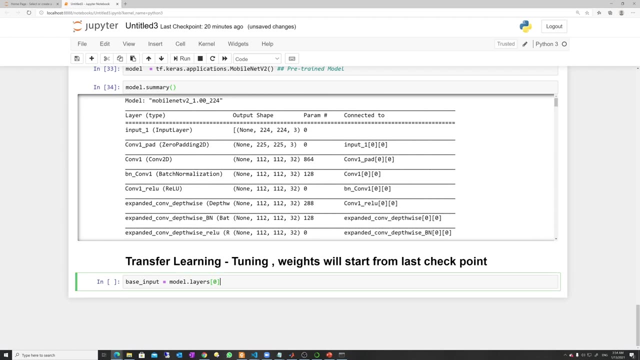 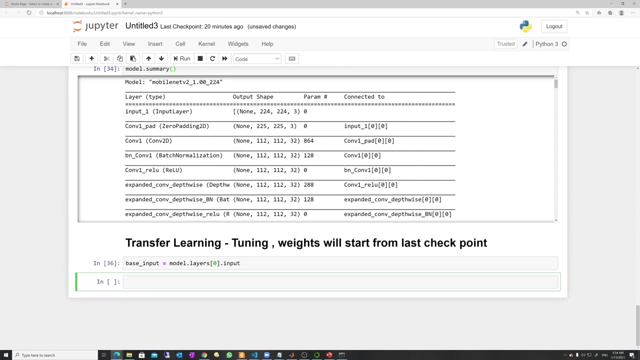 i have already downloaded the model. so when i say model dot layers, if i want to check the zero, zero mean the first, okay, and zero the first layer- okay. i'm just taking the first layer dot, so let me be cured, okay. now i want to check the base output. this is again my variable and i will check from the model. 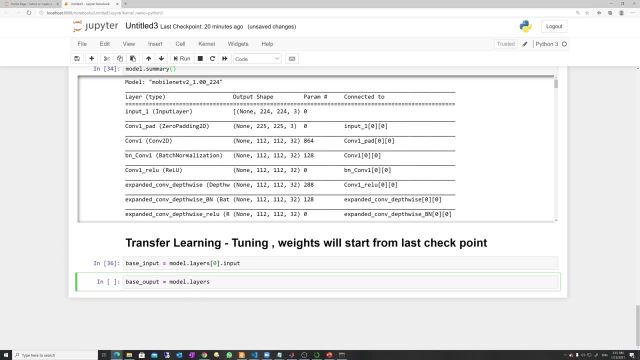 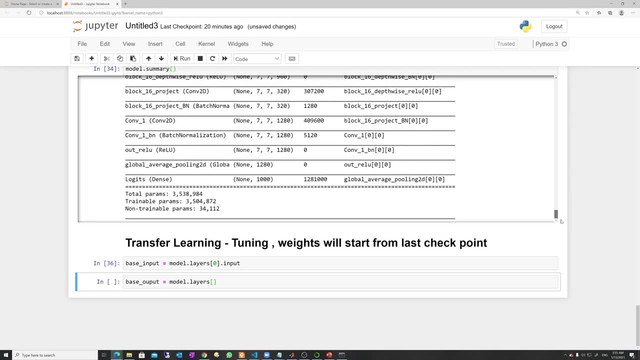 dot layers if i press the tab. and now this time, so this time i'm i would just want to have. so this is minus one right. always in the python, the last layer is minus one right. all i need is to just cut it down, because i want the seven classes, not the thousand classes, so i will just 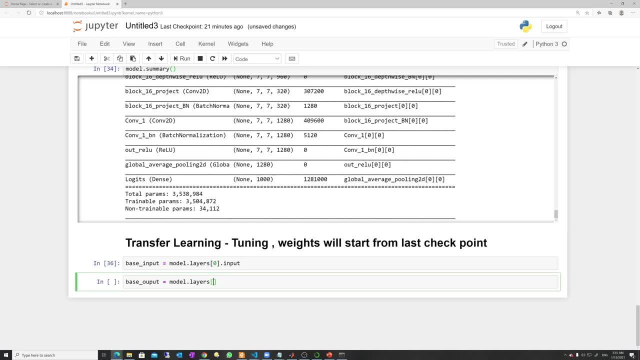 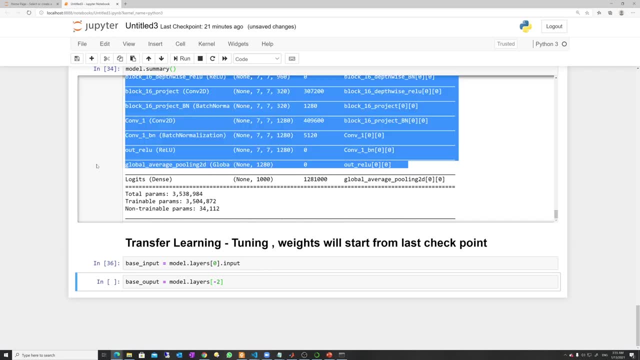 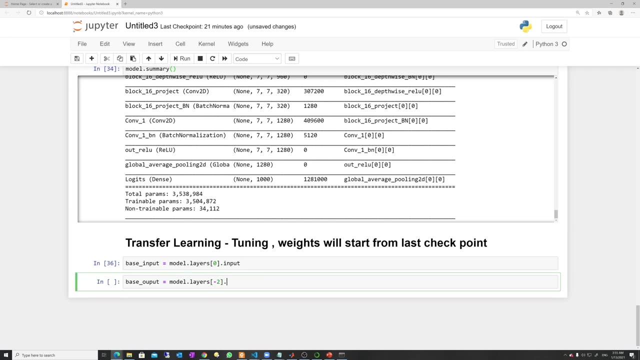 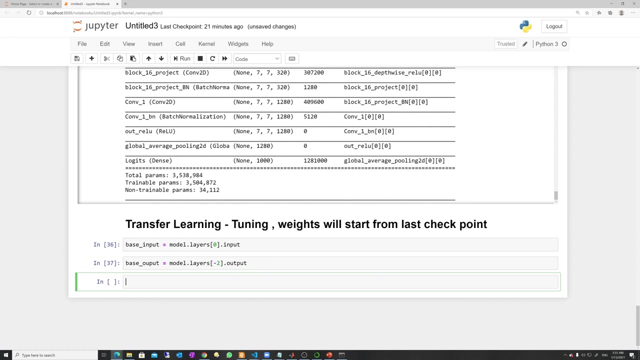 convert into seven. all i need is to just minus two. okay, so this is minus one and i want only this one. so this is minus two. right, this is minus two. so i will just cut this one. i will ignore the minus one output because i need the output of the base output. okay, if i just pull, just show what's. 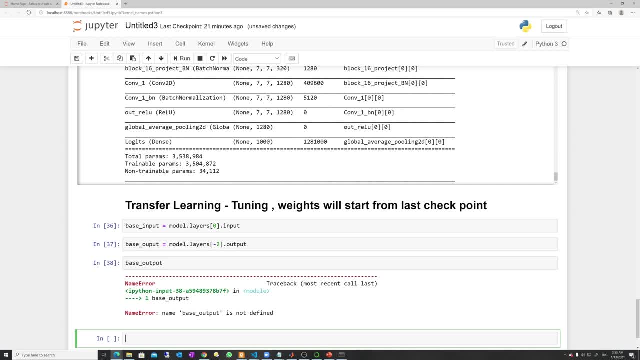 what is inside the base output. let's not show something. it must show that. okay, we, we can verify later. it's okay, okay, so soon we will verify. okay, let me do it like this, because i should must have like this, and then base output should be tensor. okay, anyways. 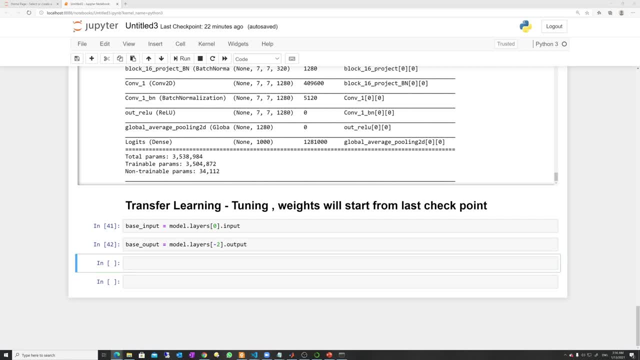 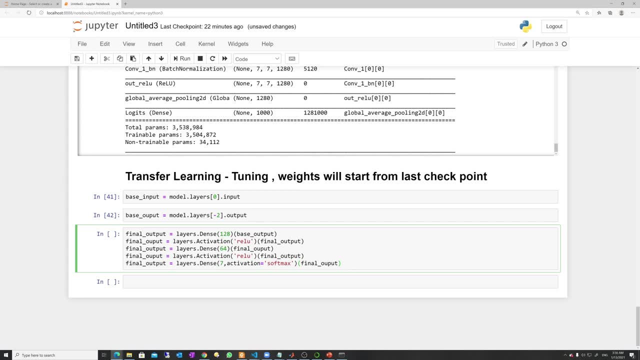 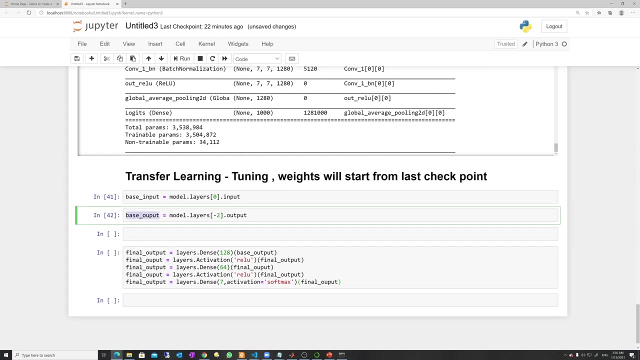 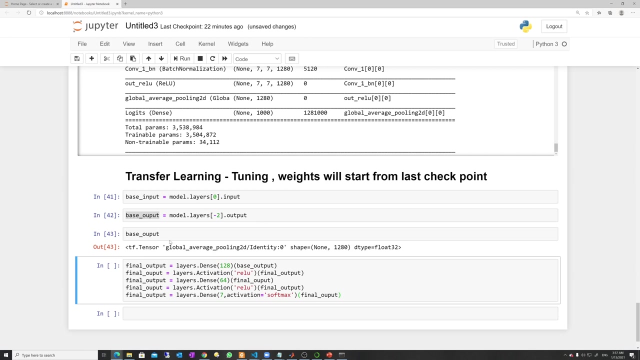 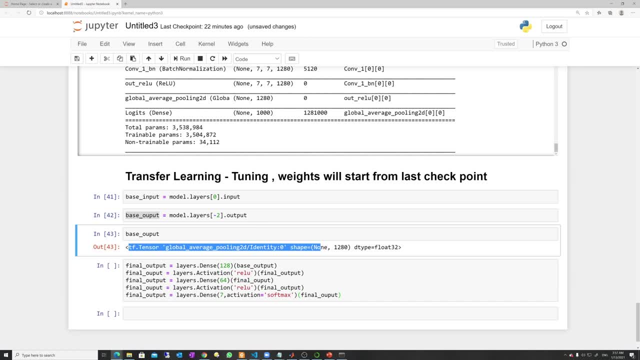 so base output is tf dot like this. right, so it must be. base output must be like this. so now, okay, it was changed. actually, i was just copying from my, from my notes, so that is why maybe the name is different. ah, that is why. that is why, sorry. 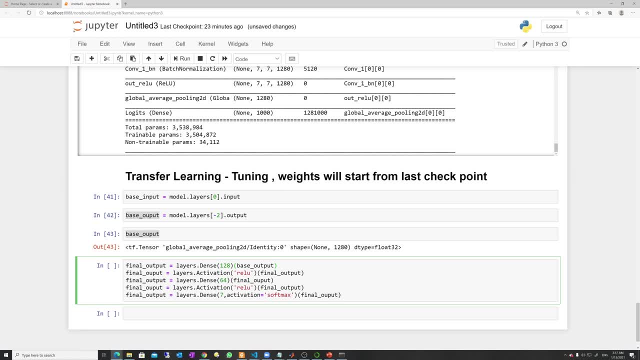 the name was different. that that's happened when you were just doing it live, right, so this is basically let me do it output, so it's better to change the name. oh yeah, the spelling was wrong. so After the output. after the output of global pooling layer: right, so this was my global. 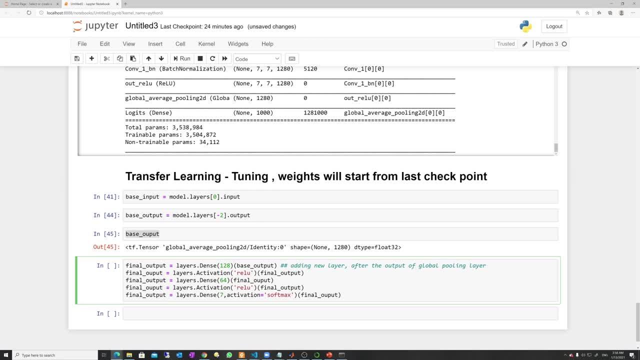 pooling layer. so after that i'm just adding it, what i'm doing over here, then this output: i'm just applying layers: dot, activation array, loop, activation function, function. this is my comments. and then after the activation function: okay, i am just adding 64. so now i'm doing it 120, 128 and 64 and then 7. right, why this? 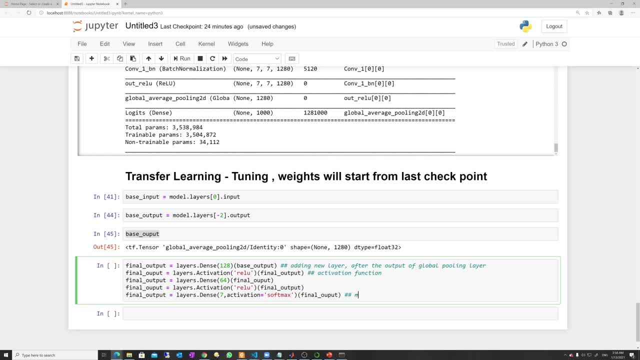 is 7 because my- my classes are 7. previously it was 1000, right, so now i'm just i just cut this and then i have added these three layers. so stepwise i am going. previously it was just trained, so that is why it was easy to have one fully connected layer. but for my class 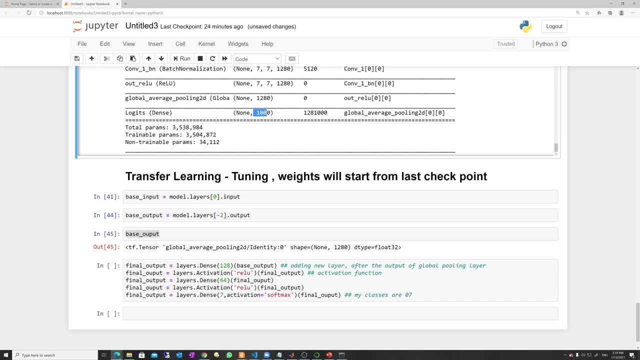 before. i have added this three layers. so if i have added this three layers, then it is going to be one layer and that's why it was easy to have one fully connected layer for case. I checked multiple times before making this demo so it's better you can. 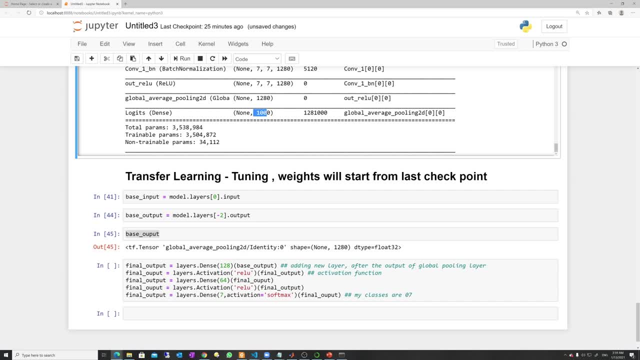 try many other settings as well, but this is one of the combination, okay, so now I can execute. okay, base input. I hope I have written the same, okay, so what I did so far is I have connected this into this. now I have this is my input, okay. 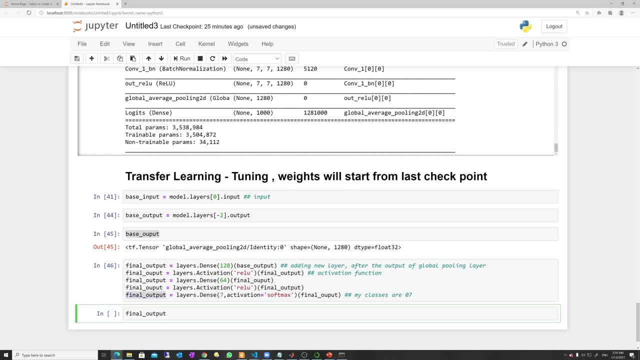 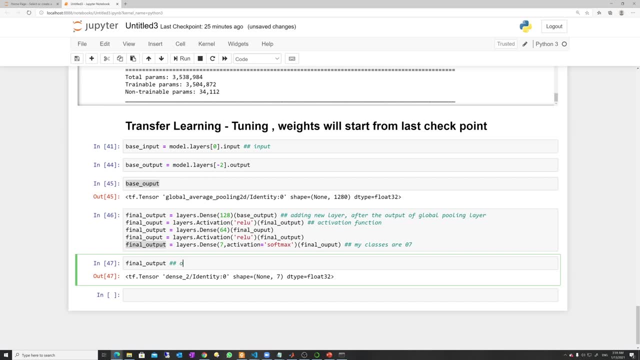 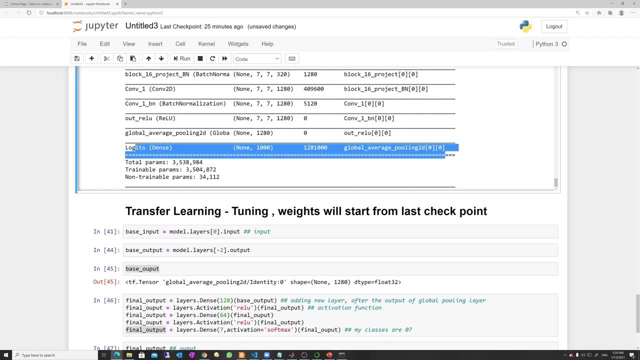 and what is my output? this is basically my. yeah, you see, so this is tensor of the salmon. so this is my output. what I did so far, I have added: after this, I have removed this and after this layer, I have added these layers, and then I have added: 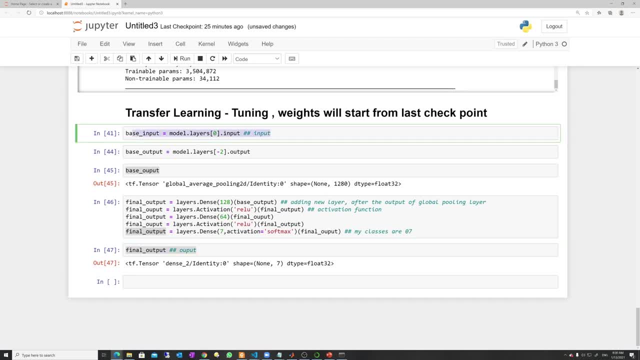 how could? this is my output and this is my input so far, but I haven't created a model yet. let me create a model. so my inputs are base input, which is this one: okay, these are my input and my final output is my output. then let me create a model- new model. now that my new 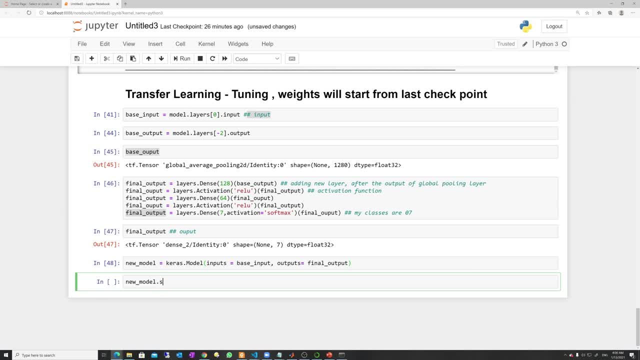 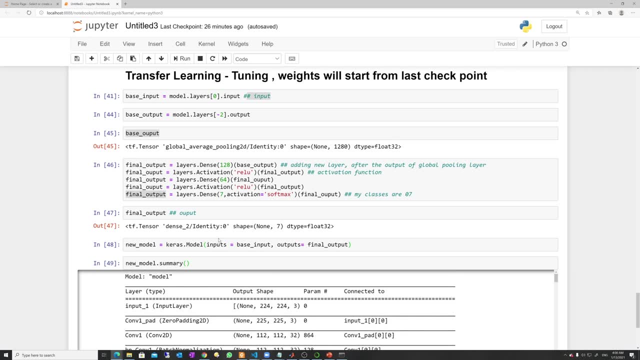 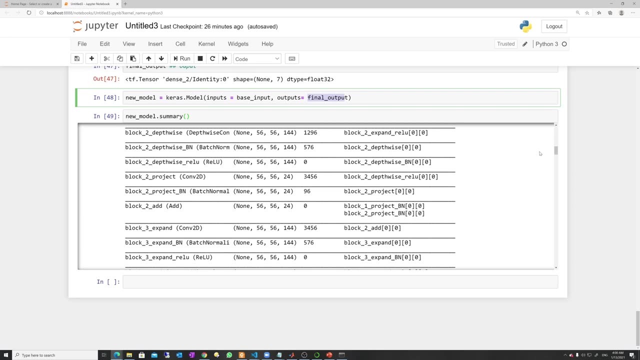 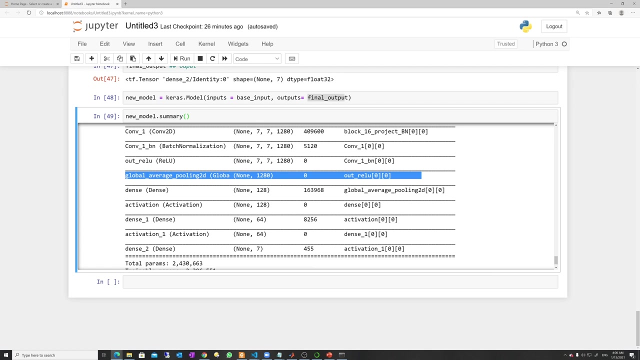 model is created. okay, let's see almost same right. why? because my input was this same and my output was final output, not this one. so what it did is, you see, after the global layer, it has created this 128, 64 and 7. these are the. 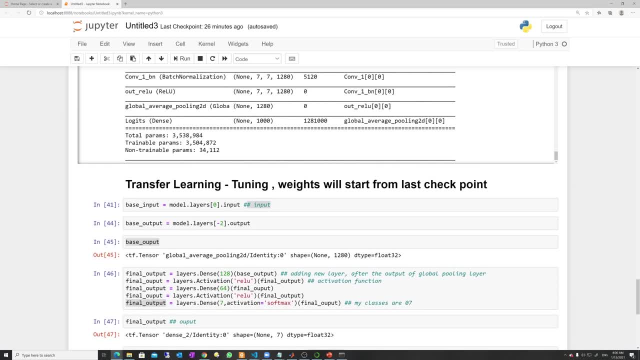 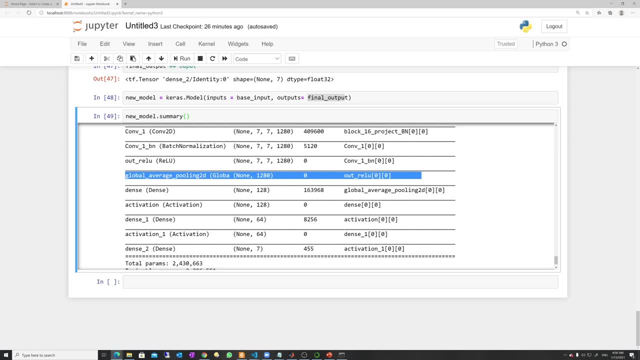 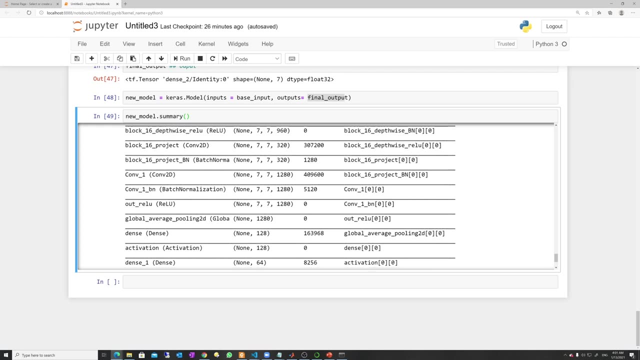 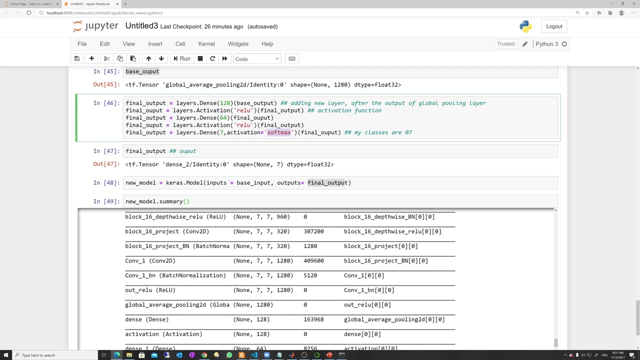 activation function. you see, you just cut, cut down this and then you just add it two more layers of three, particularly three dense layers, which is also called as fully connected layers, and we stepwise go for the seven and make sure. last fully connected layer: activation function: softmax. while previously there was a redo- okay, because this is my- 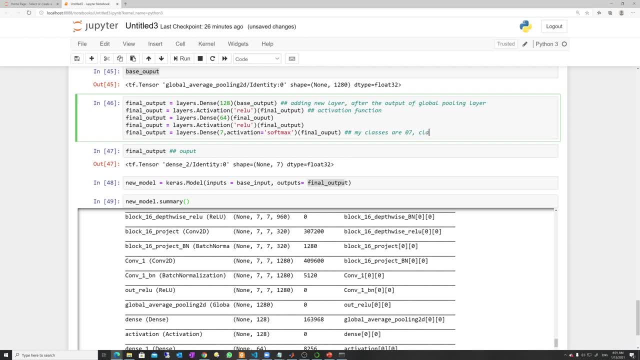 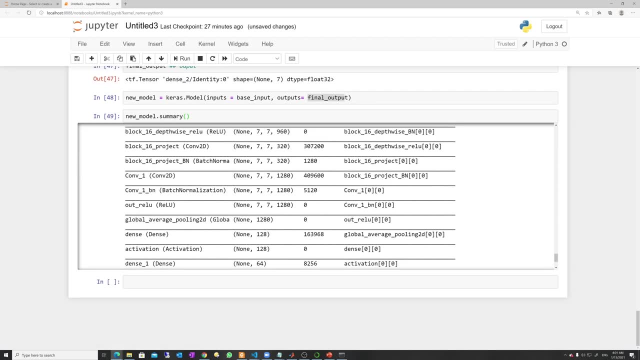 classification there. so this is my classification layer, but that is why I just did it: softmax. I can use others as well, but usually softmax is the most famous one. okay, so now that I have created a model, let me set like. let me create a model of like, let me compile. so these are my last sparse, categorical cross entropy. basically, what i did is: 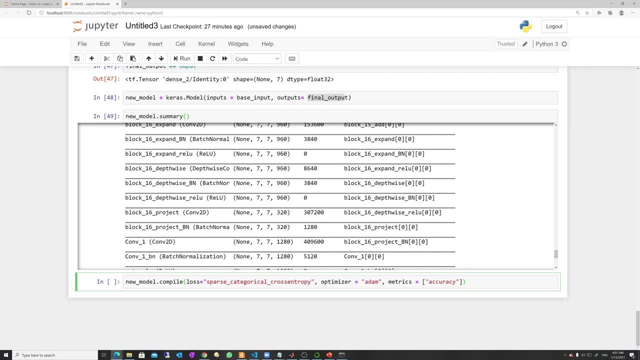 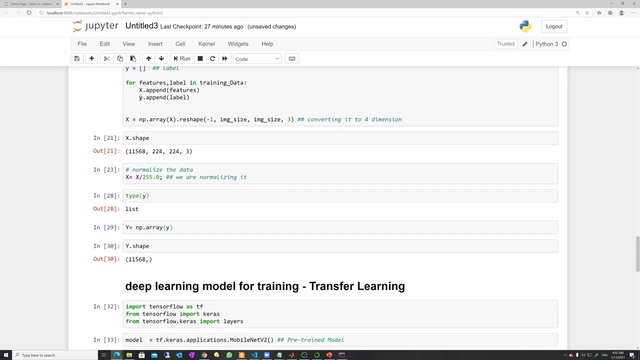 my labels are 0, 1, 2, 3 in the numbers right, not in our one hot encoding. so that is why i'm i've just set sparse, categorical cross entropy. so if your base, if your labels like this one, my label, where is it okay? 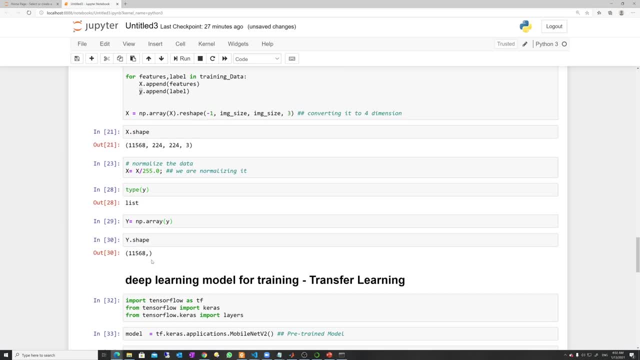 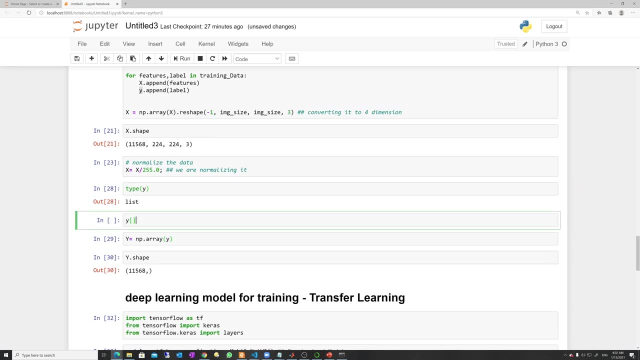 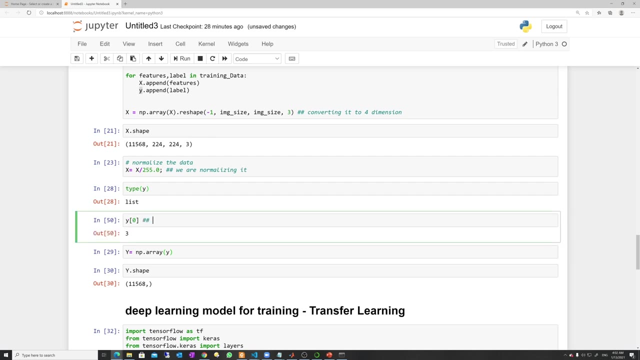 these are my. why is my label right? well, let me check again. let me show you. let me show you again why. here's my zero. you see, my labels are in the numbers, not in one hot encoding. one hot encoding is means that if it is three, then it should show like: 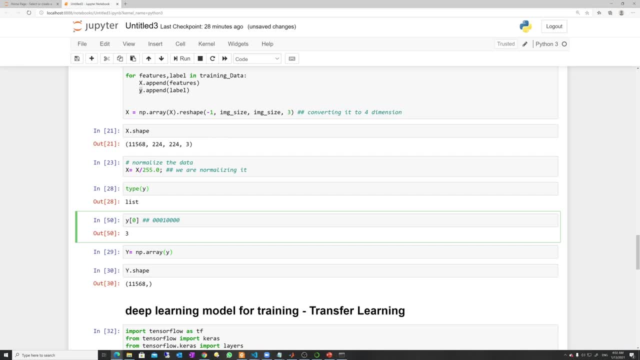 zero, zero, like this. okay, 100 encoding is like this: sorry. for example, this is: well, i'm not hot encoding, so that means that i'm not hot encoding, so that means that i'm not one. this is, for example, zero. this is two right, similarly. so one on, in what heart? one heart. 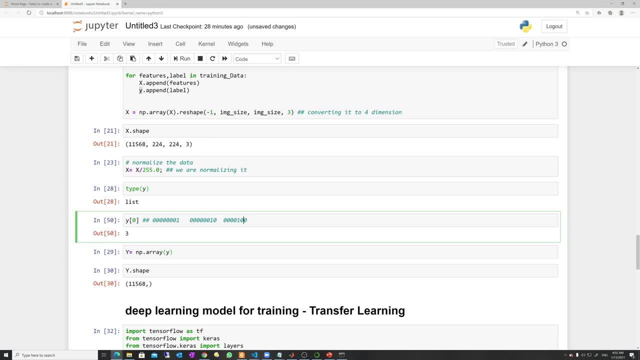 encoding is that, like we shift one towards the position, so position shows, all of these are one heart encoding. but in my case it's not one heart encoding, right, so one encoding is means like this, particular I. so wherever is my class, I will just say the one. so this is another class. 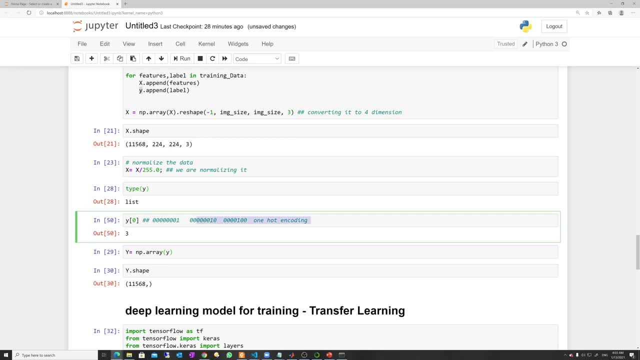 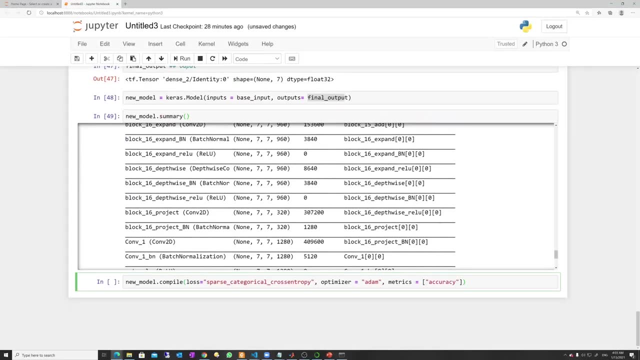 this is another, like we do have different labels, so in my case it's not one hot encoding. okay, now that we have defined everything, let me compile because this loss- I told you why I chose similar to optimize that you can choose anyone, Adam and at a grade, and a lot of them, and my matrix is: 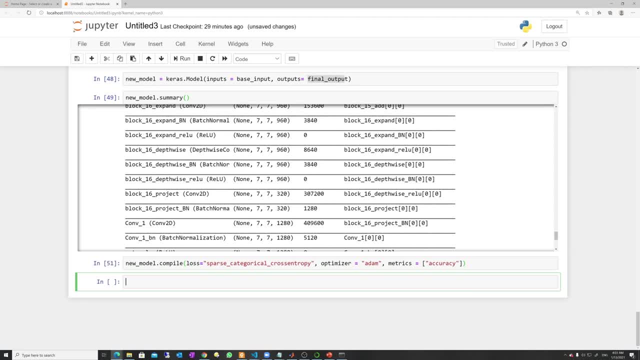 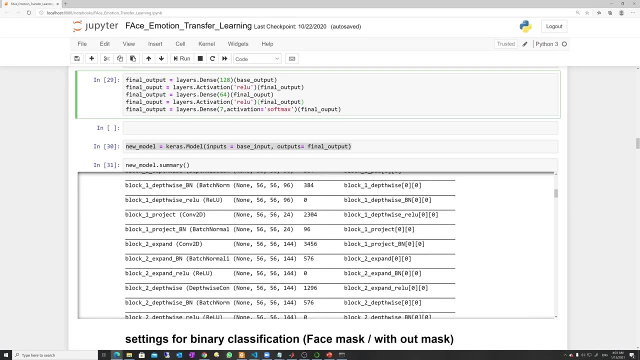 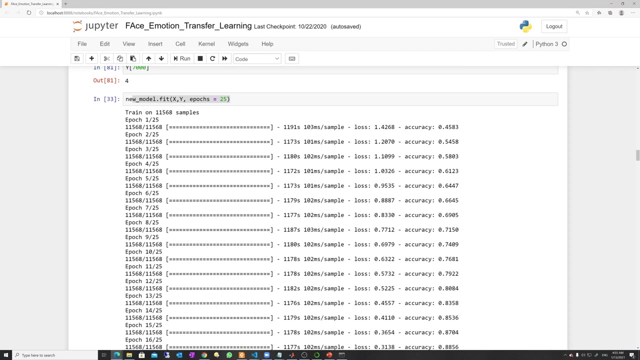 accuracy. now that I have compiled, I okay. so actually in the live demo I will not just do it, let me show you my notes. so over here I have actually sorry. I have already trained it right using 25 a box, so in live it is very difficult. 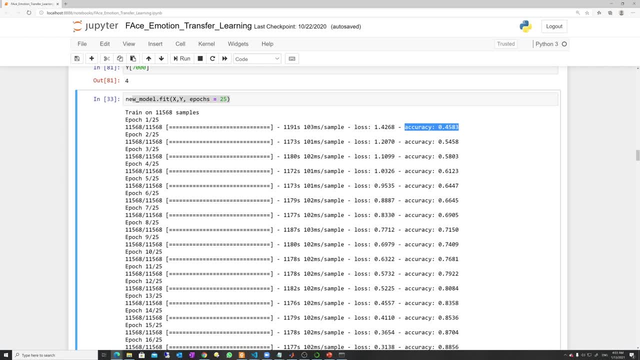 so you see it just started forty five percent. why? because it was already already trained. and you see it just started 45 percent. why? because it was already already trained. and you see it just, the classification problem was really similar, so it tuned the weights accordingly. so in the first 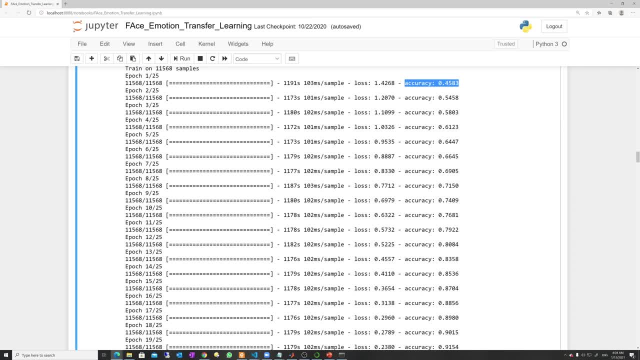 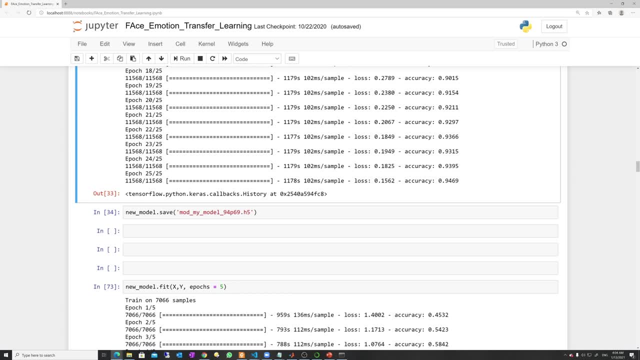 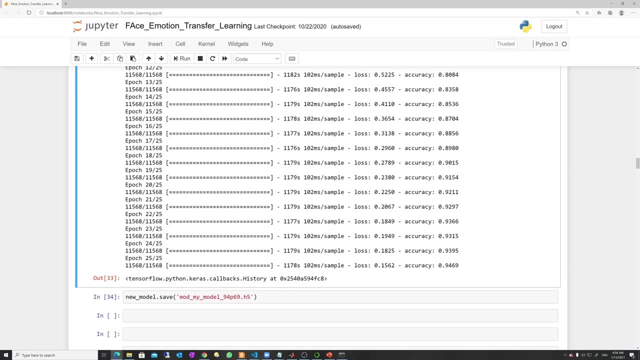 but if we i do not use, if i create my own deep learning architecture, then definitely it will start from zero or two percent. right why? because then it is not transfer learning, it's not getting the trained weight, so we are using the trained weight and then, once you train, you can just save. 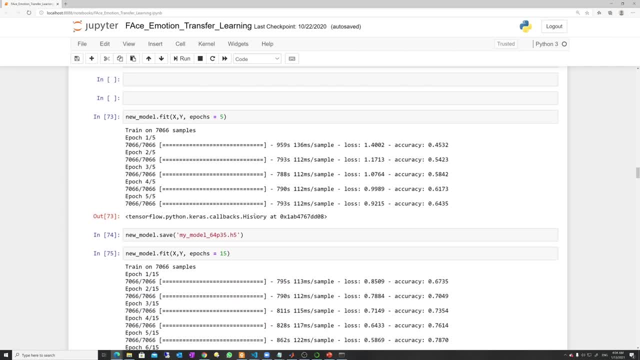 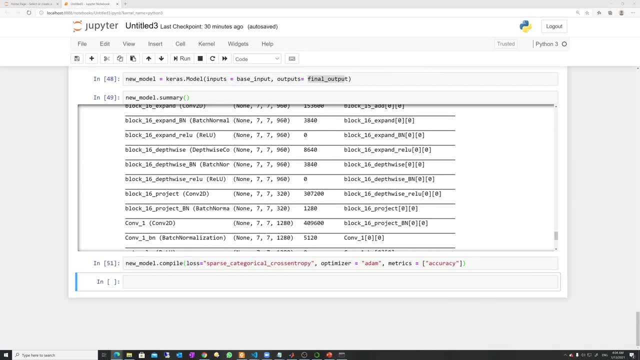 your model and then i have just run different epochs. i'm just showing you how i did right. so once i show you what, how i did, i hope i have. so far i have trained right, i believe, but i have to train in the live so i don't want to train over here. let me load a particular model, so i have. 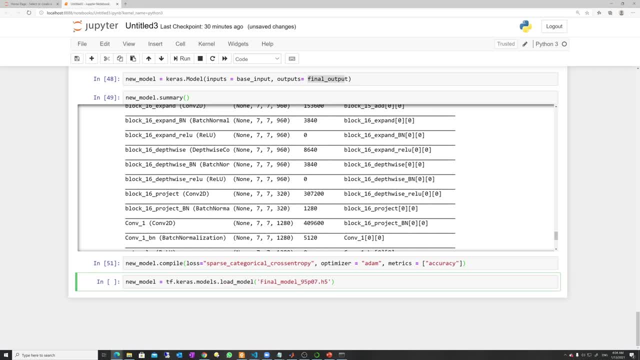 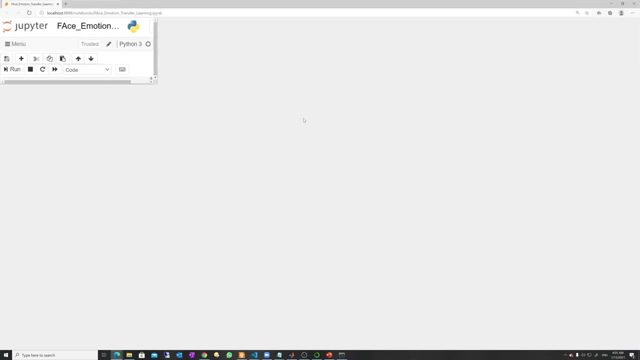 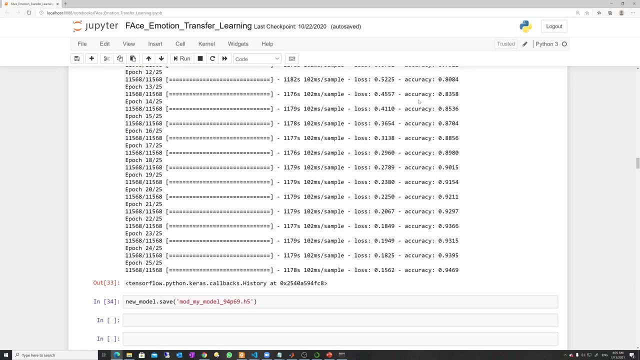 already trained. so, if you want to, when you press the compile, all you need is to just, for example, just fit. when you press this, fit as i show you that it will be like this: right, sorry, it comes through. yeah, so you can just run like this. you see, everyone is starting from 45, but i was actually trying different. 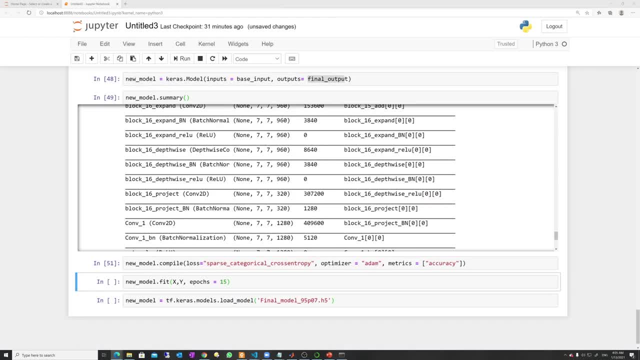 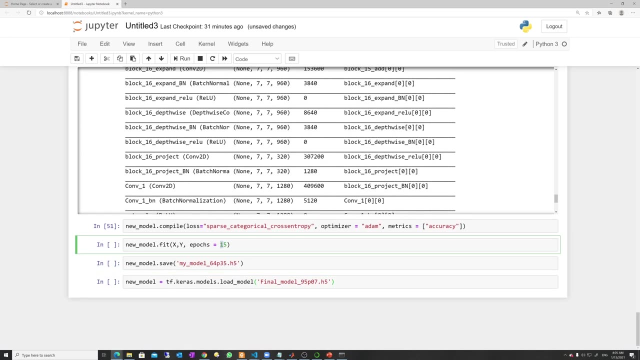 combinations. so i believe that i have trained everything and then, after training, what you need to do is just save your model. so i'm just copy pasting the steps. i'm not running them, i'm just copying pasting. so, based on your epochs, you can have less epochs on. it depends upon your training, right? so 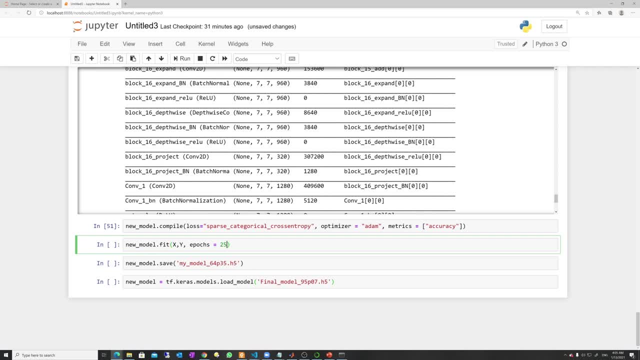 if the accuracy is not good, just increase the epochs. so i i'm just just not running these two guys. but these are the final steps. after compilation, you need to fit and then save the model once you click the save button, because it's what you need to do now. so the next step is to load it. so 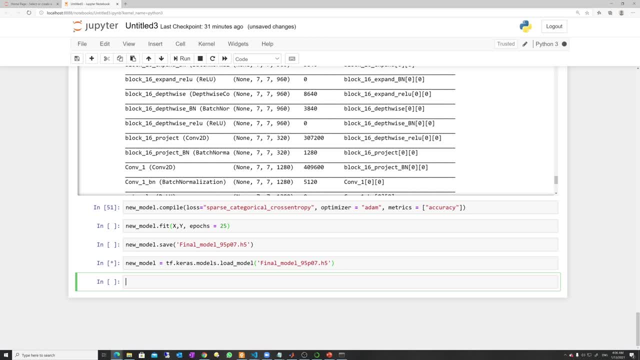 you can see that i have already created a new model, so i'm just loading my model and i'm just loading my pre-trained network, and i don't know why i'm loading it because the name should be technically, the name should be, for example, same. so, for example, you have saved this and now i need. 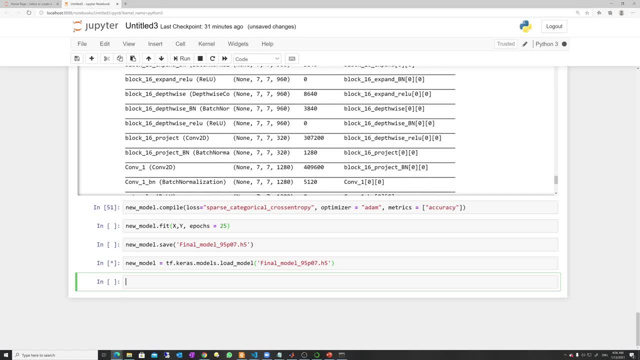 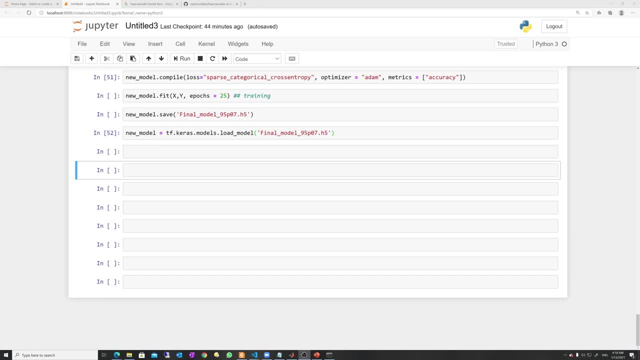 to load. so i'm just loading my model, so i have already trained. so, in order to save my time, i'm just loading my pre-trained network, our model, and i believe that you have already trained the model- and then save. and if you do not get a good accuracy then you increase the epochs. so now that i have already loaded the 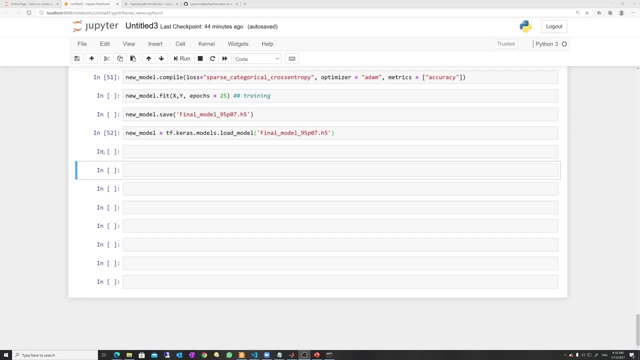 new model. okay, that i have already pre-trained. so in this variable i have my model. now i can test using new model, dot evaluate. but actually at i don't need the accuracy, right, so it's for accuracy purposes. so actually i don't need my test accuracy. in this case i can have my, i can use my test data. 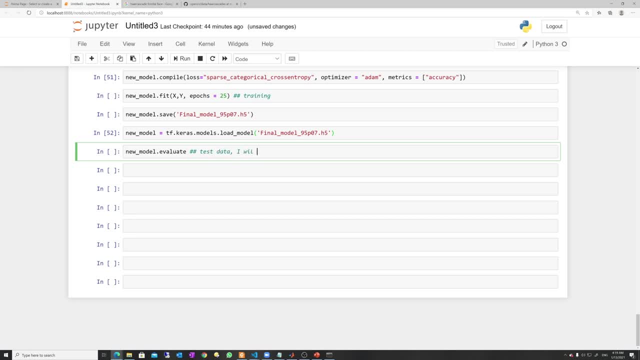 sign, but i will not use my test data sign for accuracy. rather, i will deploy a live image demo right. so that is why i do not want to evaluate my testing accuracy. i'm not interested in my testing accuracy actually, so i can just deploy on google images what i can do. 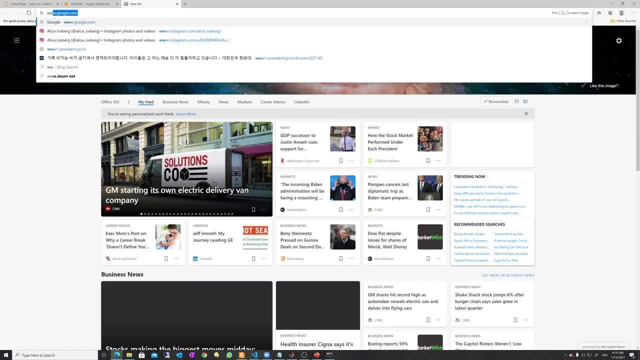 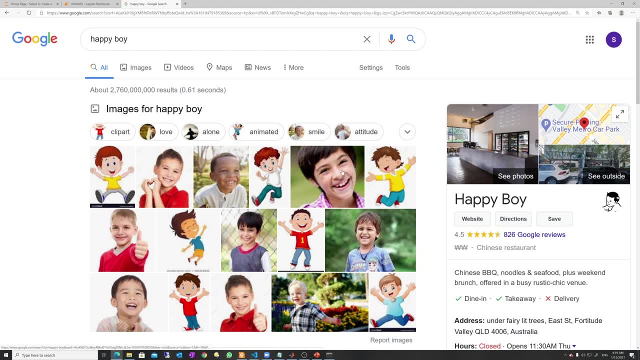 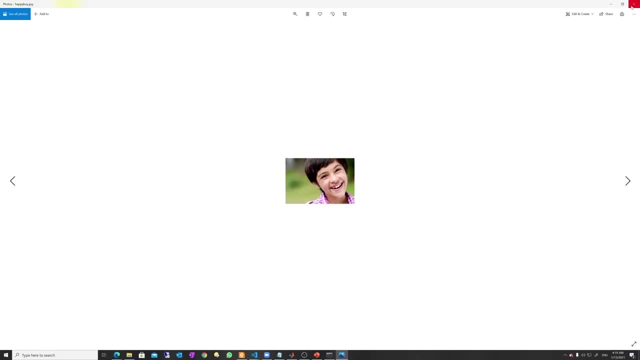 is just google. uh, google is the happy image, for example, any happy random boy. so this is the happy boy i can just download. so i have already downloaded this happy boy image. let me show you. this is a happy boy image, and this happy boy image is in jpg format. 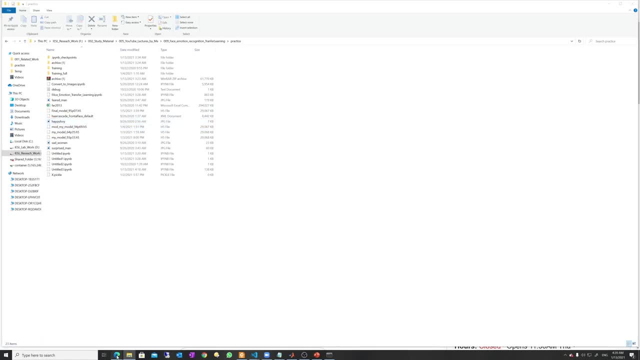 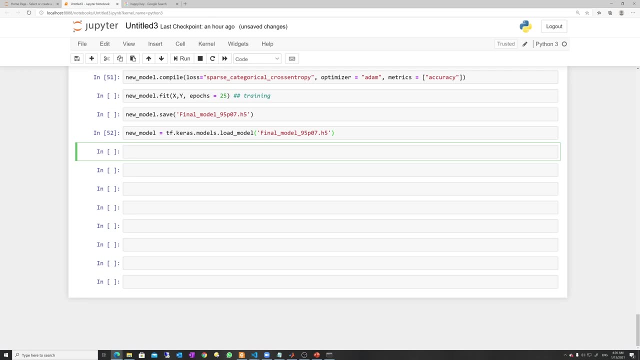 so i can just copy the name and let me just write that, such as- let me name it- frame is equal to c to dot. i'm read sorry, and then i can just paste the name as it was jpg. okay, so let me load this image as it successfully run. 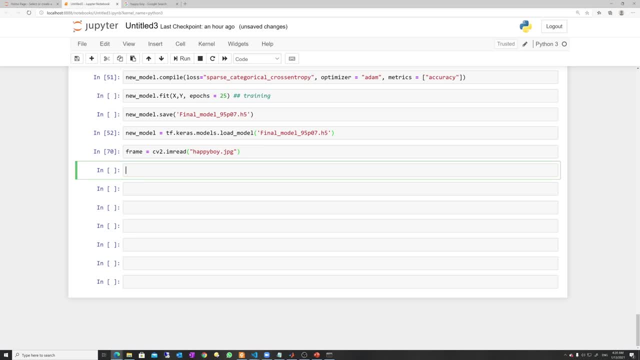 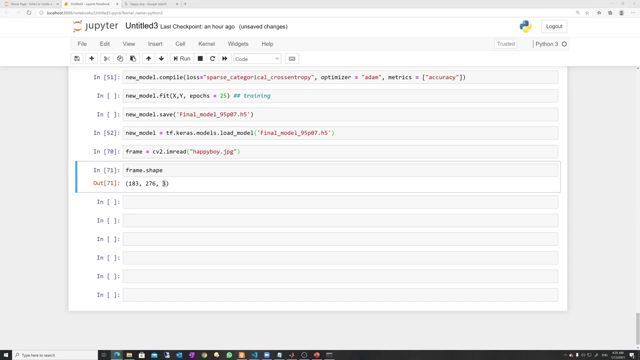 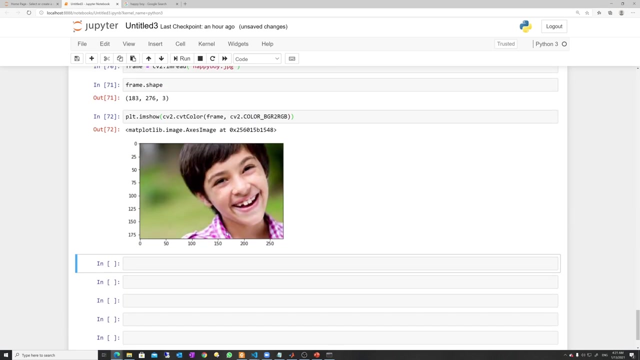 and then let me check the shape of this image. okay, this is the shape, so this is rgb image, as there are three channels, so let me show you. so this is the rgb channel. so now the best thing is that we need to crop the face right. so we want to check the accuracy on the only the face, not the background, so we need to crop, so we 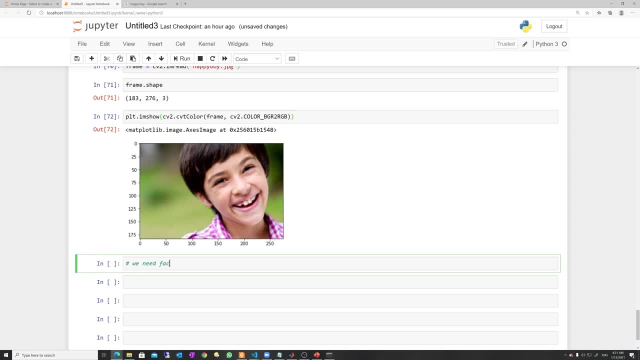 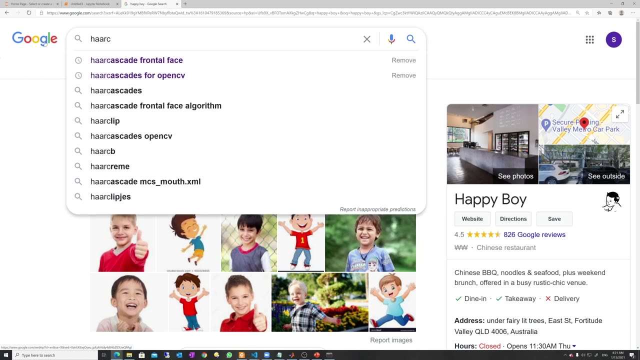 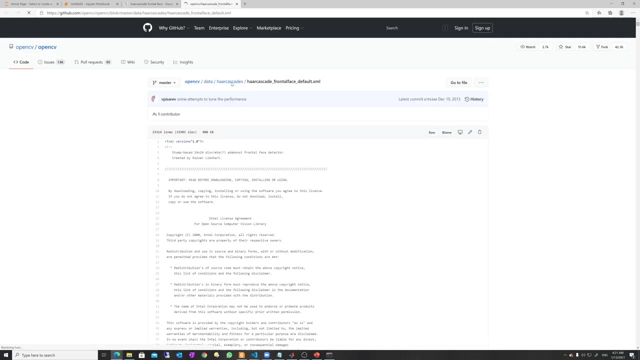 need now. we need face detection algorithm again. we do not need to reinvent the wheel, so let's write r- cascade frontal face. just write in the google and just go to the github link. you will find this. this is the one. this is the file we need. it has. 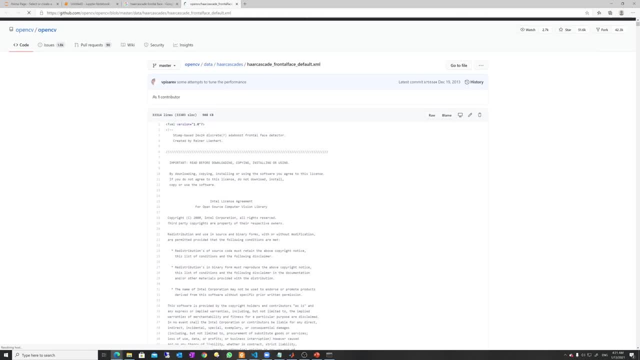 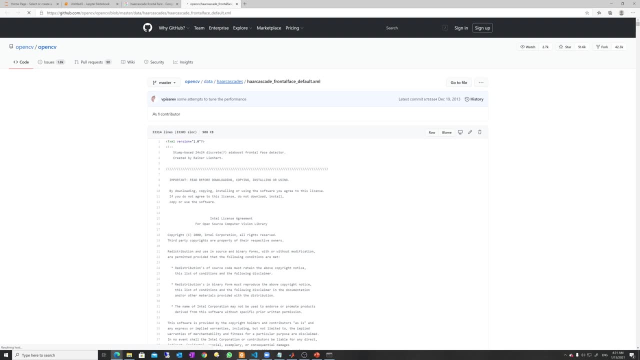 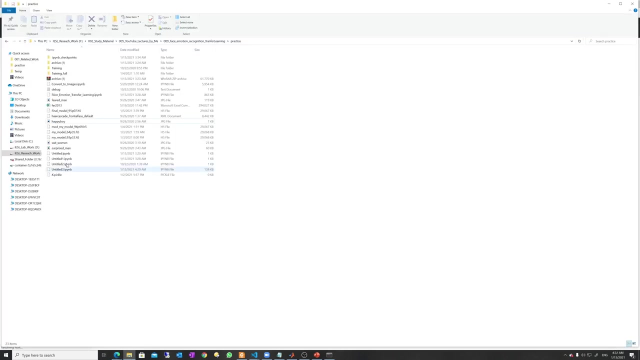 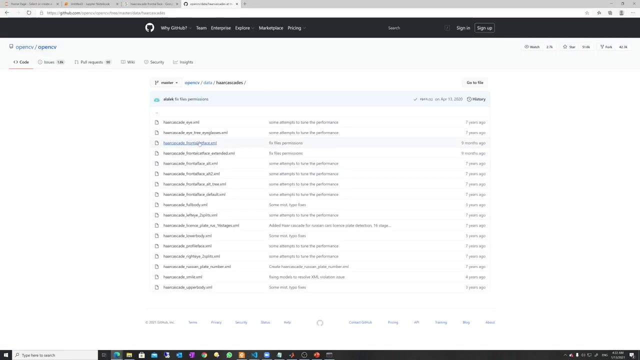 already trained weights for the face detection. if we go back, let me show you others. okay, so you need to download this file. so i don't know why it's taking time. okay, actually i have already downloaded like this one: hard caskets- frontal faces- xml file. let me show you here. so this is the one. this is the one, okay, so all you need is to just download. 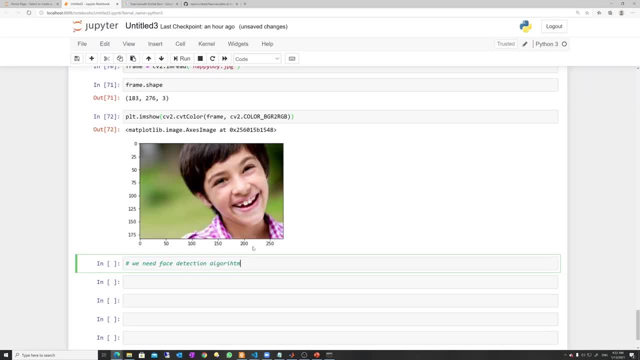 this one: hard cascade frontal default. this is face detection algorithm. so basically it works on the gray images, not three channel, right? not rgb. need is to just convert uh, my images into gray, but first i need to run this command, okay, so this one is this one i'm writing over here is for latest opencv, right, if you're using older version, you. 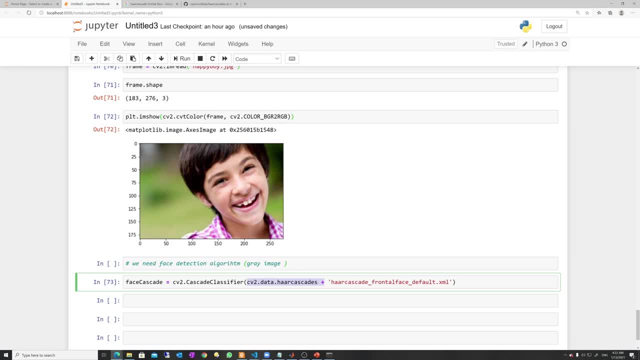 don't need this, but in case you're using opencv latest version, i believe you will install, so then you need this one. so now that i have, i need to convert into the gray image. actually, let me convert into gray image. okay, let me check the shape of the gray image. you see that there is no. 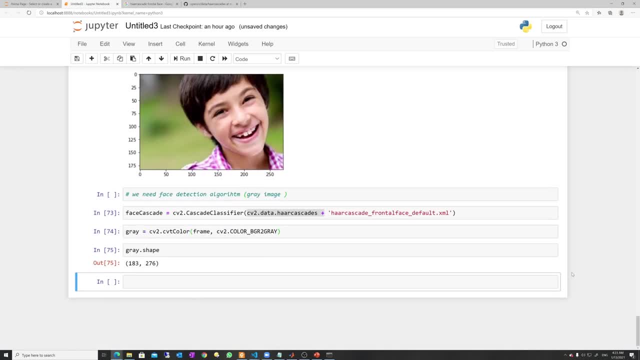 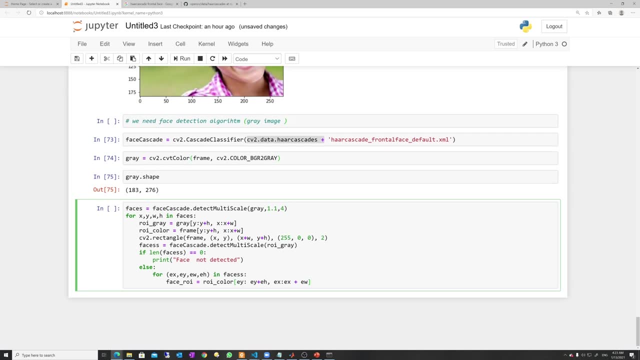 three. now three is gone. okay, because now it has been converted into gray image. so let me write a code such as: face is equal to face, cascade dot detect multiple. this is the opencv code. okay, you can just use it and you can just copy. uh, the this. you can just pause the video and just copy the code and once. 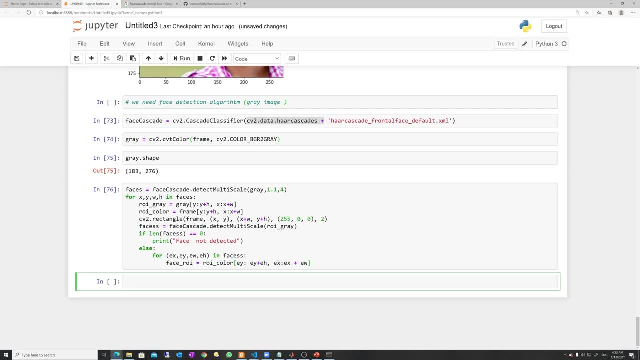 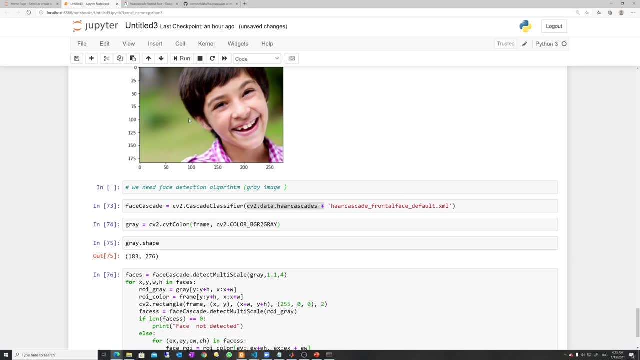 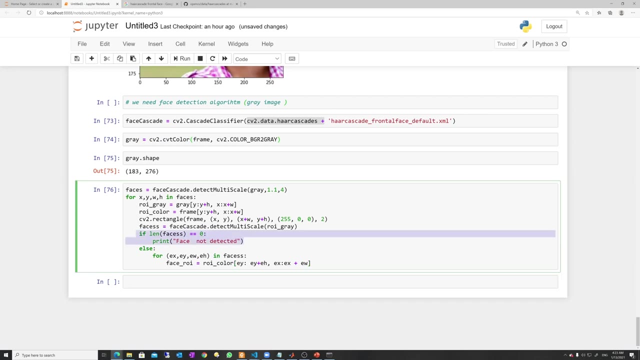 you. it is actually basically finding all possible images, uh, all possible faces inside the image. so if you have multiple faces, it will detect all of all of them, right? so if it do not contain any face, It will just throw an error that I could not find. any case, You can just change the code. 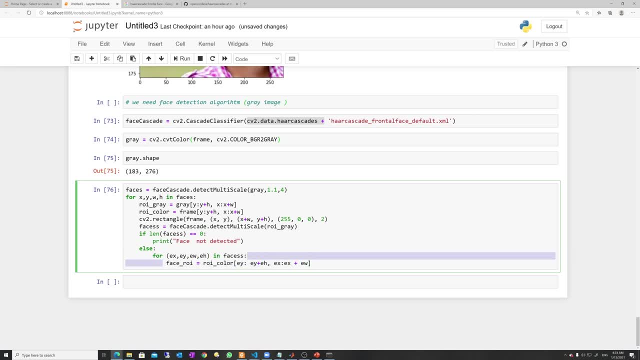 Okay, and now we are having some region of interest, So I have defined some boundary, Okay, so I'm just Defining, I'm having a rectangle across the Boundary of the face right now that we have detected the face. Okay, so let me a lot. 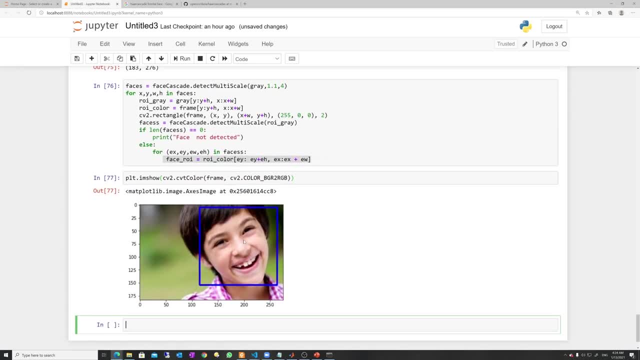 You see, over here it is with a rectangle. why this color is blue? because I Have just said that this is BGR. actually, These are actually BGR: blue, green, red. So blue is one. that is why it is blue. if I just change it to Red, it will be red, right. 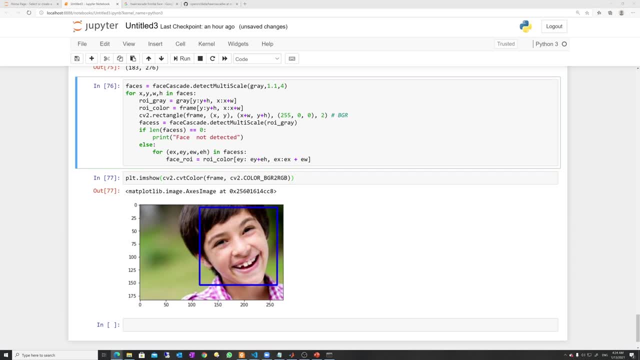 So any of the image, you can just do it. Let me crop, so as in this Particular, I have just plotted the frame, But in this particular I have already cropped the image. Let me plot this. So this is converted right. so now we have only happy face. 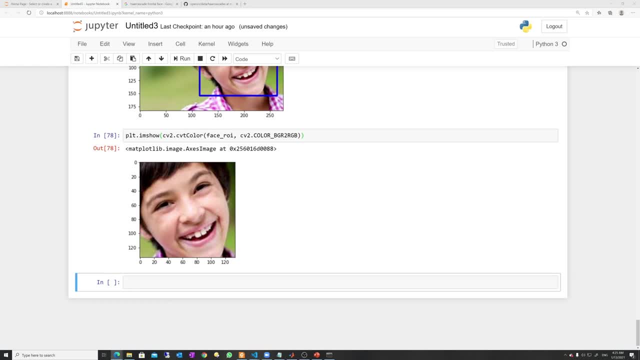 Okay, So let me change the size. Okay, or let me, As, as you know that this one is, this is one is not is an RGB and we need to convert into: Definitely we need RGB, right? So all I need is to Just do it like this, sorry, 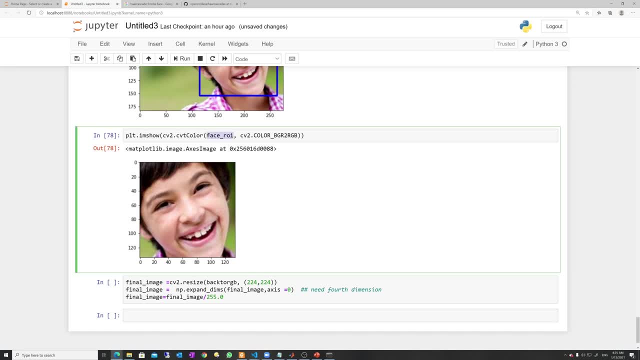 Sorry for some terrible Mistakes. as it is live. Okay, so now face ROI is RGB. actually I was trying some back to RGB and different things to you. I was working to get some good, accurate results for you guys. So what I'm doing over here is just again converting two to four. 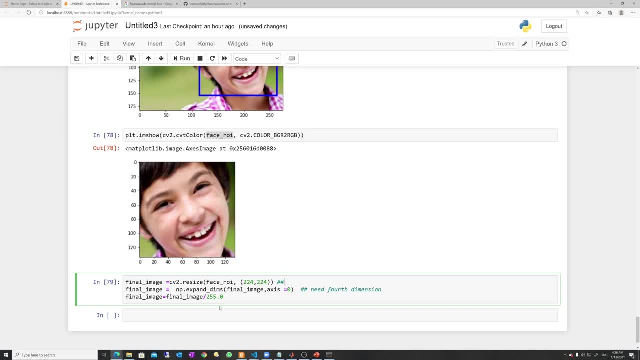 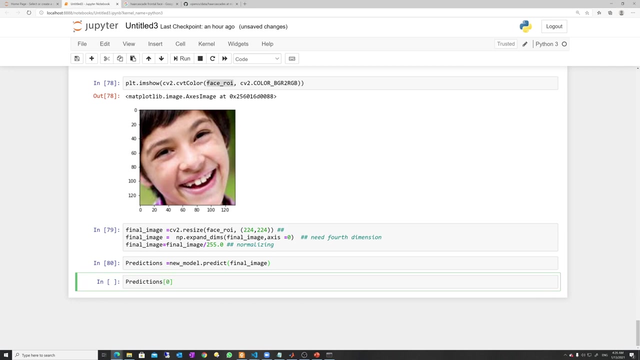 Resizing and just adding one fourth dimension. as I told you before, it needs four dimension, and now they over here. You're just normalizing it, Right. so we are normalizing it. now that we have normalized everything, let's predict, Okay. Okay, now that I have a prediction, Let me show you the predictions. What are the predictions? So these are my prediction. 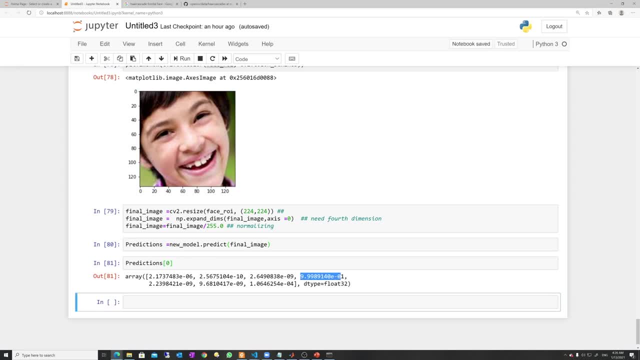 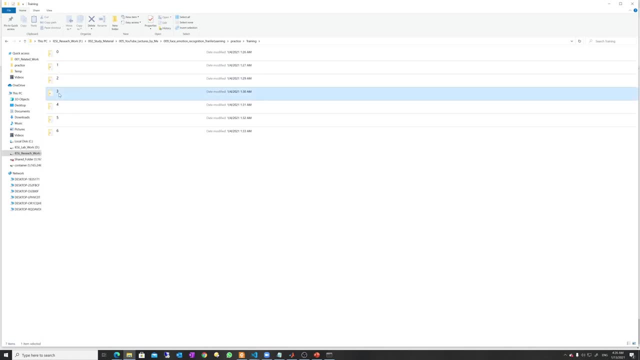 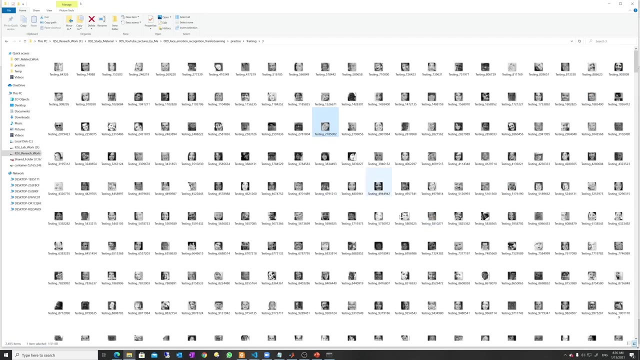 This is zero. This is one, two and three. you see, three is the Minimum one. can we check What was our three? You see, all of them are happy faces, Okay, and I'm telling you that this happy boy is not inside these images. All of them are happy faces, okay, And I'm telling you that this happy boy is not inside these images. all of them are happy faces. 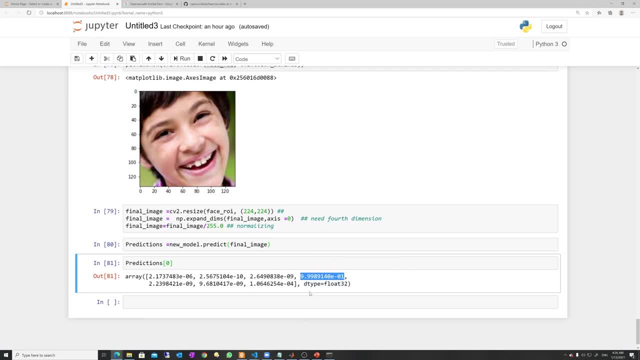 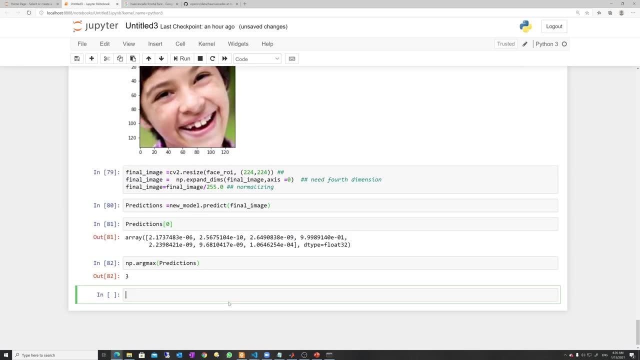 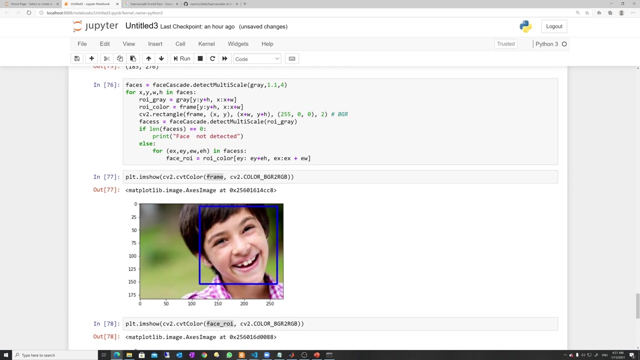 All of them are happy faces. So it has categorized is at three. but I didn't get What I'm, so let me check. Convert the the min, the maximum of it. So it is three, so maximum is three. three shows it is happy, Right. so now, when it says three it means it is happy. and then then, now we have written the code. 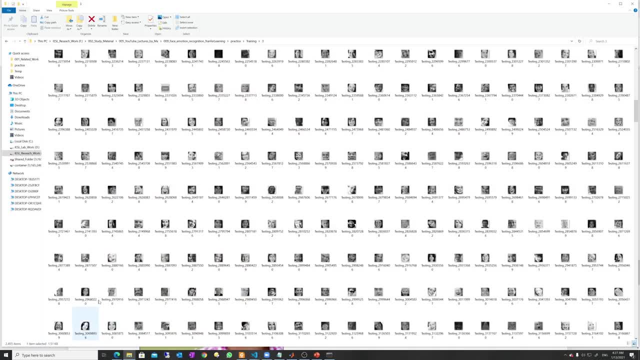 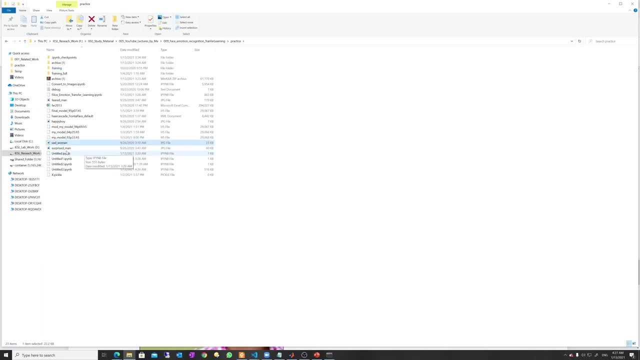 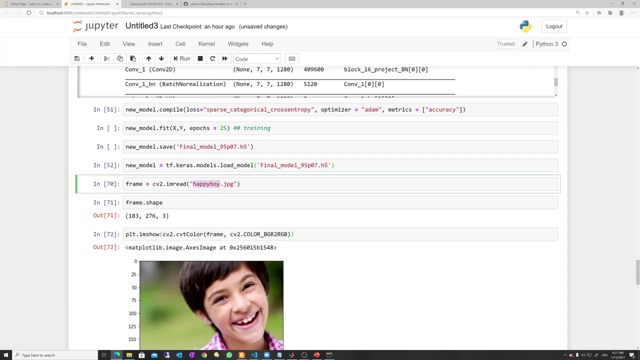 Let me do it again for everything, but this time Let me check for another image. Oh, Let me check, Maybe for surprise man. Okay, then again, I have downloaded it. Please assume that I have download. you can just search surprise man. Okay, let me do it again. again, You see, this is change. 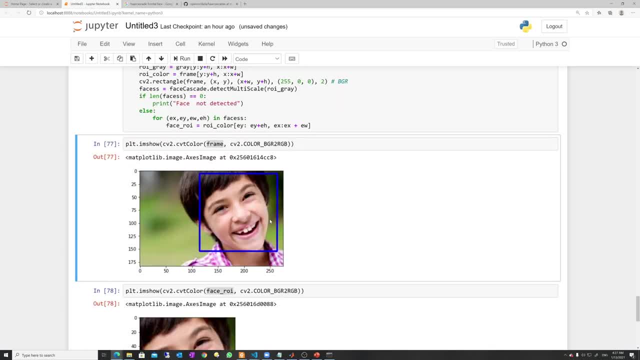 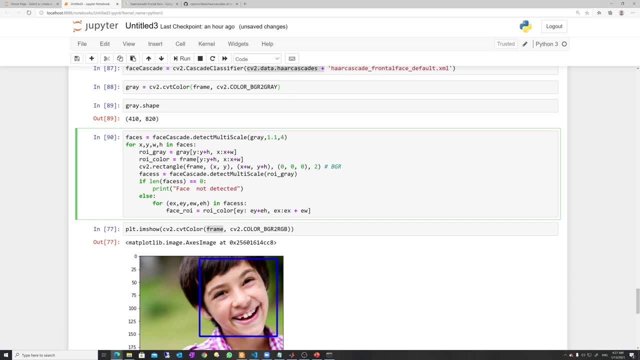 Let me execute all my lines again and again. Oh, okay, Let me. I Let me show you that if this is two five four, And this is two five, five, BGR, Now this time it would be green. So let me do it again. 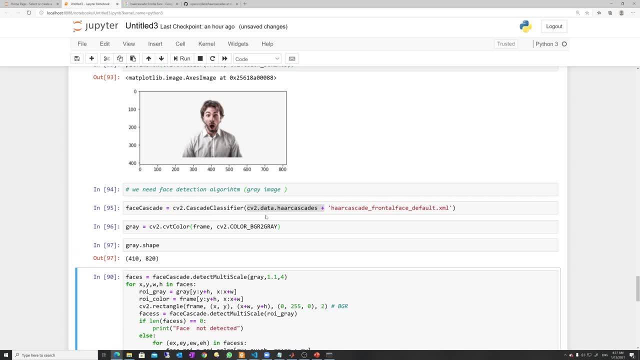 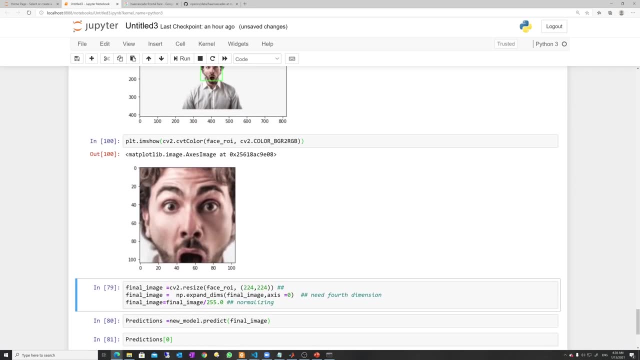 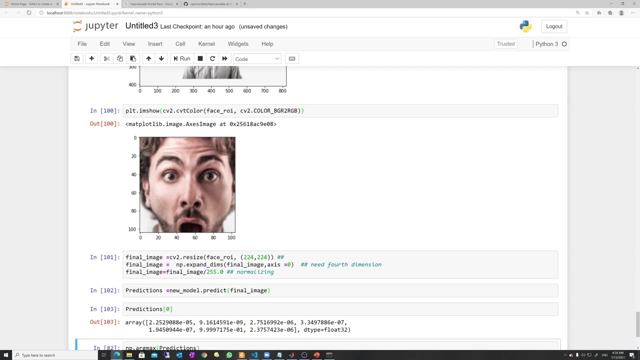 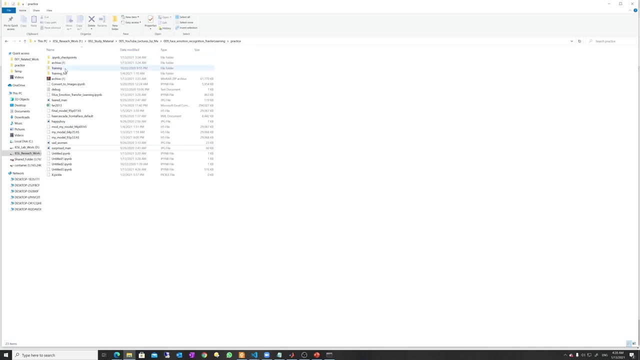 And we load again. You see, this is green this time. why- and that makes you get again shift enter is the shortest. come on, let's Resize it and just predict. and now The prediction is which one? let me check my predictions: It is five. So if I go to my training and I've had checked five, 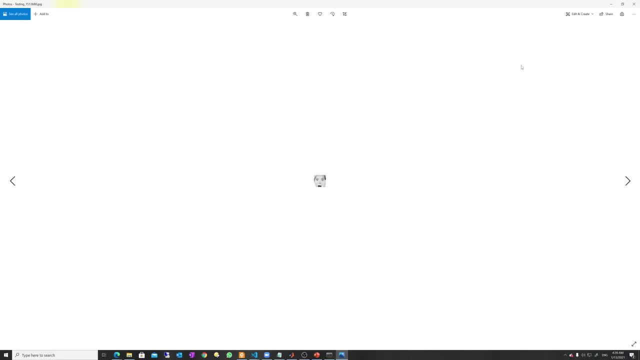 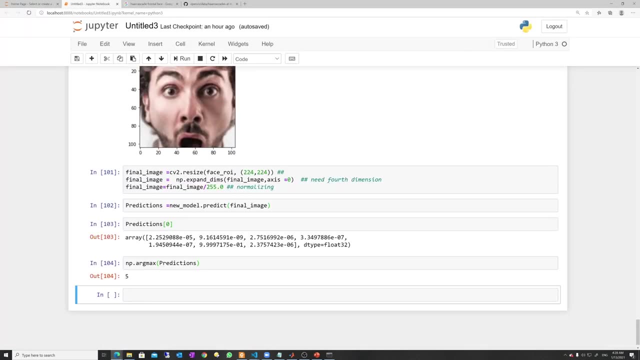 Five is definitely surprised, right? So all of these are from surprise. Yeah, Yeah. So now I have found that my deep learning architecture is going. well, Let's go for the live demo. Well, this is the code for the real-time video demo. 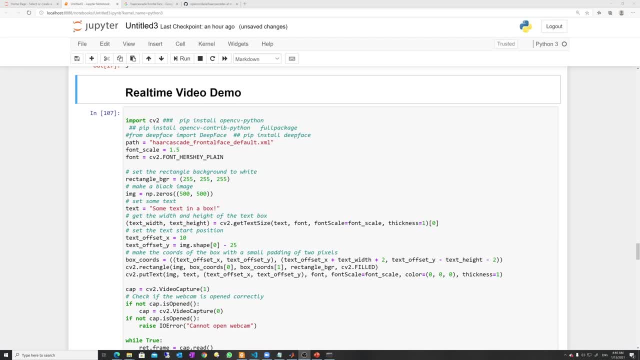 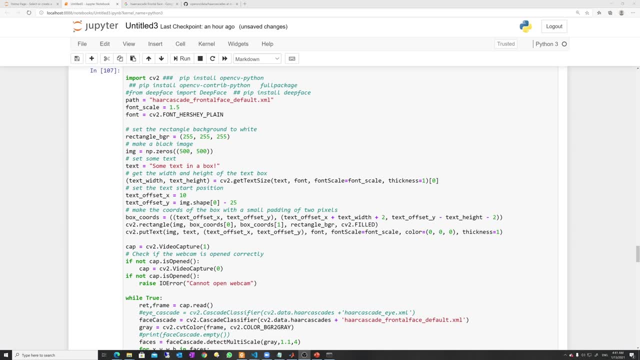 Import cv2. we already did, but I'm just doing it again And this is the path. previously We just down, although we already did hardcover interface. but I'm just providing the path and these are the foreign scale. you can just define and you your phone style, you can just define and 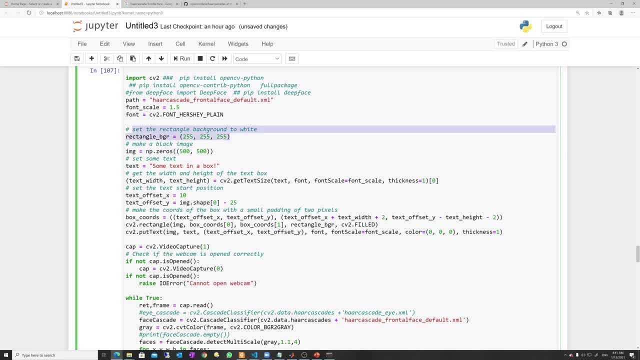 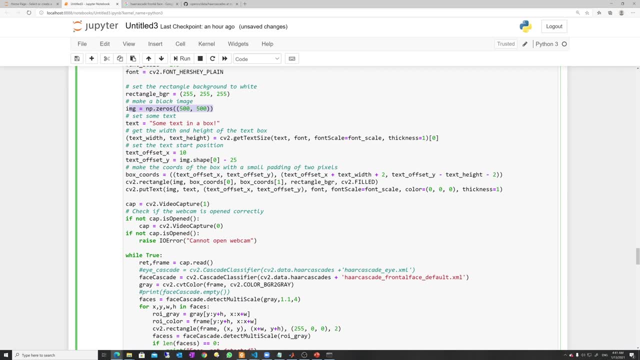 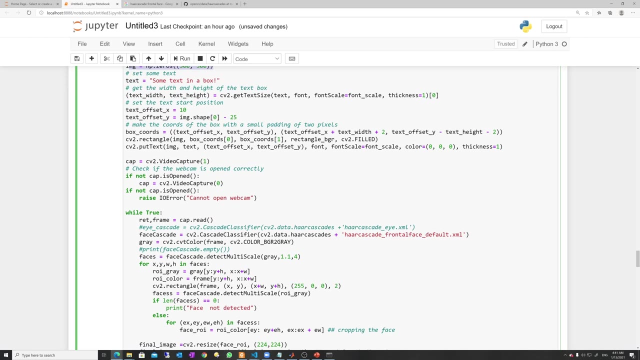 Over here. I'm just setting some background, a black background- You will see shortly in the webcam demo- and I'm just putting everything zeros, okay so, Okay. so I'm just putting some text and then I'm just getting this size and these are some offsets. i'm just, i have just defined and okay. so actual code is starts. 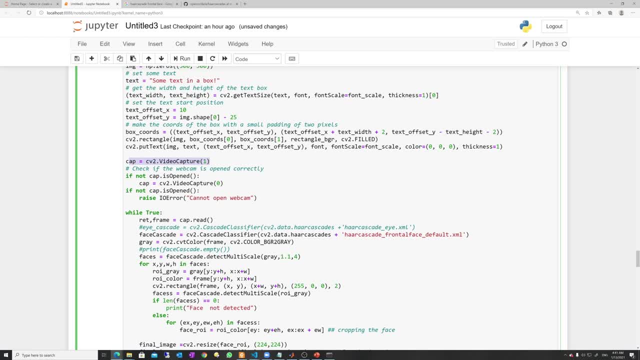 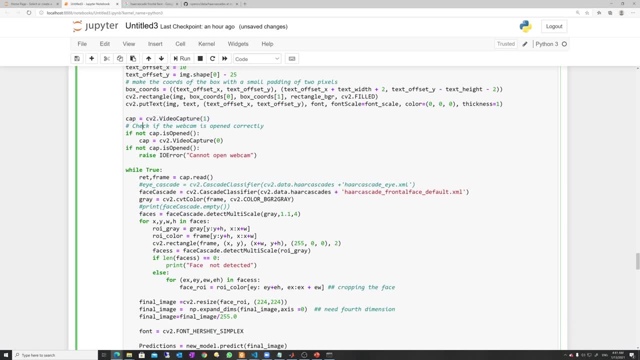 from here. all the previous code is just to show you the black rectangle to plot something i will just explain shortly. so, based on your webcam, which webcam you are using actually? so you can just have zero or one, but it is. it is actually a dynamic code. if you write this code, your camera will. 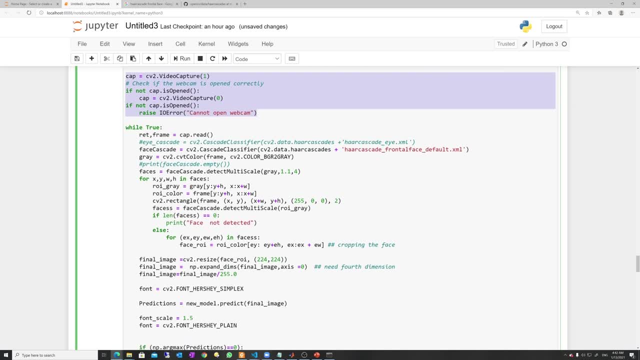 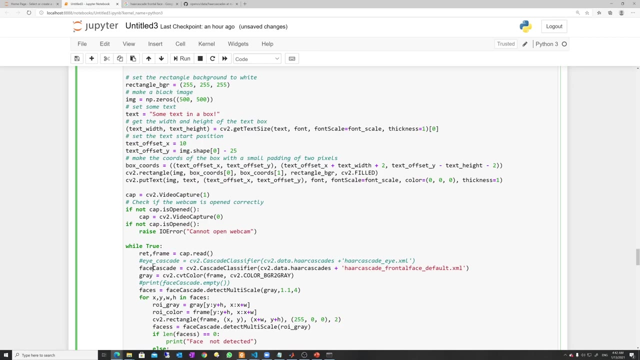 switch on. once your camera is switched on, we will be getting this cap and cap dot. read. this video will read frame by frame and it's for infinite while loop and then phase cascade, and that that this is a go like this. so okay, you don't need this path, but i have just over here, if you. 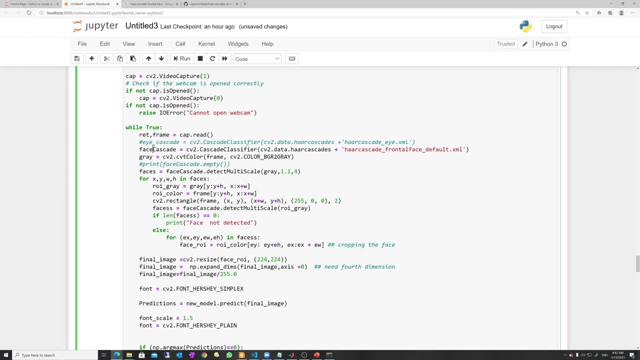 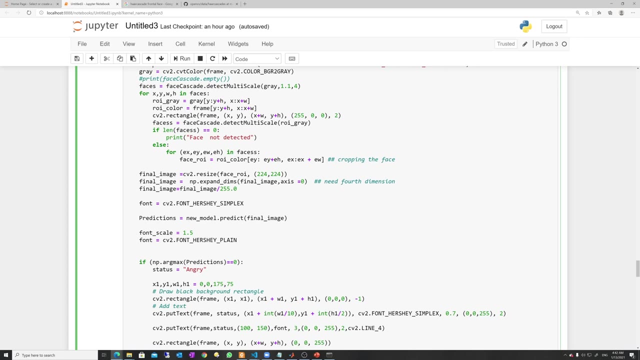 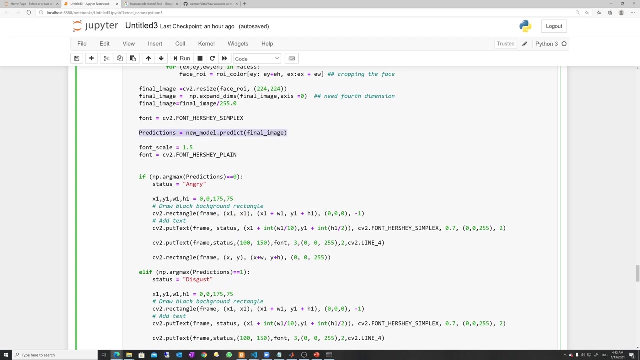 can just write the path over here as well, and then gray is equal to. i'm just converting into gray and then checking all possible faces inside the corresponding frame and then i'm just doing cv2.resize and then npexpand and then all of them now once i get the prediction right. so if my prediction nporg max, as we did- 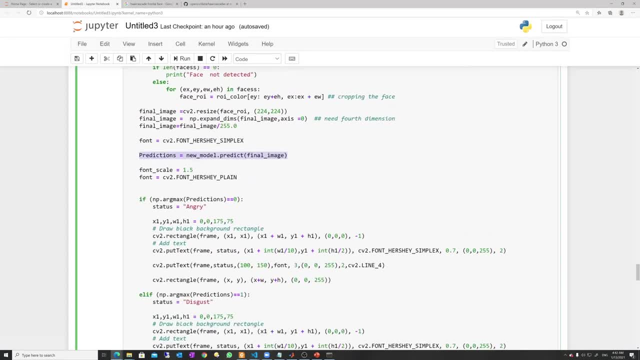 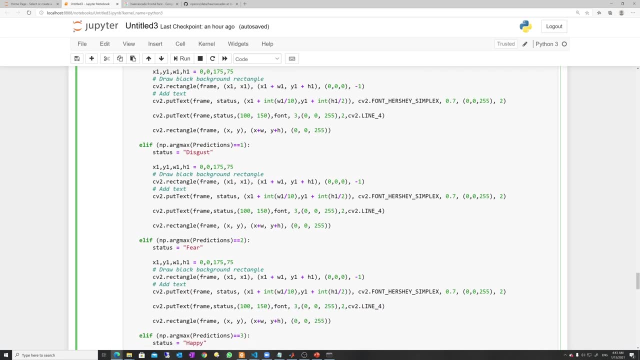 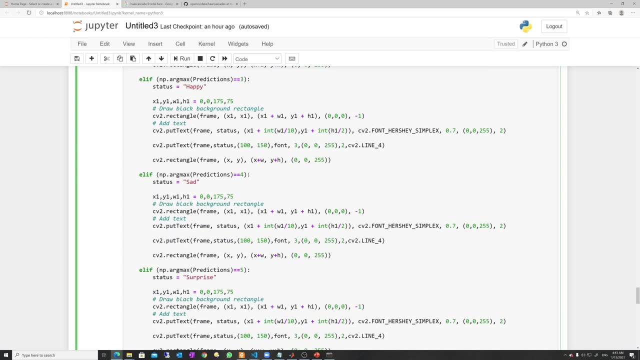 before, like it was five for surprise, so for example, it could be any right. so zero says it is angry, and if it is one it shows disgust, and if it is two it shows fear, three it shows happy, four shows sad and five surprise, as we did before, and else anything else. 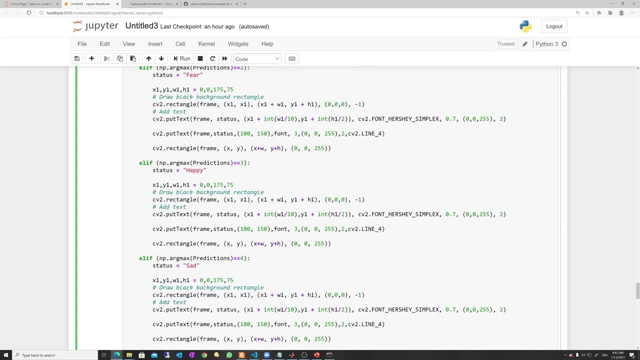 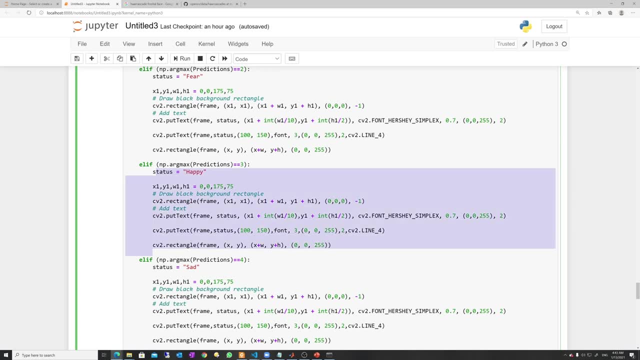 is neutral. so this is the code, what i'm doing, and just this is all of them are just copied, copied paste, right, and all you need is you just write three and instead of three. you need just three to four, so you don't need to worry about it. and then you just write three and instead of three. 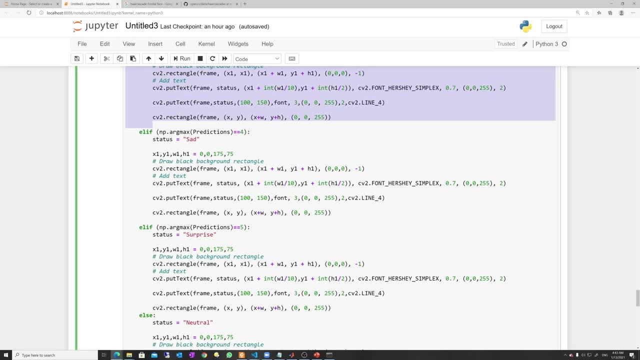 once you write this one, all you need is just repeat and it is actually put text on the frame and put rectangle right. so these are the code to have rectangle on the face and these are the put text to write the status, because if it is sad it will show the sad. so i'm doing, i'm writing sad on. 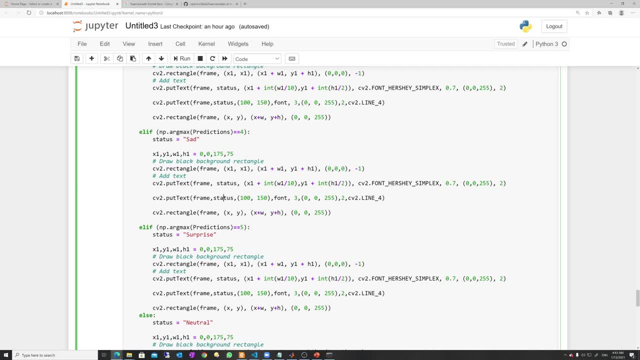 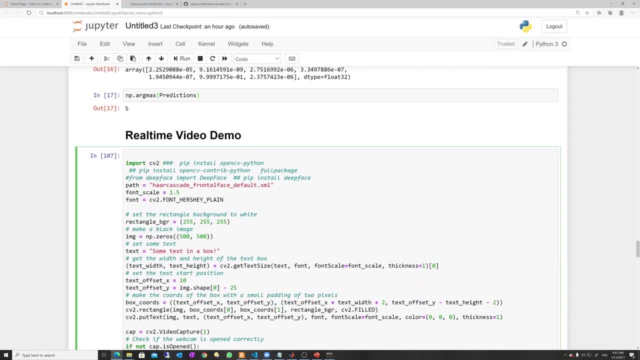 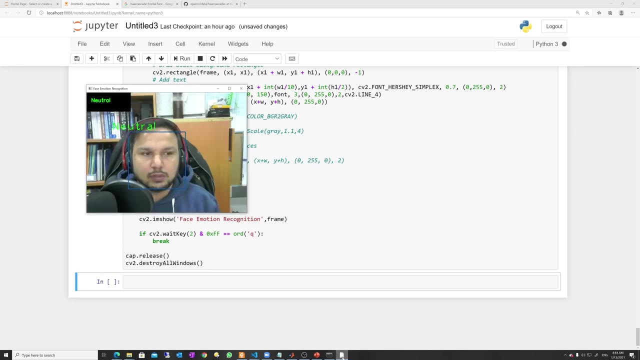 two spaces: one is near this rectangle and another is on the black rectangle. i will show you shortly. let's have, let's execute this. if i execute this, you see over here i'm neutral. now let me happy. when i show my teeth, it is having happy. so surprise, if i want to be angry. 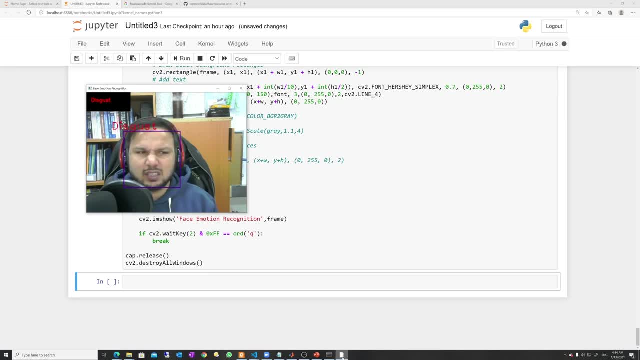 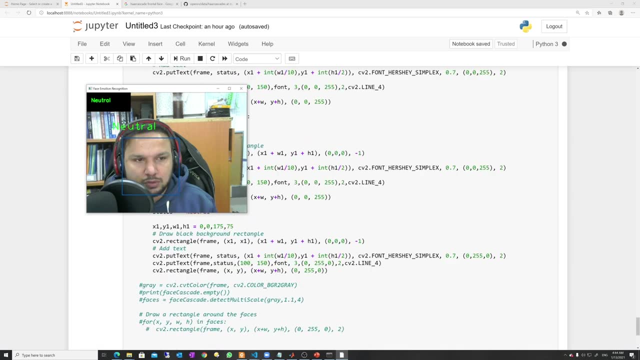 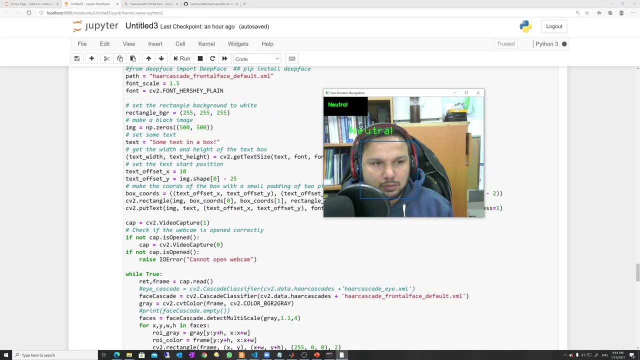 so fear and angry is like, and what discussed is like this. sorry for my terrible emotions. so you see i was discussing this. so here you see the black rectangle. so in the code, in the code, i was doing this. yeah, so this is the first part. i'm just writing the black over here, right? 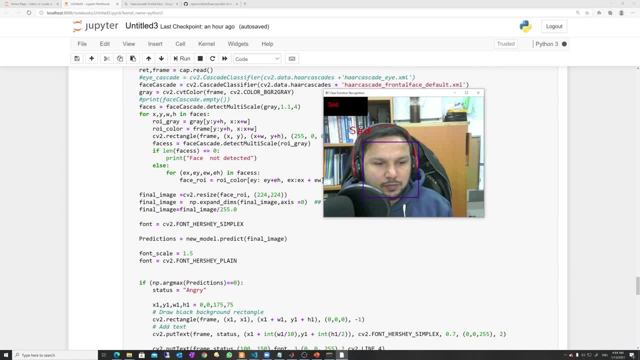 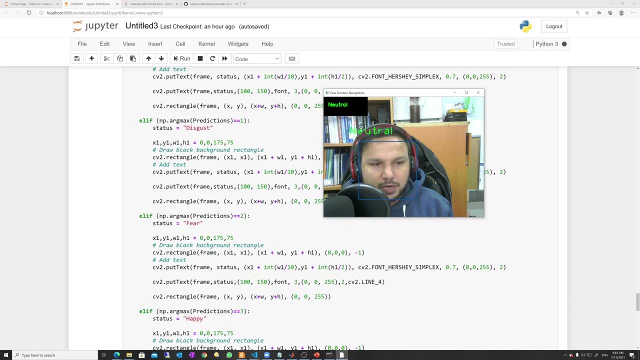 so i'm over here, i'm just writing the black and definitely for plotting the rectangle, i'm just doing it over here, right? so these are the one. so i'm rooting writing two status: one state is on the black. this is the black and one status here, you see.